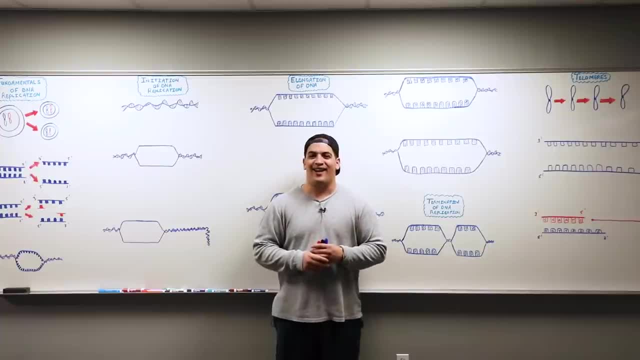 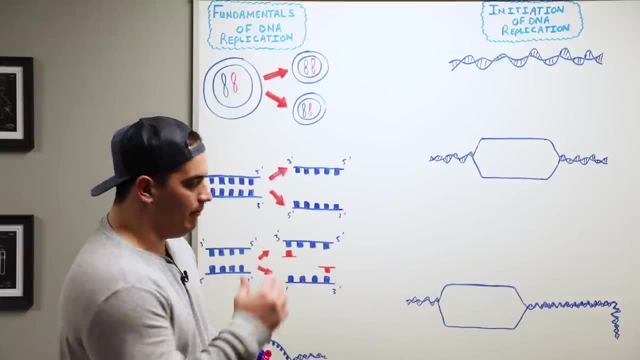 we have links to our Facebook Instagram Patreon account. Go check that out. All right, Ninja Nerds, let's get into it. All right, Ninja Nerds, when we talk about DNA replication, the first thing that we need to talk about is a couple of fundamental points, very important. 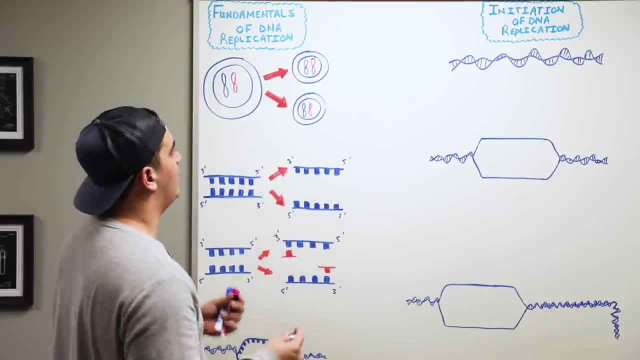 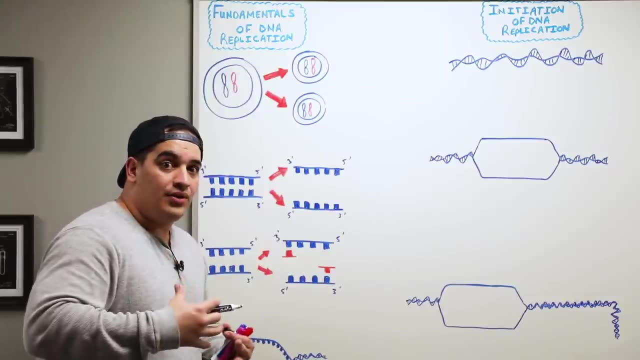 things that we're going to build on throughout the process of this lecture, And so the first thing I need you guys to know is: what in the heck do we do DNA replication for? And the whole point is that, in order for cells to be able to replicate and make more cells, we need the DNA within those. 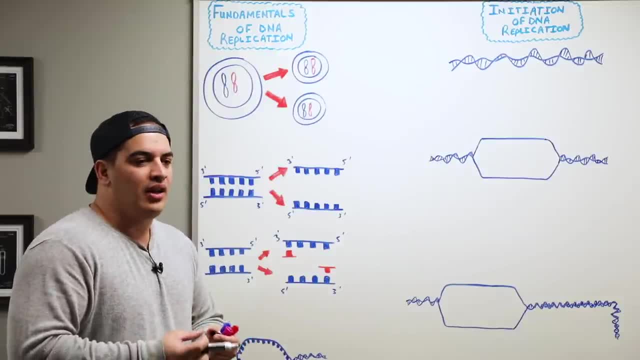 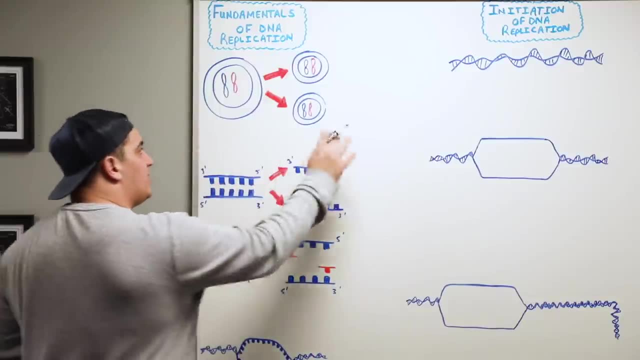 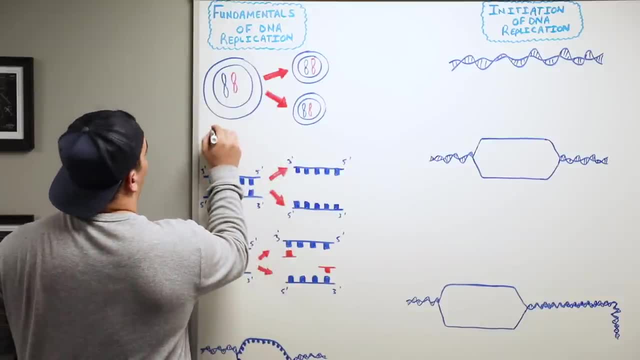 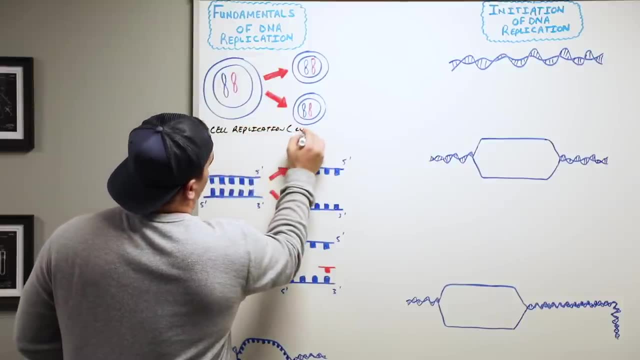 I really want you to understand that the whole purpose of it is to allow for cell replication. Okay, Or sometimes we refer to this as the cell cycle, Okay, So the cell cycle- And I know you guys know the cell cycle In the cell cycle- what's kind of the really quick part of it? 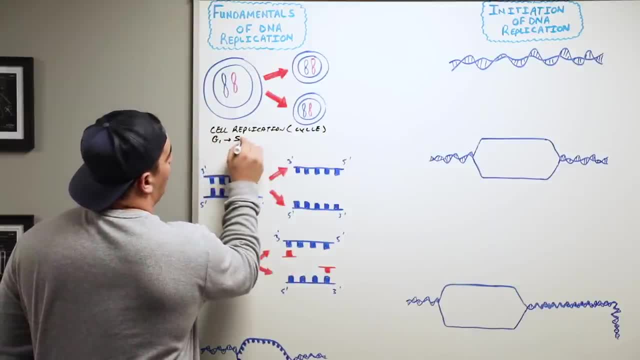 You start off, you go G1,, then you go S phase, G2 phase, and then you go into the mitosis part, And then out of that you go G1,, then you go G2, and then you go into the mitosis part. 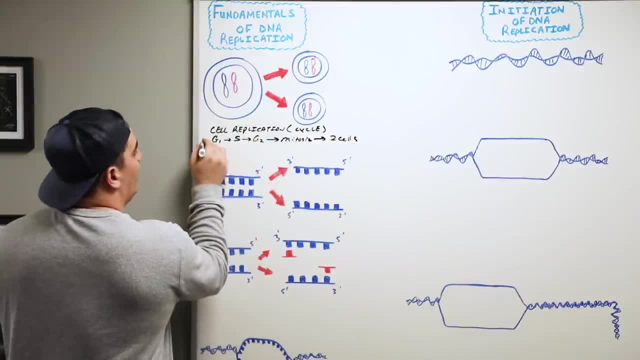 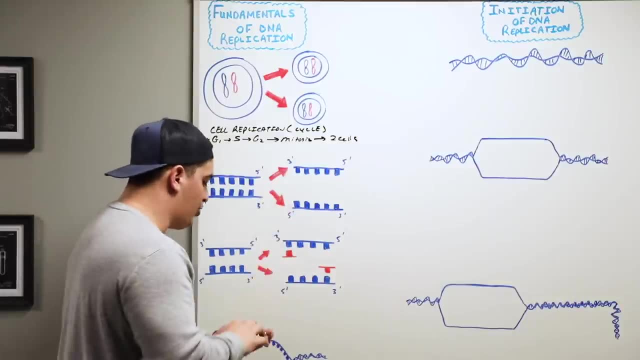 And out of that you get two cells, Where you take one cell, that cell enters into the G1, S G2, goes through mitosis and makes two cells. The big thing I want you to know is that DNA replication primarily occurs within a particular part of the cell cycle. When a cell is replicating. 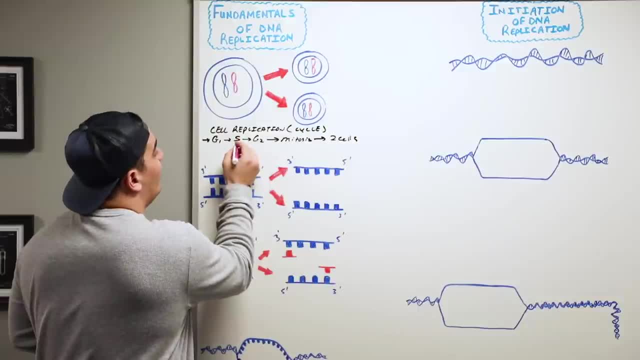 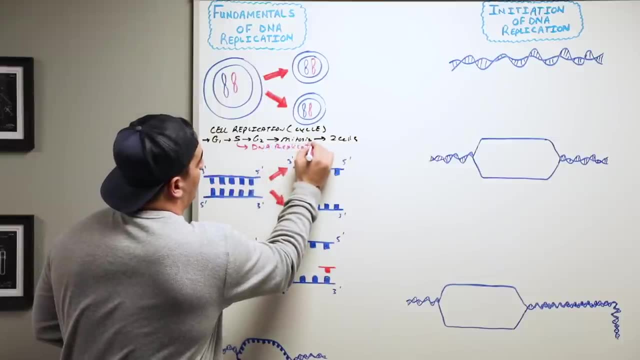 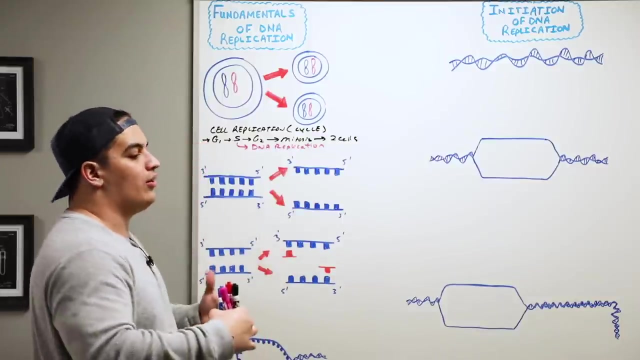 and making more cells. it primarily occurs within the S phase, So in the S phase, that is where DNA replication is occurring. So the first fundamental that you need to know is: why do we perform DNA replication? In order for our cells to replicate, make more cells. So whenever 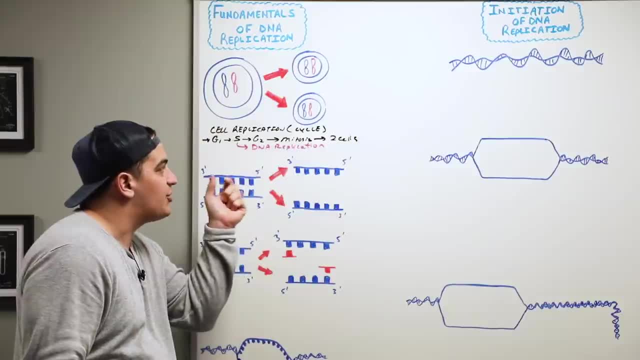 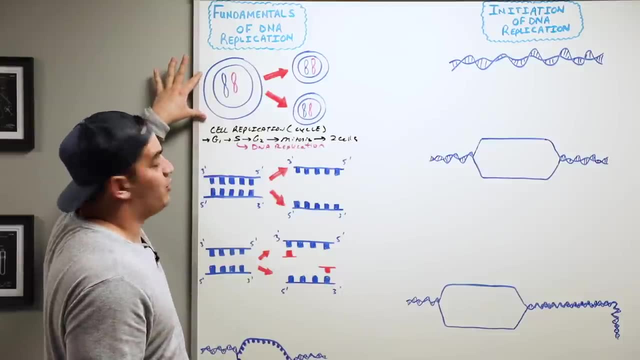 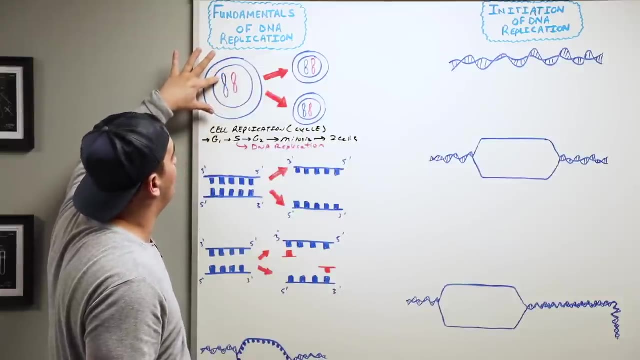 they go through their cell cycle. the particular point when the DNA is actually replicating is in the S phase of the cell cycle. Now, real quick, what in the heck is cell replication? It's really simple. I'm taking this cell here which has 23 maternal and 23 paternal chromosomes and all I'm 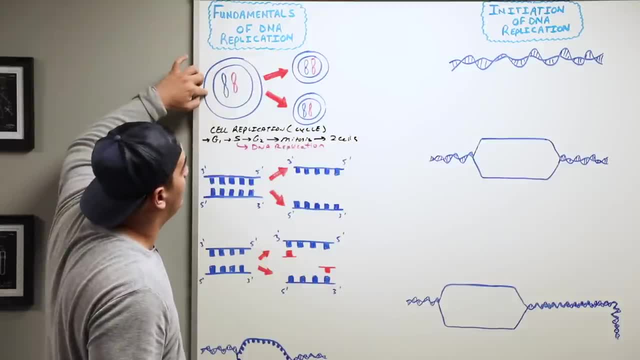 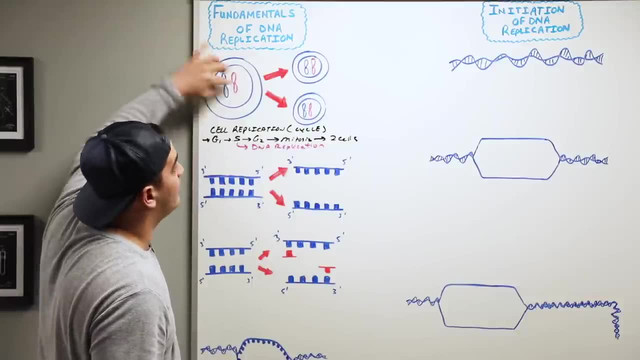 doing is I'm making two identical cells that look just like this, So I have to replicate the DNA within this chromosome and the DNA within this chromosome, and I'll make two of this and two of this, and that's going to give me these two identical daughter cells, And that's the basic. 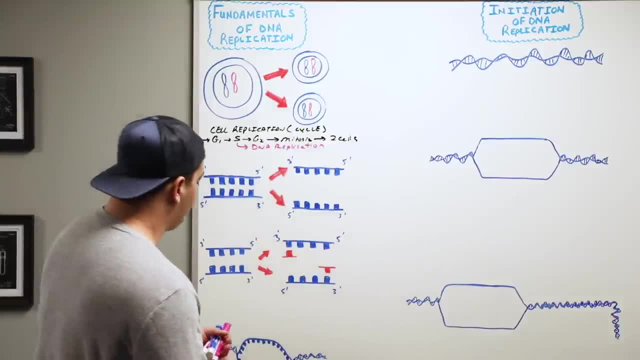 process of cell replication. So that's the first thing I need you guys to know. The second thing that I need you guys to know about DNA replication is that it occurs in what's called a semi-conservative model. What the heck does that mean? Zach, I got you, So the next thing I need you to know is that. 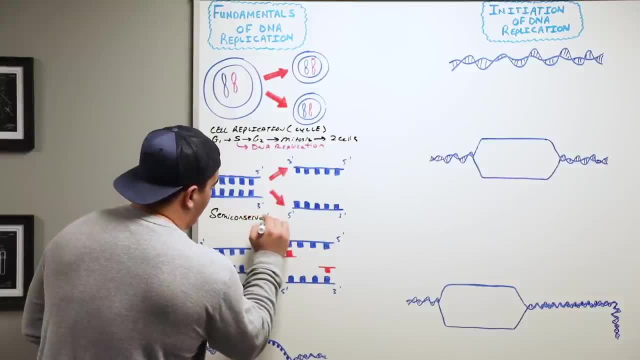 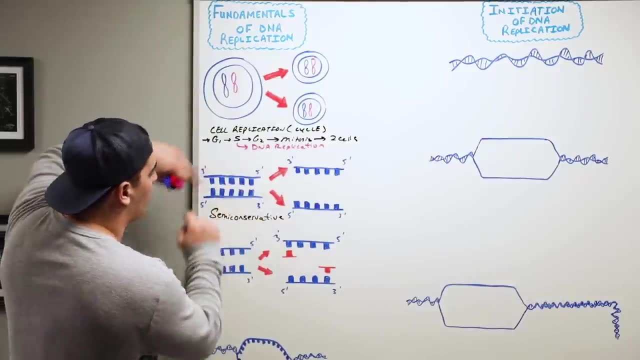 DNA replication is semi-conservative. Semi-conservative means let's take a piece of DNA here, right? So DNA has two strands and we're going to call these. we're going to give them two names. We're going to call these blue DNA strands. 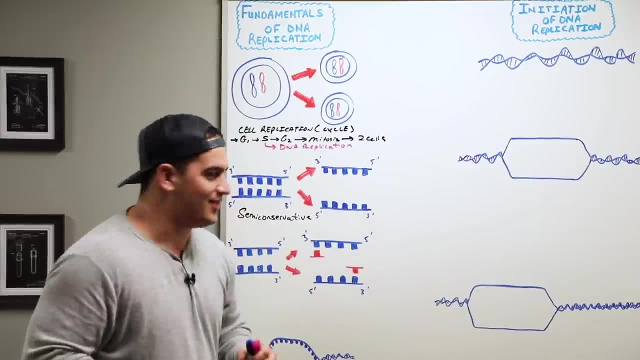 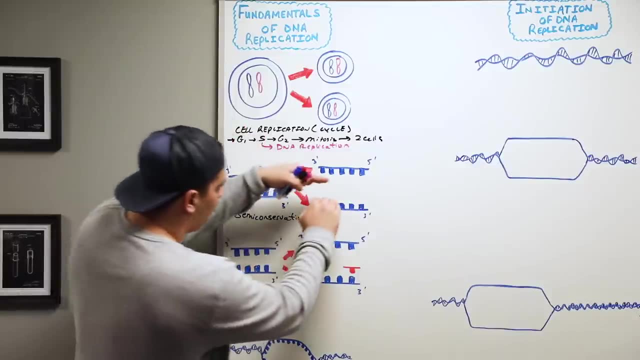 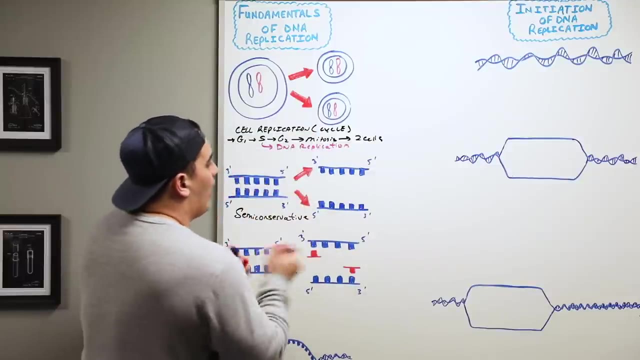 parental strands, or let's call them old strands. What I'm going to do is, when I want to replicate this DNA, I have to separate them, and we'll talk about how we do that. When you separate the DNA into separate strands. here I have two old parental strands separated. What I'm going to do is I'm 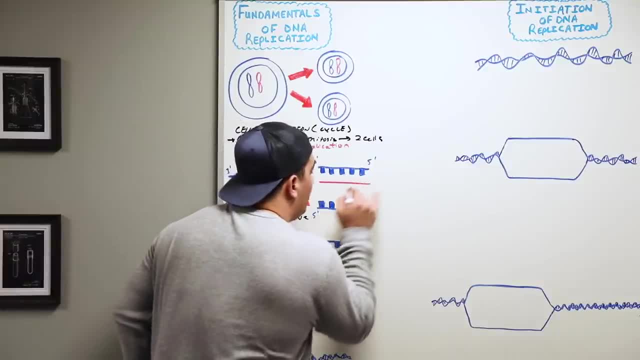 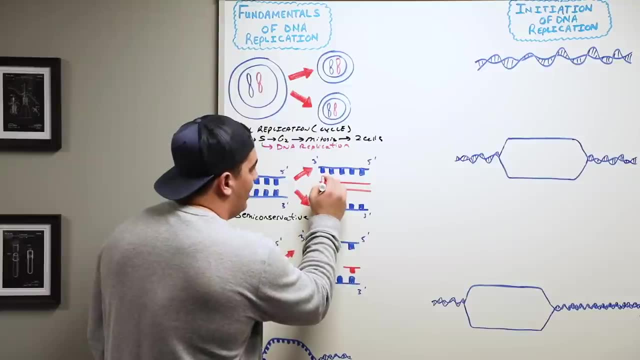 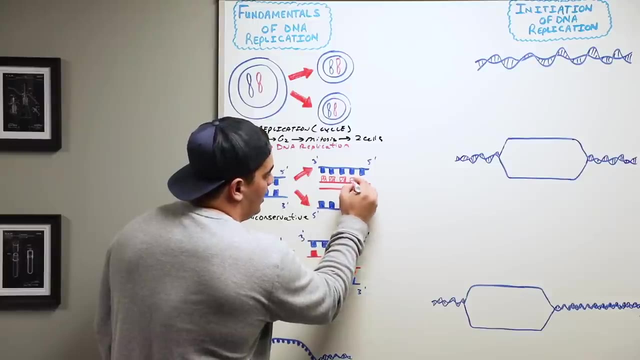 going to replicate the DNA in a complementary fashion. So what does that mean? complementary? That means if, for example, this nucleotide was Adenine or A, this would be T. If this was T, this would be A. This was G, this would be C. If this was C, this would be G. You get the point. 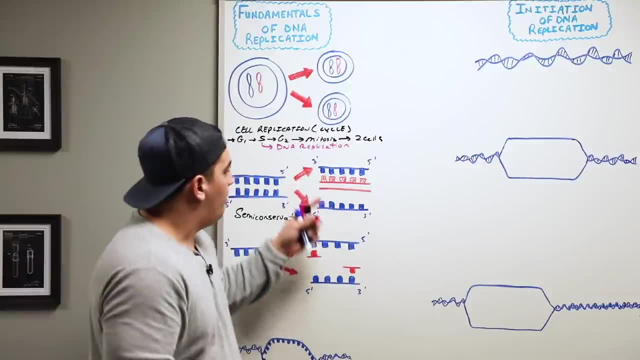 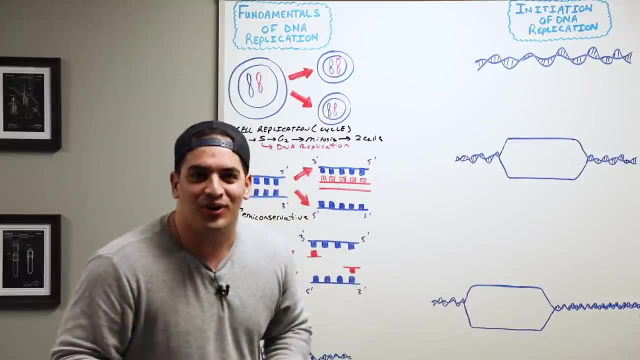 I'm going to make nucleotides that are complementary on that, But do you see how the color is different? And I synthesized a new strand- daughter strand, if you will. that's one aspect of it And I'm going to do the same thing to this. 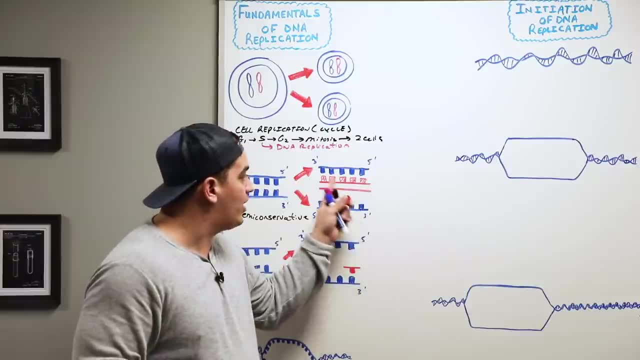 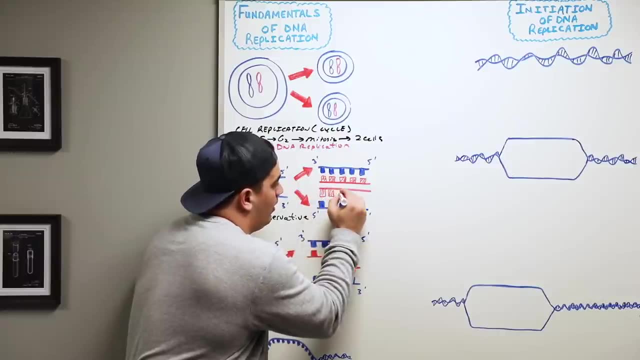 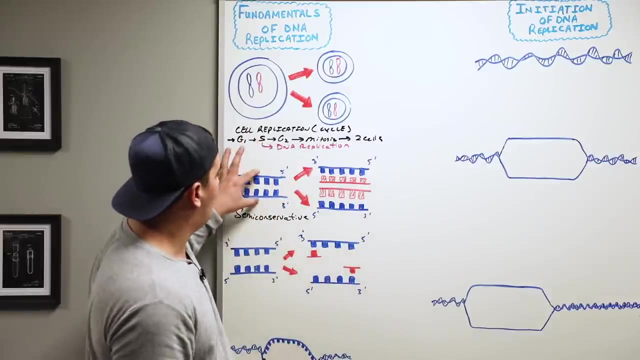 other strand. So I'm going to use this old parental strand and make a new strand with complementary nucleotides. On the other old parental strand I'm going to again make DNA that is complementary to this old or parental strand. So the whole concept here is that I start. 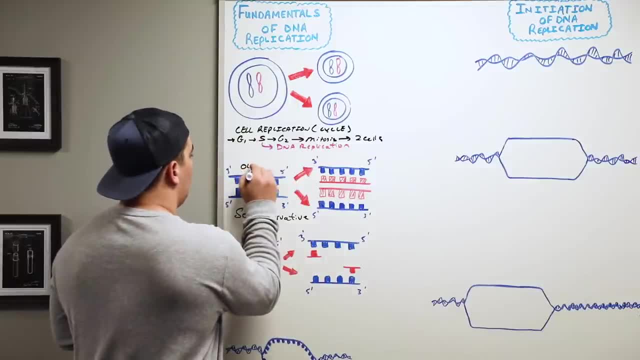 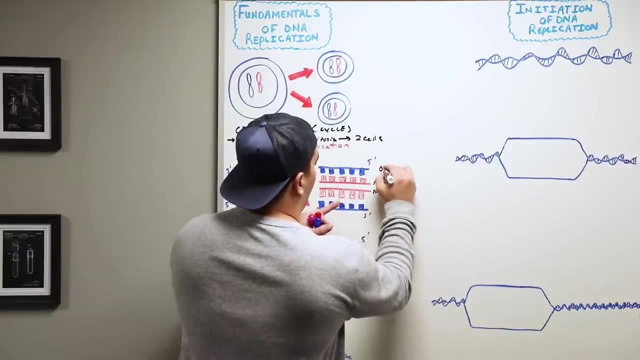 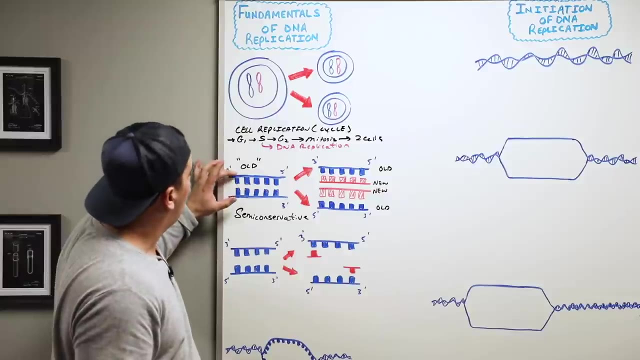 with old. if you will, let's use the term old and I make new mixed with the old. That's really the easiest way of understanding DNA replication is: I'm taking two old parental strands, separating them and making two new DNA strands that are complementary to them. 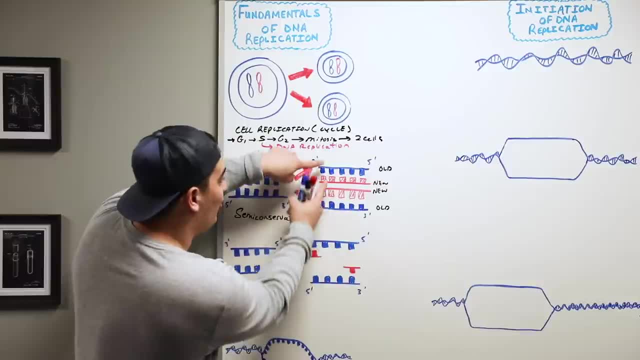 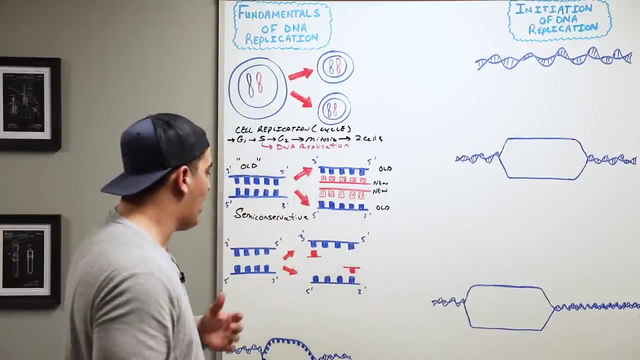 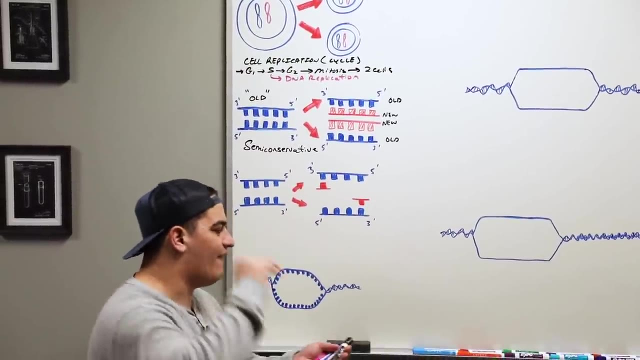 So what I did is I took this DNA and made two new double-stranded DNA molecules. Isn't that cool? And when I did it, I did it in this semi-conservative process. The next really important thing that you guys need to know is that DNA replication occurs in a very 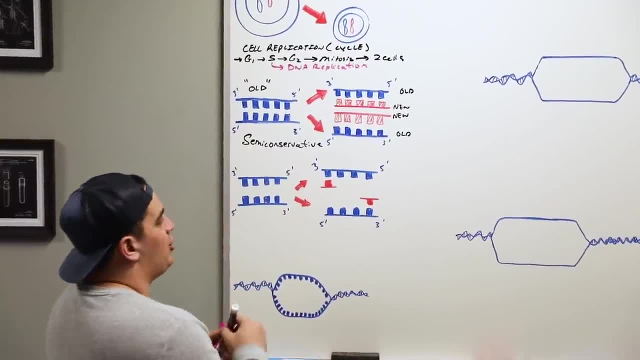 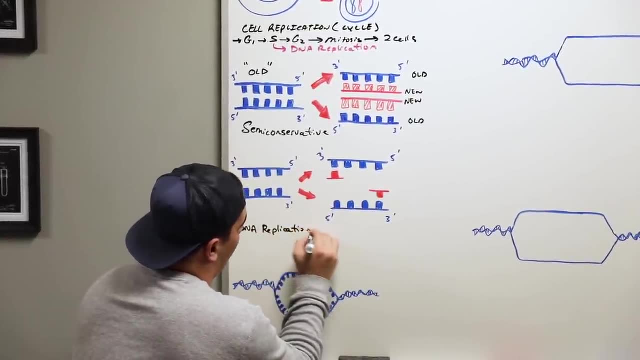 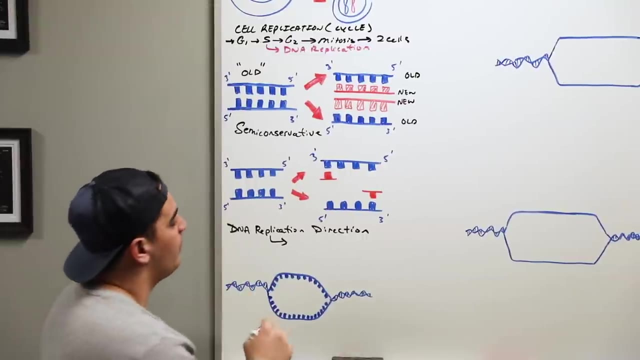 very specific direction. DNA replication has to occur. okay, the direction, okay, replication direction is very important. It's kind of annoying- We'll mention it a lot throughout the process of this lecture- But DNA direction always has to occur from the five prime end to the three prime end. I can't. 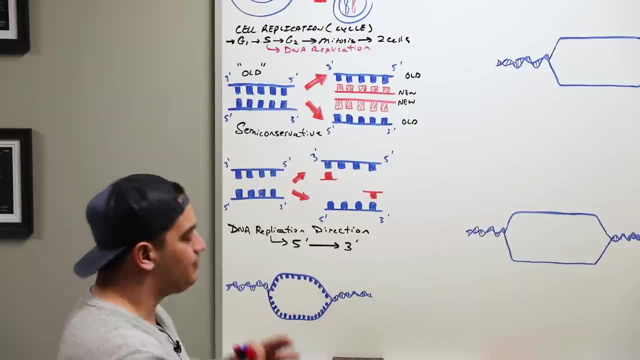 stress that enough, Super important. It's going to come up a lot. What the heck does that mean Really quickly? Do you guys remember from the DNA structure video What was on the five prime end of a nucleotide, The phosphate group? What was on the three prime end of the nucleotide, The OH? 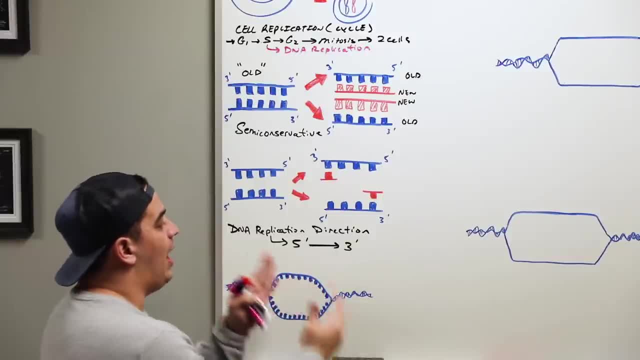 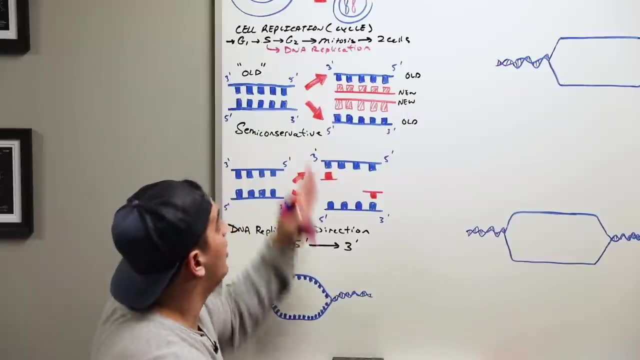 group. So when I'm adding nucleotides, I'm adding a phosphate group onto a three prime group of the preceding nucleotide. Let's show you an example of that. So let's say that we took this old DNA strand, We're going to do replication following the semi-conservative model. Here I 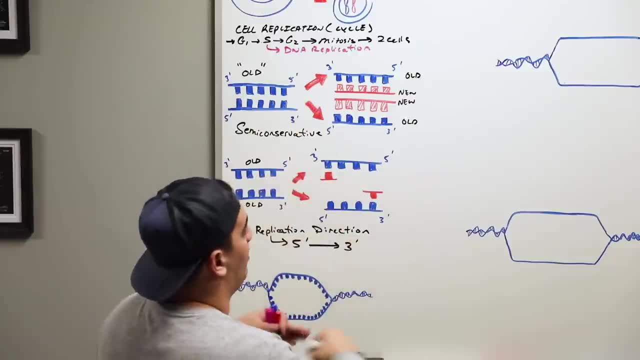 have two old parental DNA strands, Separate them. I'm going to replicate it via the semi-conservative model, But I'm also going to follow this process where I have to replicate five to three. So let's say, on one end of this old DNA strand I have a three prime end here. What does that mean That? 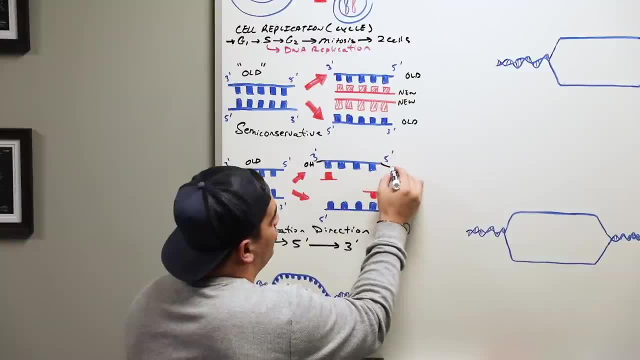 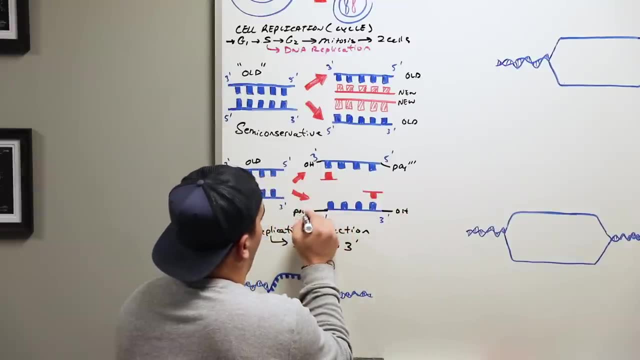 means there's an OH group here. On the five prime end of this DNA strand, I have a three prime end, I have a phosphate group here- Okay, Same thing here- OH group and then the phosphate group right here. So that's basically what the five prime, three prime end is, And you guys remember that. 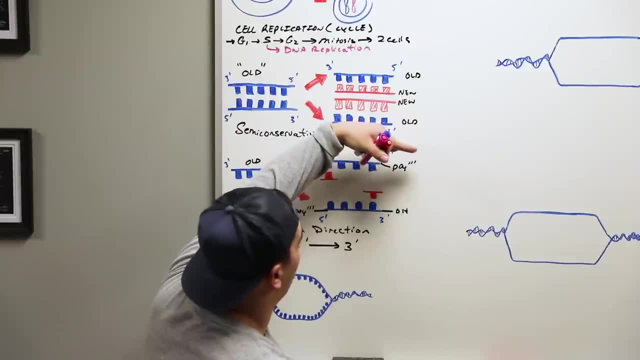 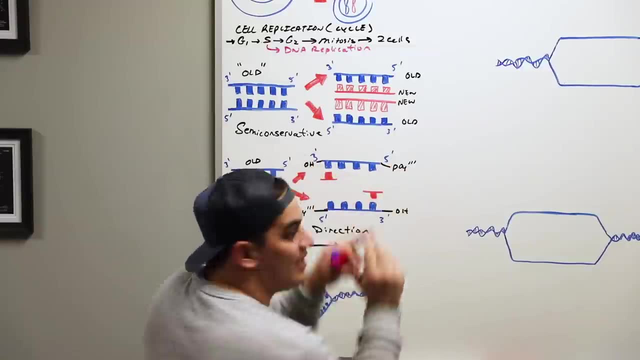 DNA is anti-parallel. So if it's three prime on one end, five prime on the other end, the other DNA strand has to be flipped. So it's five prime on the same end that it's three prime and three prime on the same end that it was five prime. That's important. So when DNA replication occurs, 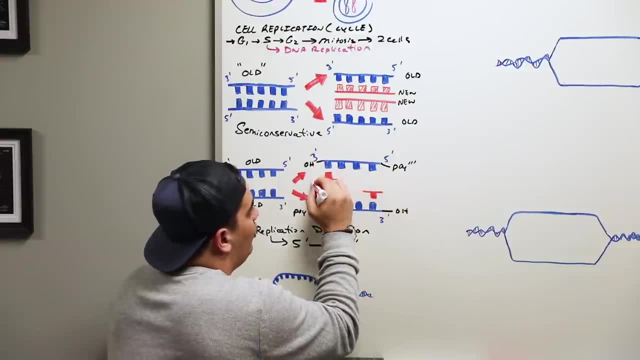 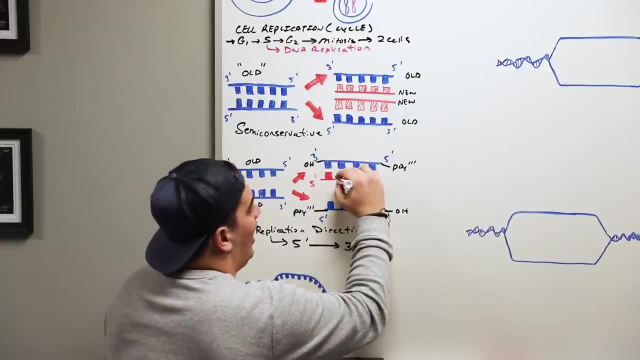 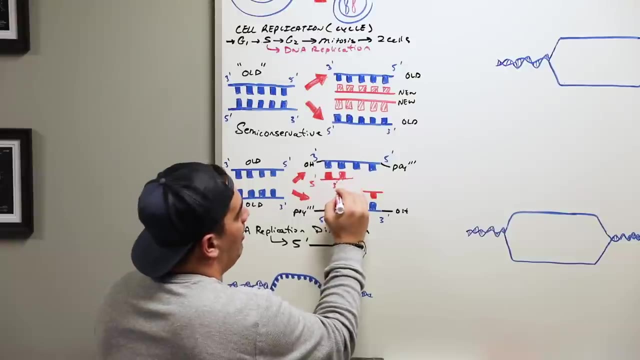 it's five to three. So here's the three prime end. When I make a new DNA strand, it has to be five prime first, three prime end here. And then what will I do? I'll add another nucleotide And then this connection here will be between what I'll have- a three prime end here, and a 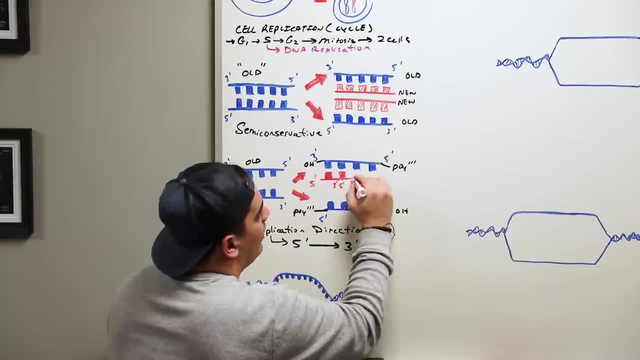 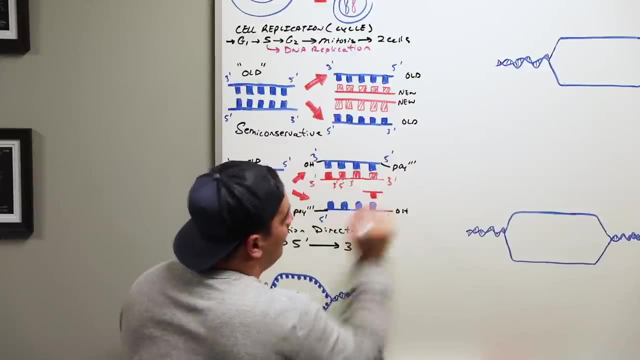 five prime end of this next nucleotide. I'll have a three prime end here. I'm going to add another nucleotide. So when I make nucleotides I make them and synthesize them from five to three. Same thing, If I'm going to do it off of this strand. here's the five end. Here's the. 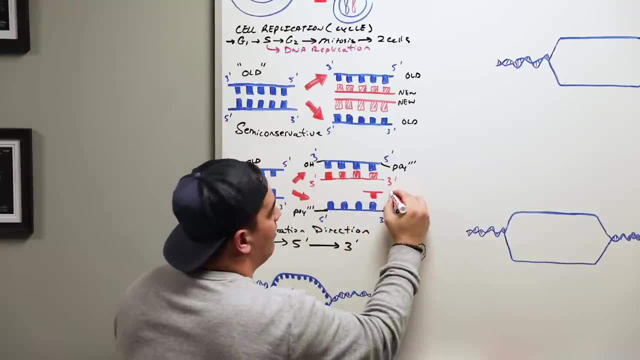 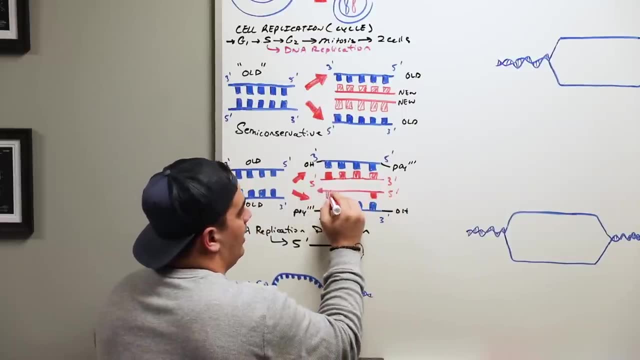 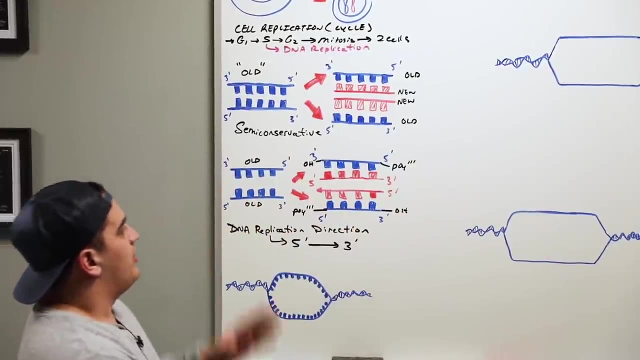 three end of the parental strand. If I want to make the new strand, this is the five prime end. So I'm going to be synthesizing DNA in which direction? In this direction, here And again, doing this according to the complementarity rule. So that's the important thing I need you guys to 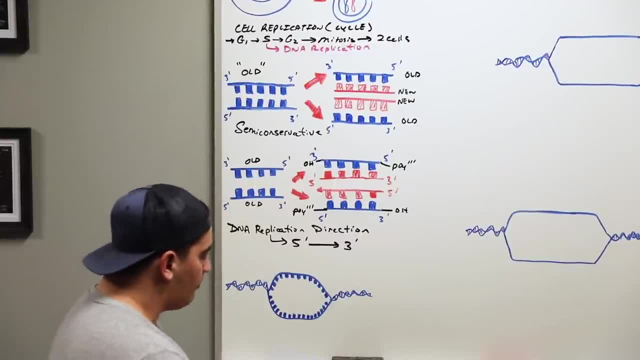 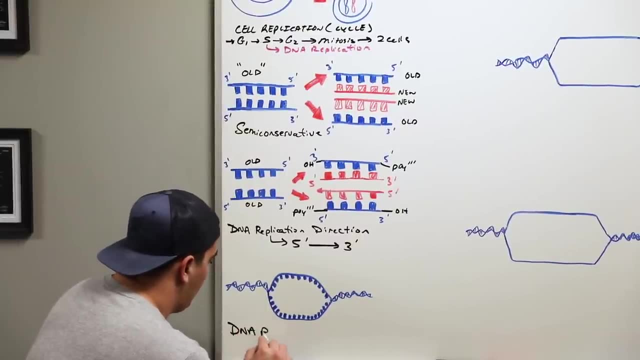 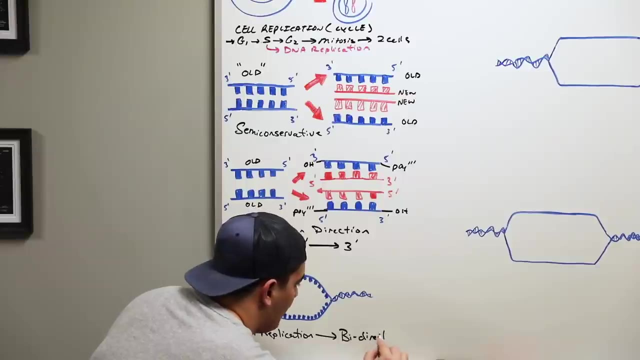 remember is that DNA replication occurs in a five to three direction. The last fundamental thing that is really important here is that DNA replication is bi-directional And you're like: why the heck do I need to know that? I think oftentimes when we're looking in textbooks, we only focus on one end where DNA replication is. 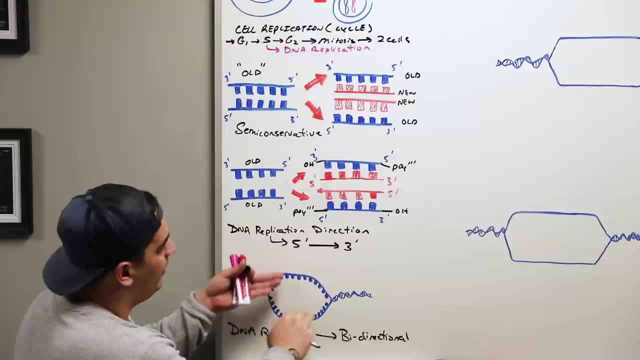 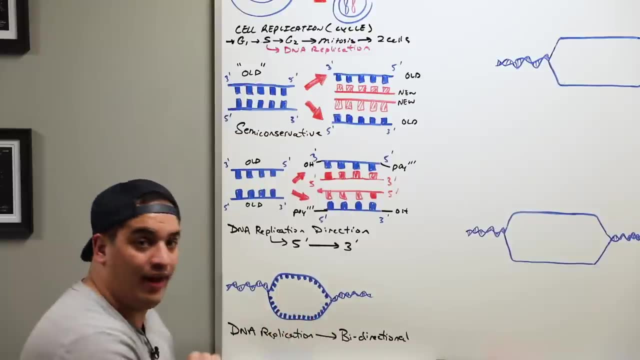 occurring. But what's really important is- we're going to talk about this in a second- but what we do is we take the DNA and we already have an idea that we're going to separate the two older parental strands away from one another so that we can create new DNA from that. When we do that, 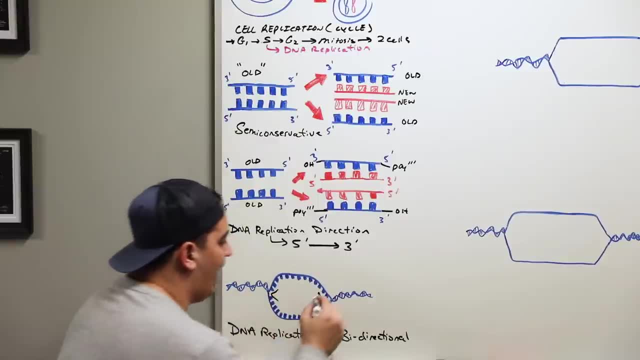 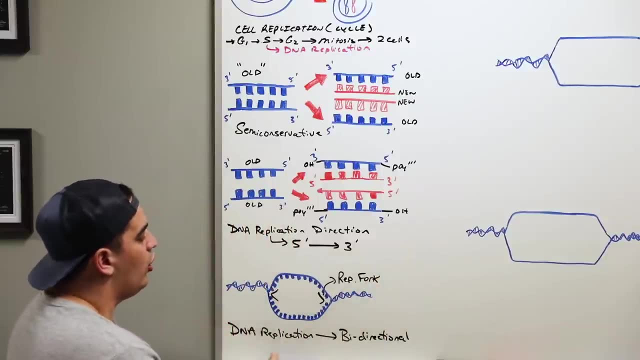 we create these little ends here, these little Y-shaped regions called replication forks. It's called the replication fork. You have two of them, one on this end, one on this end. There's going to be enzymes called helicases which are going to come in and unwind the DNA on both sides. 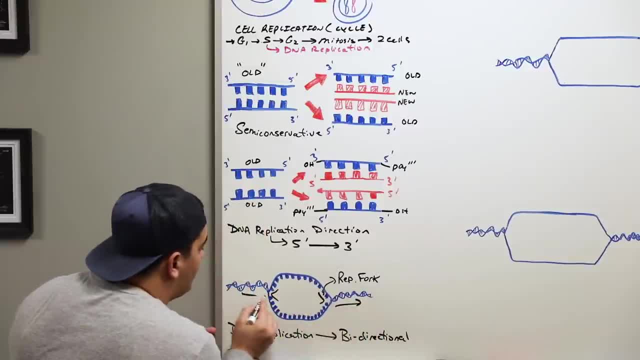 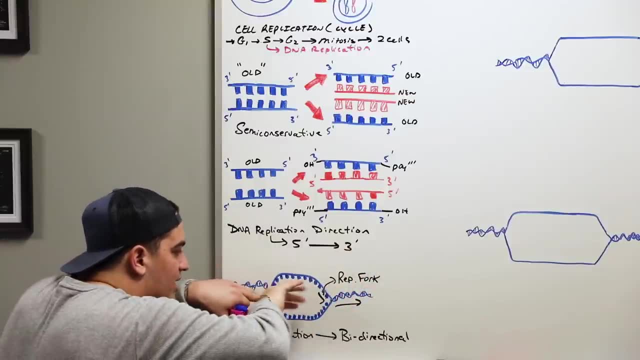 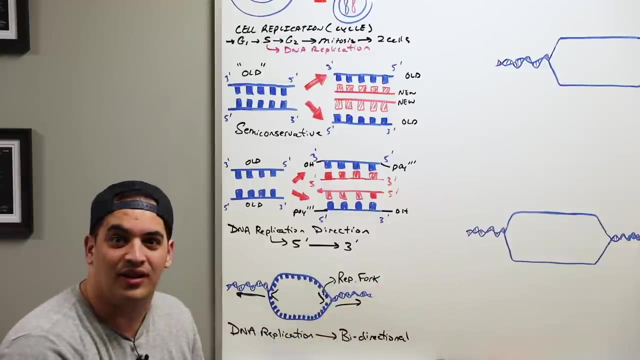 moving it in this direction. and moving it in this direction Then, enzymes called DNA polymerases, which we'll talk about, they're also going to move into these areas and follow the helicase causing new DNA off of that parental strand in a bi-directional fashion. The big fundamentals I 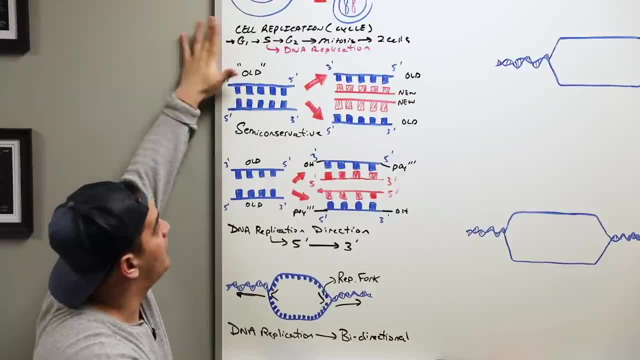 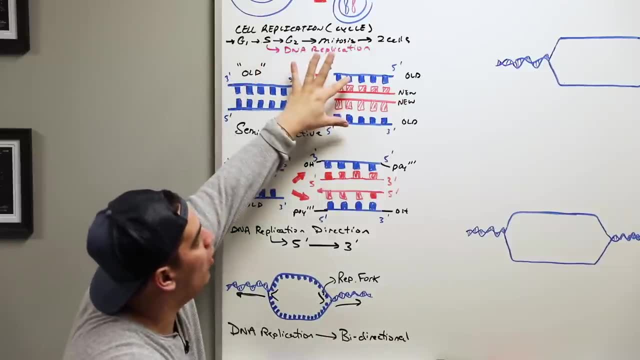 need you guys to take away is that? why do we do it? DNA replication in order for cells to replicate and make more cells. It occurs in a semi-conservative fashion, taking old, making a mixed old and new, two double-stranded DNA molecules. It occurs in a five to three direction. 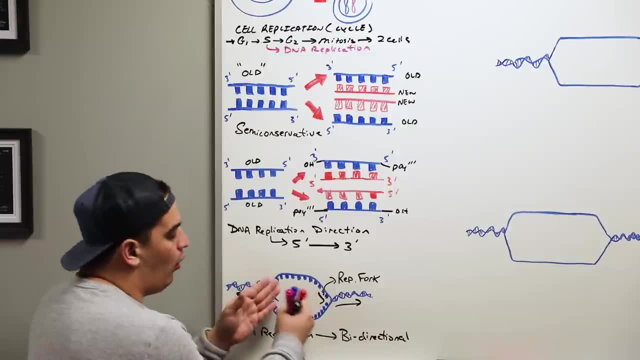 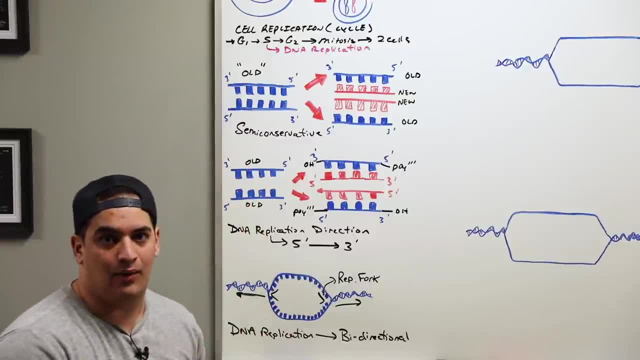 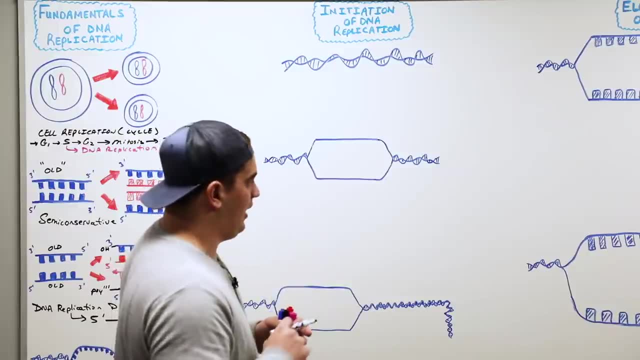 Now that we have the fundamentals, let's now talk about the steps of DNA replication. All right, So the first thing that we have to talk about when we're talking about the stages of DNA replication is three stages of DNA replication: Initiation, elongation and termination. Okay, 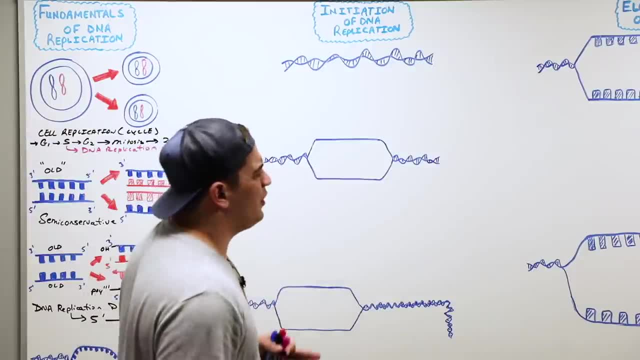 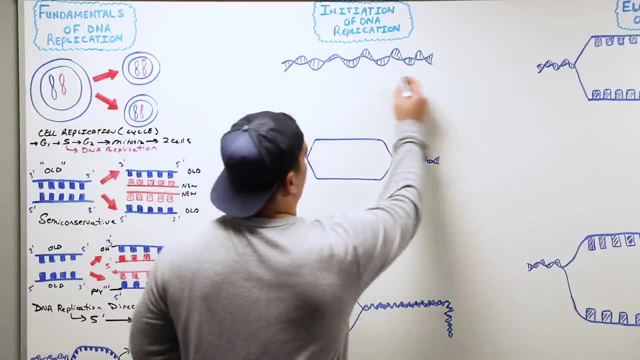 Initiation, elongation and termination. Initiation is really an easy process. It's not too hard to remember. So what happens is let's say that here I have my double-stranded DNA, Okay. And let's say there's a particular region. 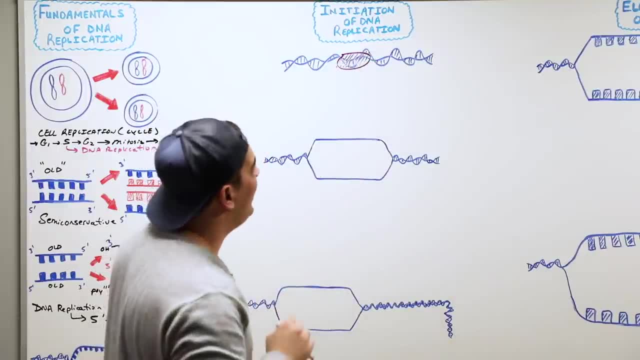 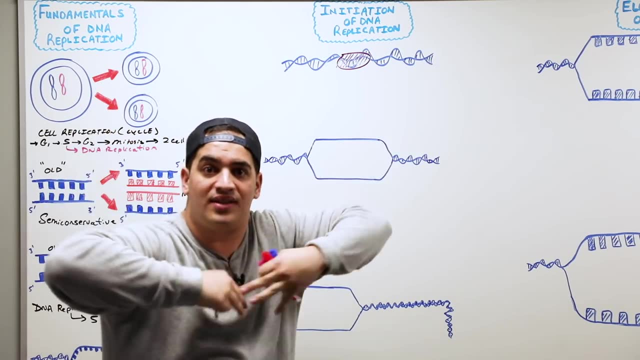 in that double-stranded DNA, which is really, really a nice little area that I want to go in and I want to separate the DNA so that I can create two separate DNA strands, parental strands, that I can use as templates to make new DNA. That area is going to become our origin of. 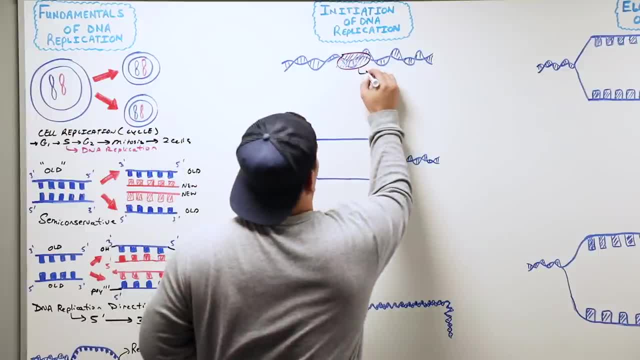 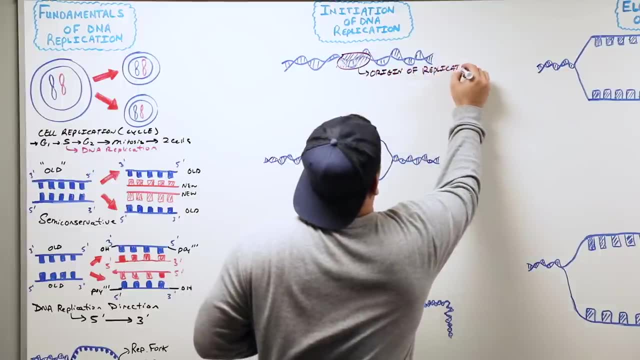 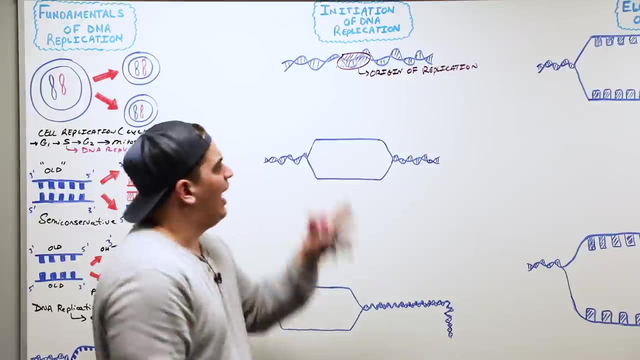 replication. All right, So this area is really what's going to be our origin of replication And why do we need to know this? Okay, So whenever we need, we're picking this spot, How do we determine what that we're picking that spot Like? okay, I know that there's a. 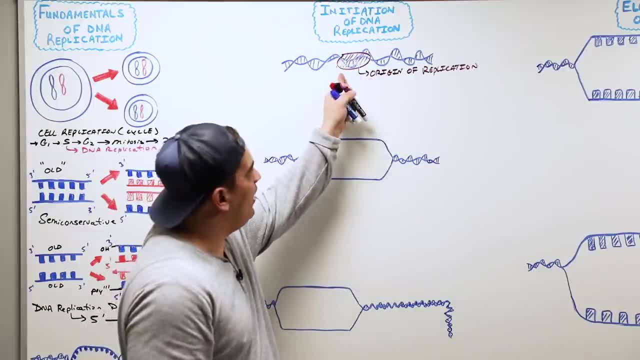 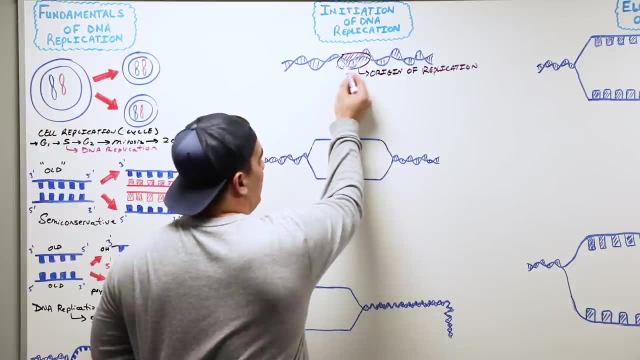 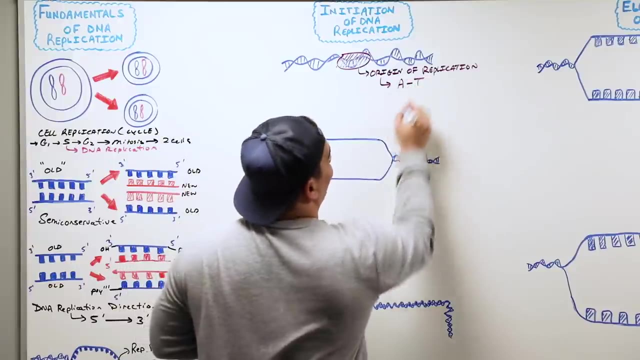 bunch of regions on the DNA. Why is this point here? the particular origin, And there's a really cool reason why There's particular nucleotides in this region which are really highly concentrated with adenine and thymine, So it's an adenine and thymine rich area. Now let's talk about this, for 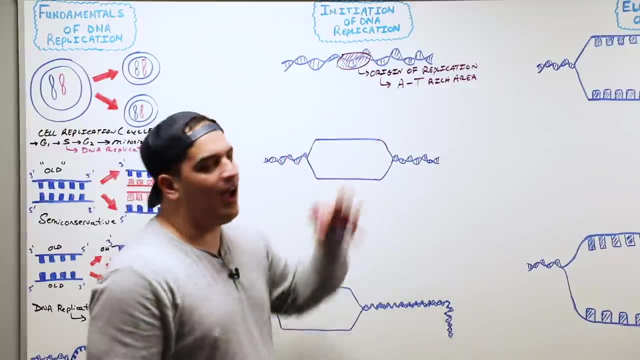 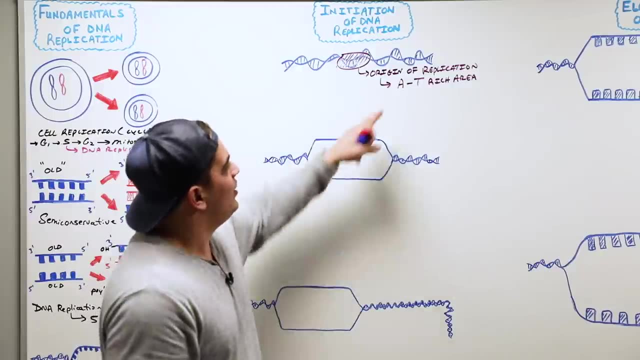 a quick second. Why would I pick? Why would I pick adenine and thymine as the area that I really want to target, as compared to guanine and cytosine? Do you guys know why? So adenine and thymine? how many hydrogen bonds are there? 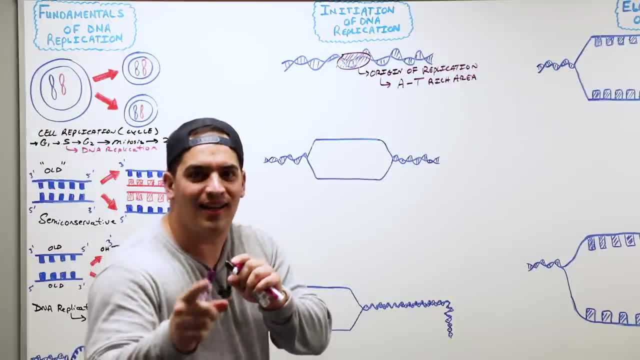 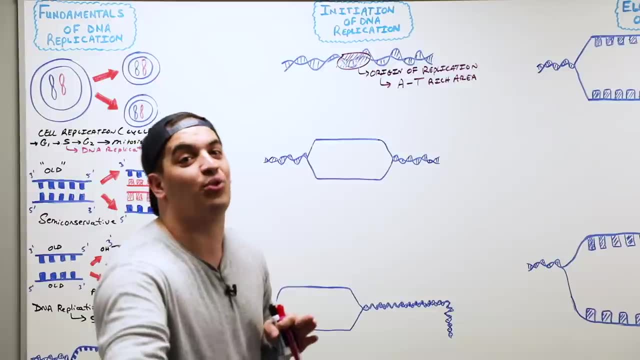 between them. Two: How many hydrogen bonds are there between guanine and cytosine? Three: It's going to be easier to break two hydrogen bonds than it is going to be able to break three hydrogen bonds. So in this area there's going to be particular areas which are really concentrated. 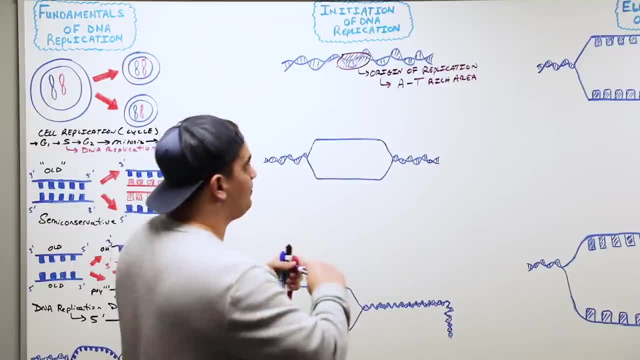 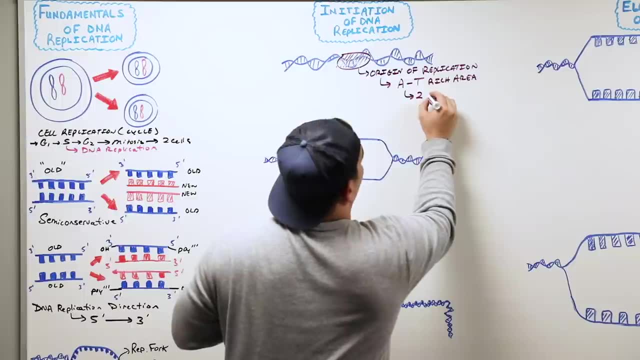 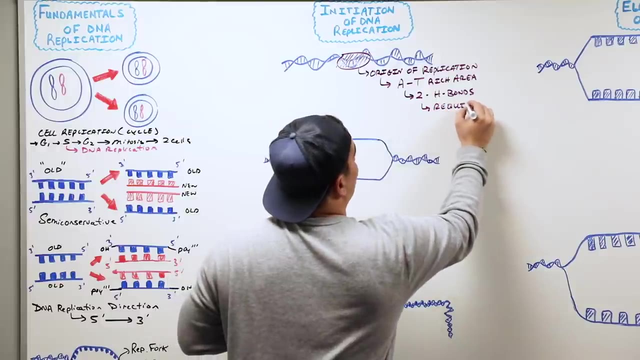 with adenine and thymine, nitrogenous bases or nucleotides. So in this area there's going to be fuckingктonucleides and that's going to be better suited as the area we want to kind of separate. Why? Because there's only two hydrogen bonds And that's going to require less energy. 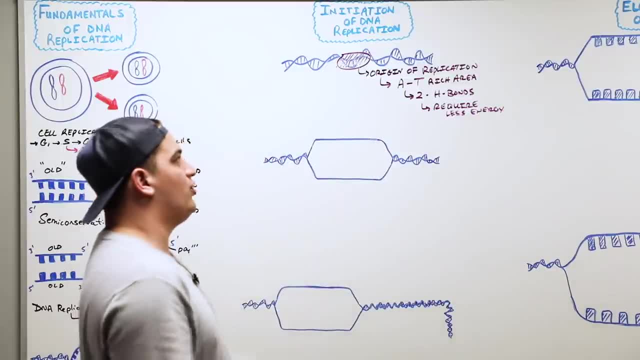 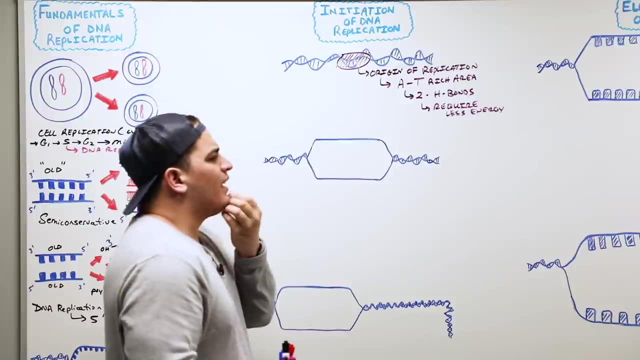 OK to break those hydrogen bonds as compared to guanine and cytosine. Okay, so that's the first thing. we have particular areas. Now. the next thing I need you guys to understand is eukaryotic cells. Is there only one origin? that? okay, there's just one area here where there's a 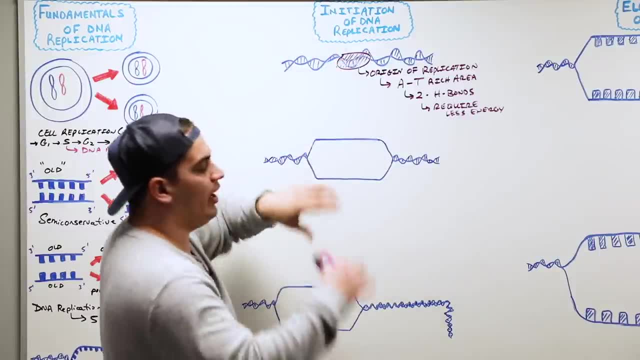 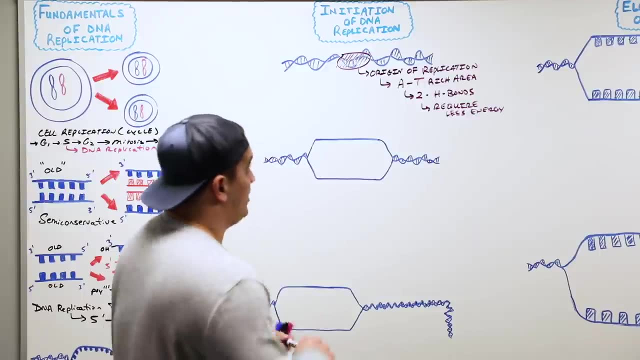 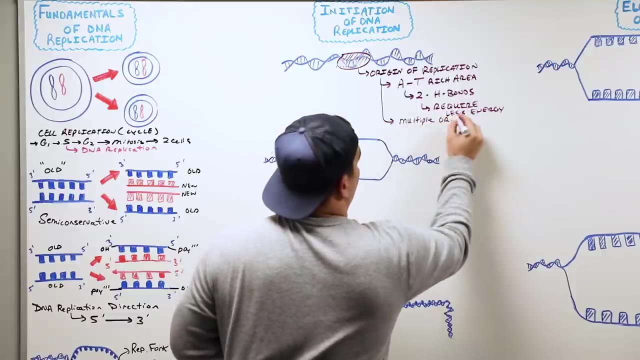 lot of adenine and thiamine. I just have enzymes bind to that portion and separate it, And the enzymes just work from the center and go to the ends. No, What's really important that you guys need to know is that in eukaryotic cells there is multiple origins, sometimes represented as O-R-E-C. 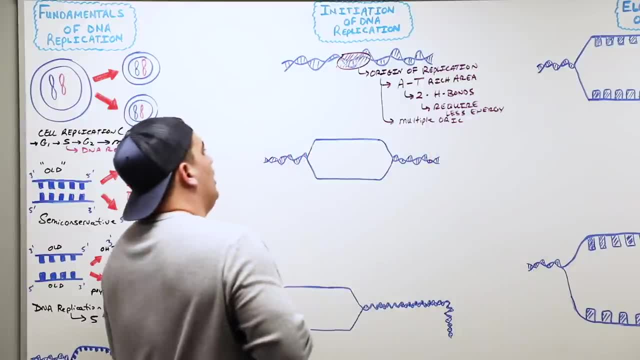 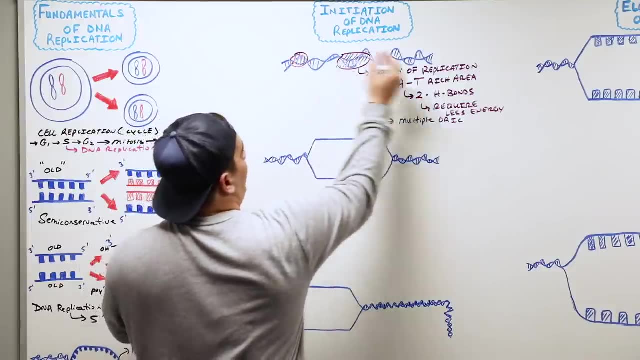 origins of replication. So that's really, really important. So, for example, I may just be representing this one portion, but there may be another origin of replication right here and another origin of replication here which is really rich in adenine and thiamine nucleotides. 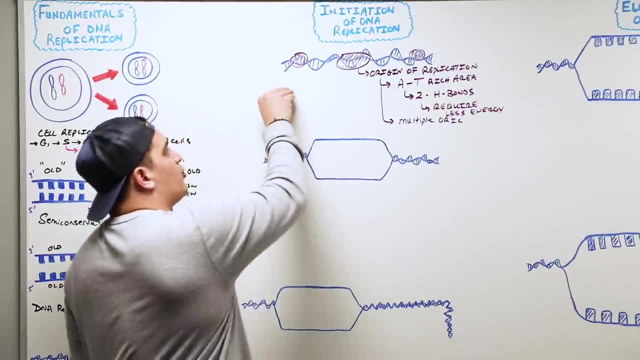 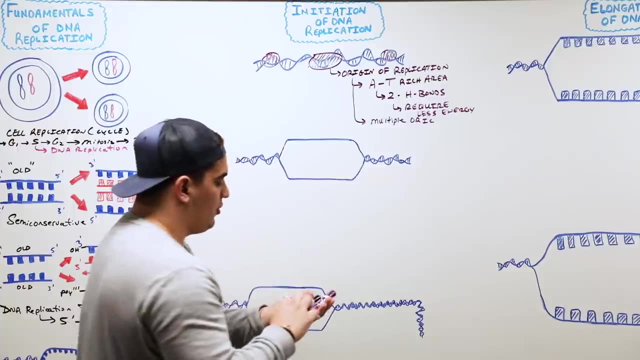 Okay, So that's one important thing. The next thing is: what type of structure is going to bind onto these areas and help to break the bonds between the adenine and thiamine? What do we have? There's a really interesting protein. 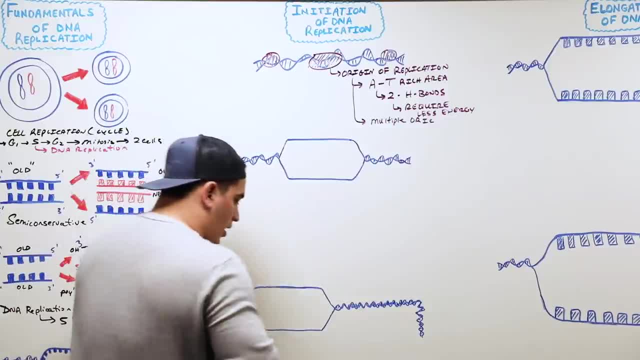 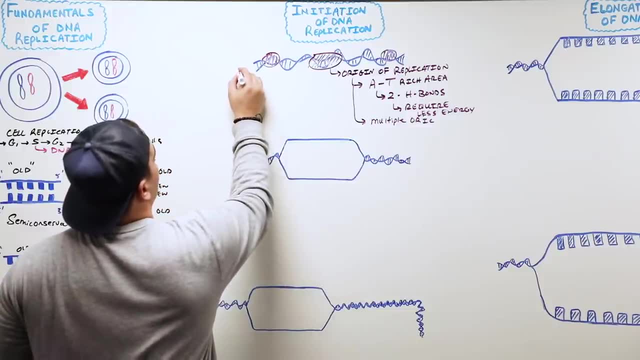 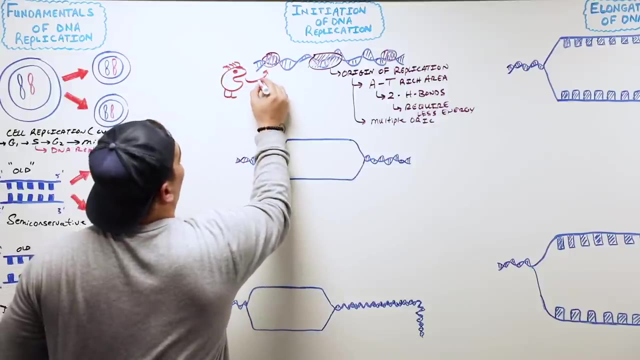 It's got one heck of a name. They always do, don't they? And this protein here is called the pre-replication protein complex- One heck of a name. So here we're going to draw a cute little enzyme here. Okay, This is a cute little enzyme, And this enzyme is going to come in and bind. 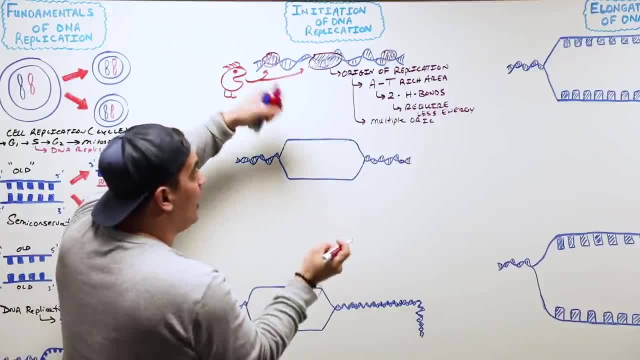 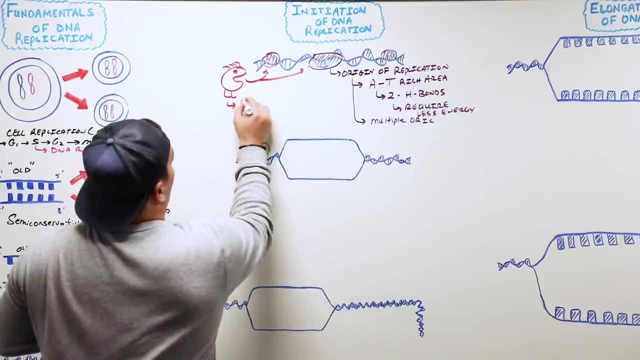 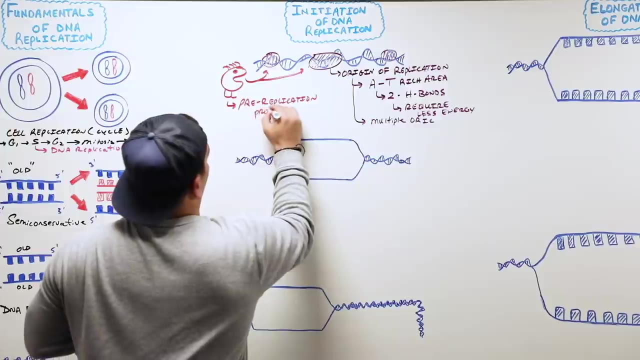 onto these areas And when they bind onto the areas they separate the adenine and thiamine nucleotides in that area to separate the DNA. What is this protein here called that separates them? It's called a pre replication protein complex. So again, it binds to the origin of replication, It separates the 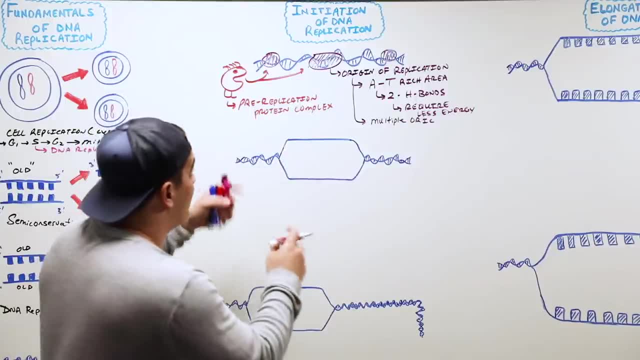 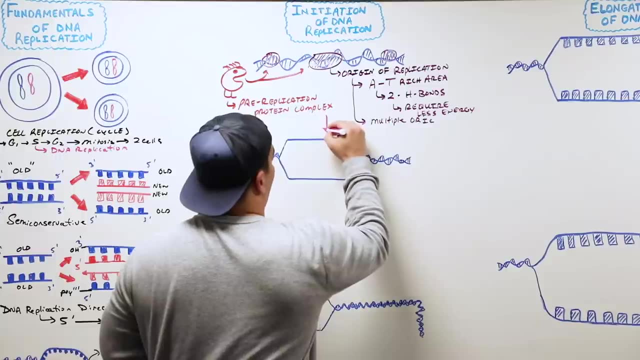 adenine and thiamine nitrogenous bases. Now, once it does that, what's that going to look like? Well, let's take the next step. We had this protein bind onto the origin of replication, where there's a lot of adenine and thiamine nucleotides. We separated the bonds between them, the two hydrogen bonds. 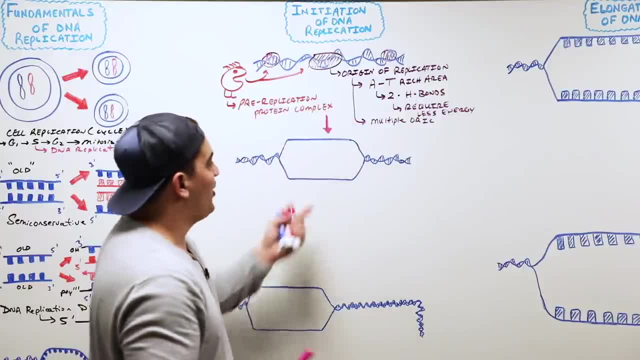 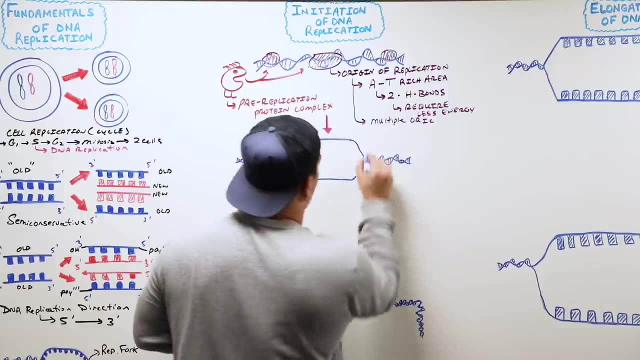 and we create this little bubble. if you will, Do you recall this? It's not hard. It's called the replication bubble. That's literally what it's called. I know it sounds crazy, But now we kind of form this little bubble due to this whole process And it's called the replication. 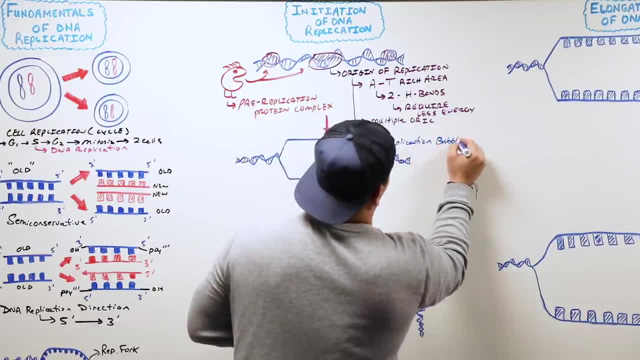 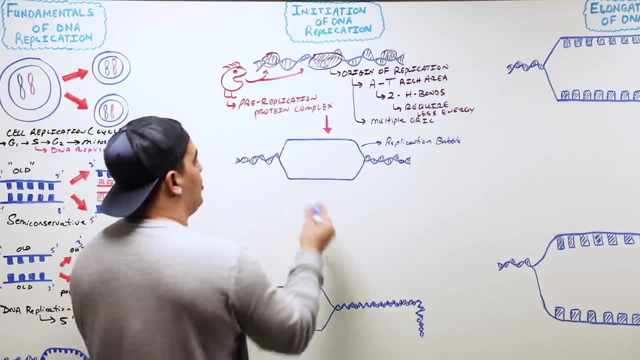 bubble. Now, once we form this replication bubble, there's a couple things that I need you guys to know. We have separated the nucleotides, So if you imagine here we're not showing them, but let's say that here I show a couple. you know, here's my nitrogenous bases that are coming off this sugar. 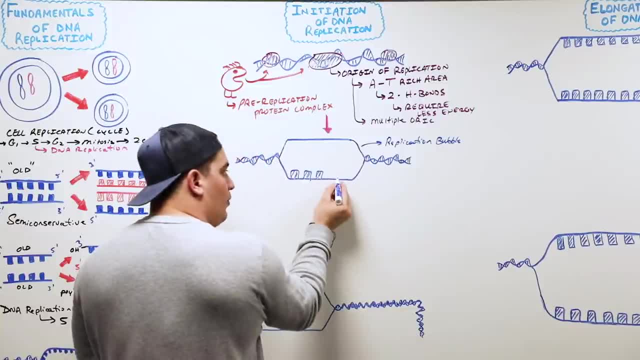 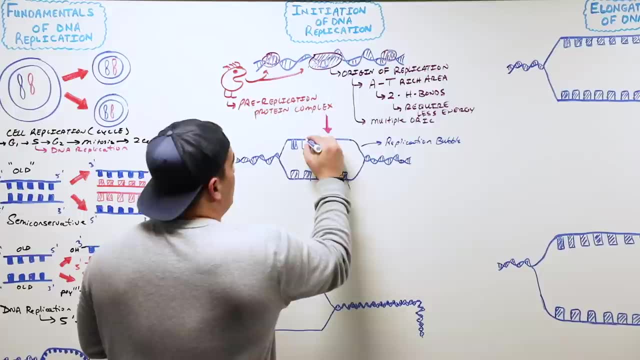 phosphate backbone right, Which is made up of a good amount of nitrogen, And I'm going to show you again the deoxyribose sugars, the phosphate groups, all that, And these are just my nitrogenous bases that are popping out off of it right. So I'm going to have these exposed now. So these were once. 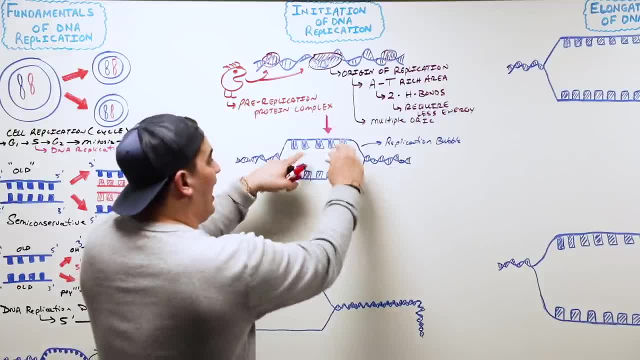 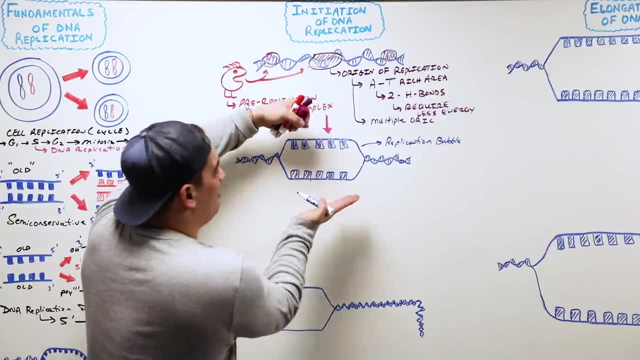 really connected nicely together, like in these regions. I really separated them, So they're really kind of like vulnerable right now. And you know what's really important, These, when you separate them, they want so badly to re-anneal with one another. All right, so what is this? 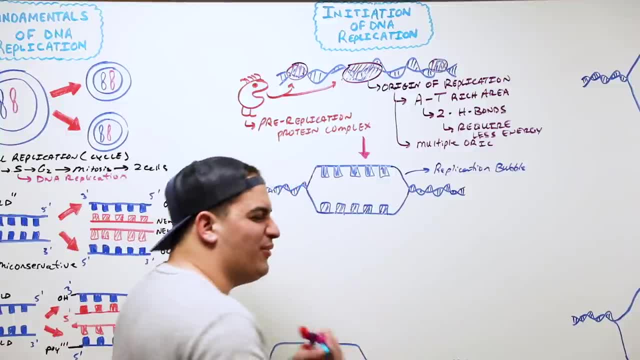 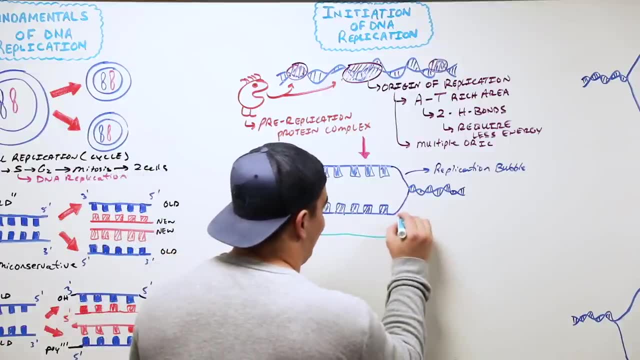 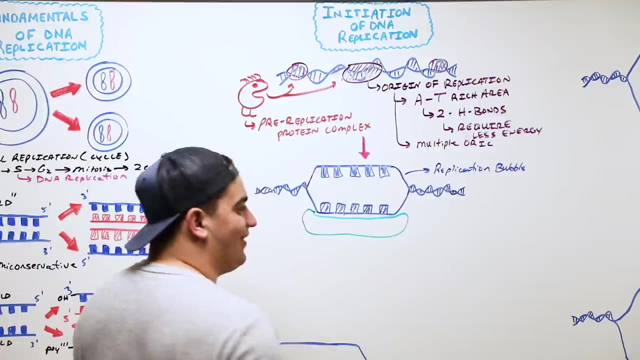 protein that really helps to protect these vulnerable separated parental DNA strands. You know it's really ironic, You know, sometimes science is: There's a big old protein that comes and binds to this and it would do the same thing on this one And this protein. you know what it's. 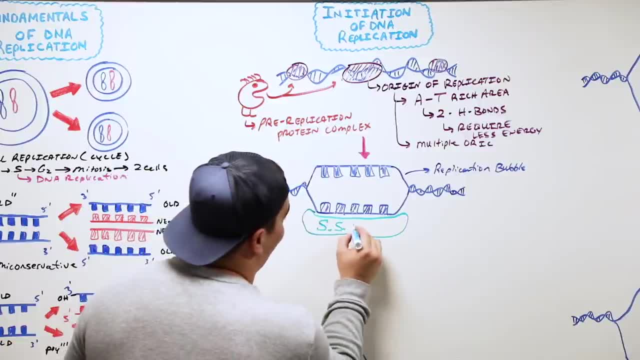 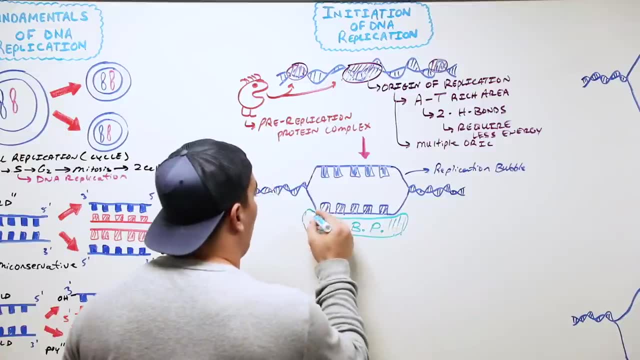 called. It's called the single-stranded binding protein. I'm not even joking, That's literally the name of it And it's perfect. It's not hard to remember Why. Because it's a protein binding to a single parental strand. So you would have one over here. I'll just 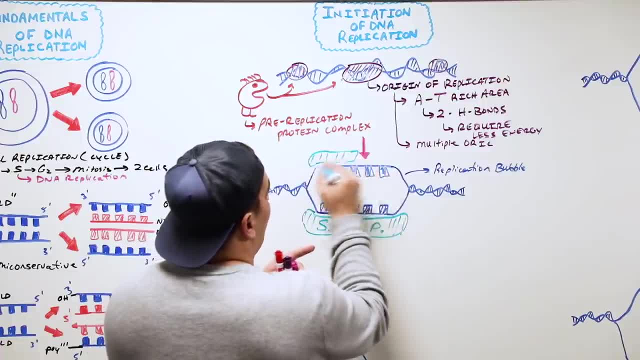 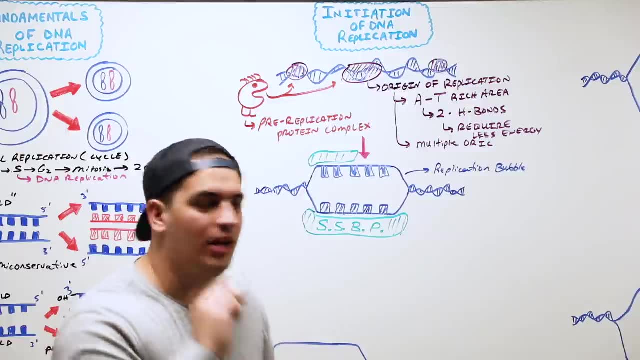 draw a portion of it, But you'd have the same thing over here: another single-stranded binding protein binding onto this parental strand. And what is the purpose of these single-stranded binding proteins? That's what I really want you to remember. One of the functions is that. 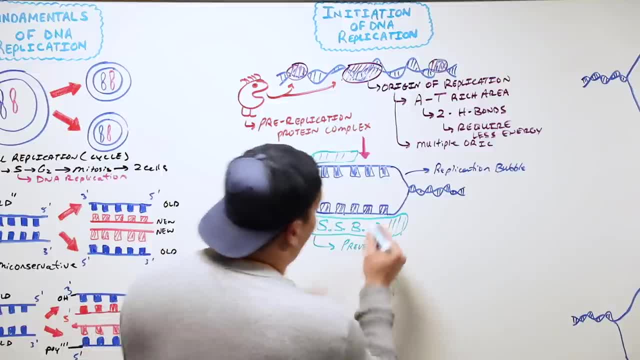 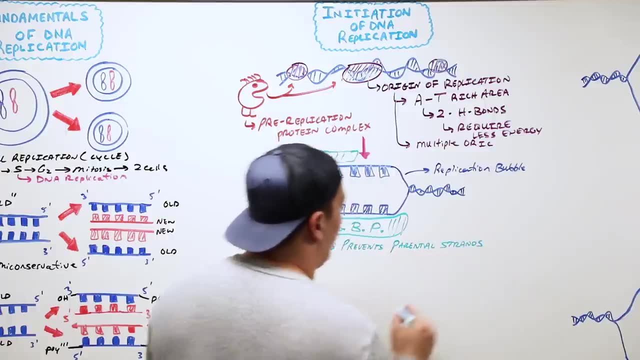 it prevents the parental strands from re-annealing. What the heck does that mean? What's that term? re-annealing? Re-annealing From reconnecting to one another, right? So that's important. So it prevents the 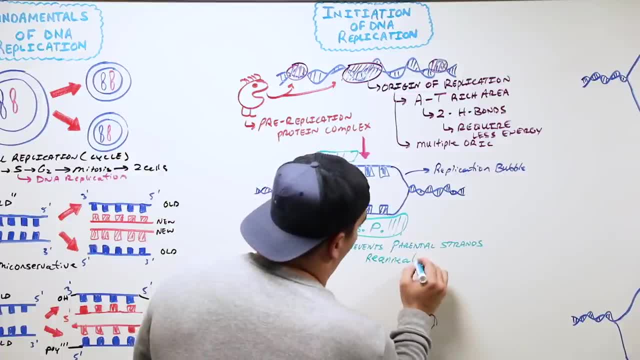 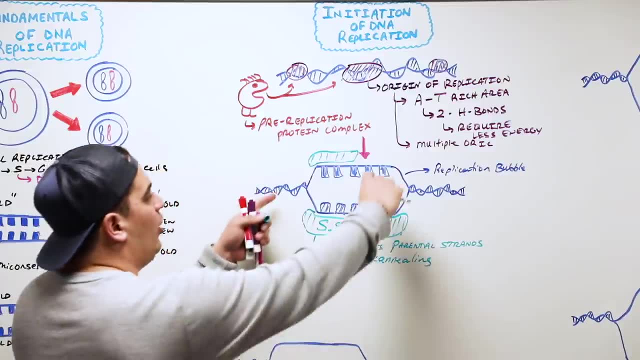 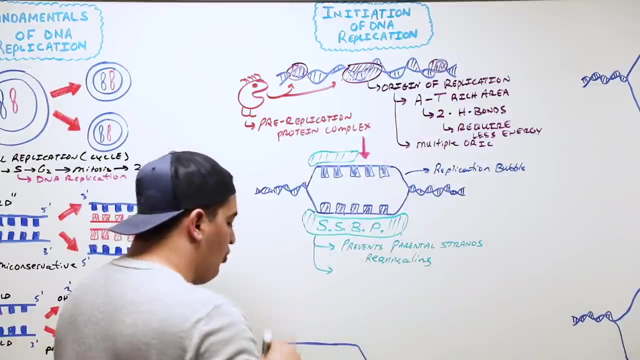 parental strands from re-annealing to one another Because, honestly, they really want to click back to one another. The other thing that they do is that when you have these parental strands separated as kind of these single strands, if you will, they're very vulnerable to very nasty little. 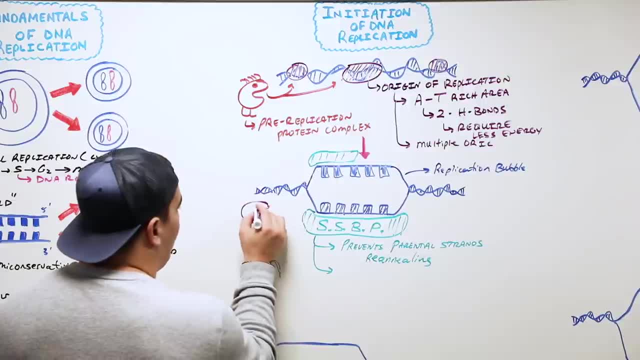 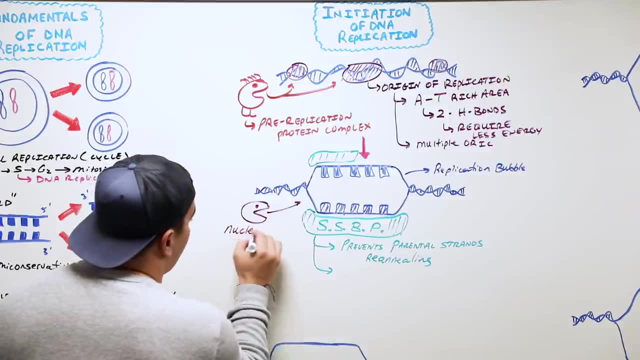 enzymes. There's some nasty little Pac-Man-like enzymes that want to come to the area and break them. They're called phosphodiester bonds. These are called nucleases. So what these single-stranded binding proteins do is they kind of act as a barrier and protect these. 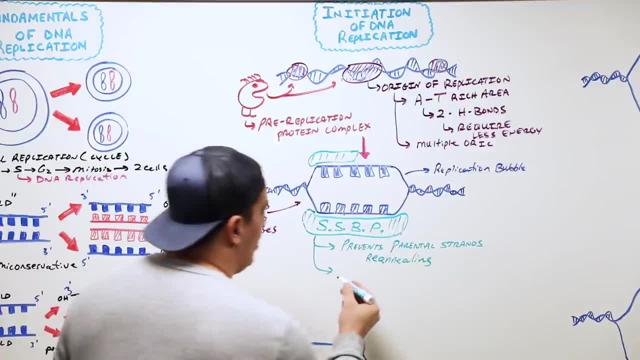 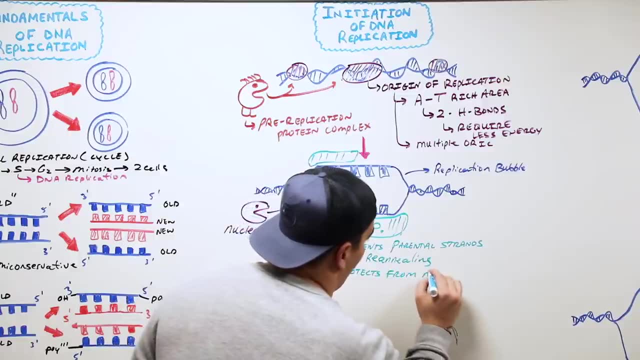 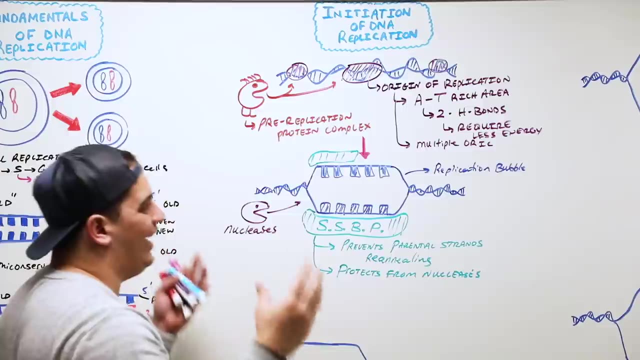 single strands from exonucleases or endonucleases. So again, it prevents, it protects from nucleases. Okay, So so far. pre-replication complex binds to the origin of replication or the AT-rich area. It forms a replication bubble. Single-stranded binding proteins bind to the single strands. 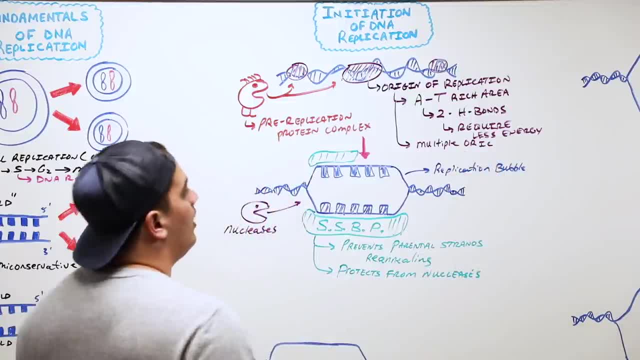 prevent them from re-annealing and protect them from nucleases. The next thing is, once you form a replication bubble, you form these two ends here. Okay, And these two ends- we already kind of mentioned it a little bit- This end here where it kind of like makes 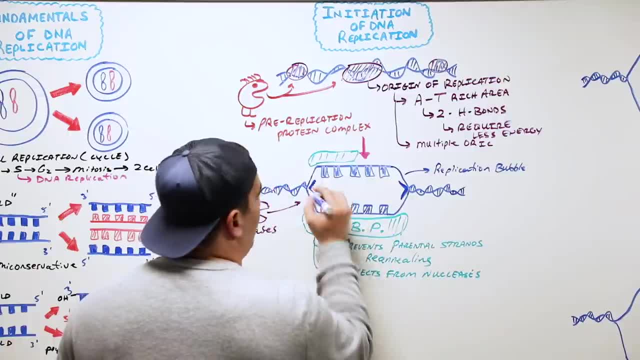 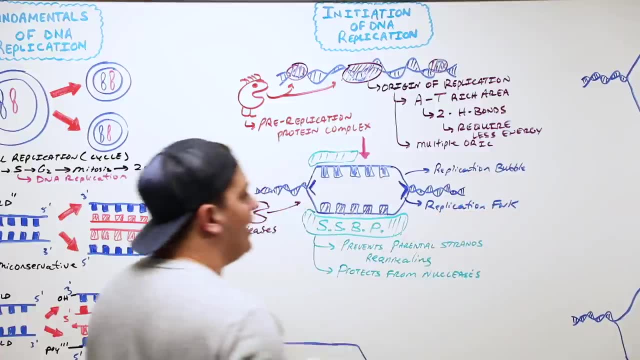 like a Y shape, if you will. this right here is called your replication fork. Okay, There's an enzyme that we're going to talk about in just a second. Ah, frick it. We'll talk about them now He hops in here. This little enzyme is like the energizer bunny He's got. 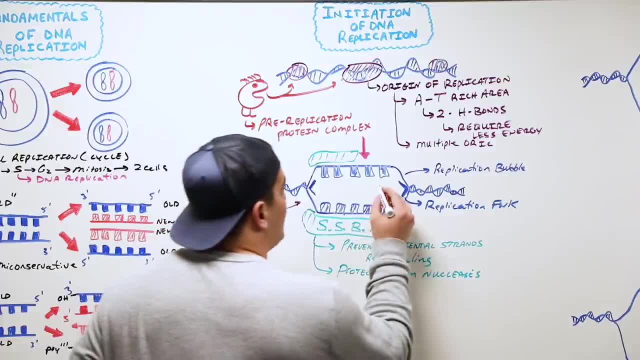 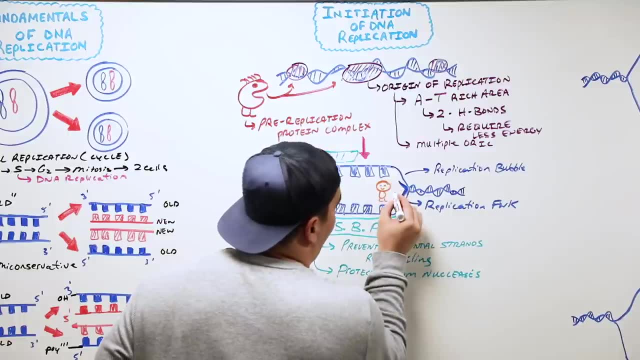 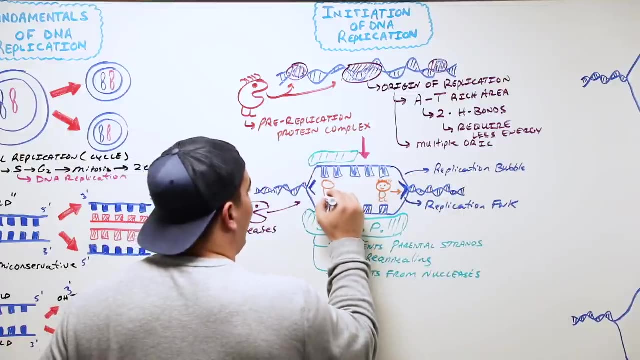 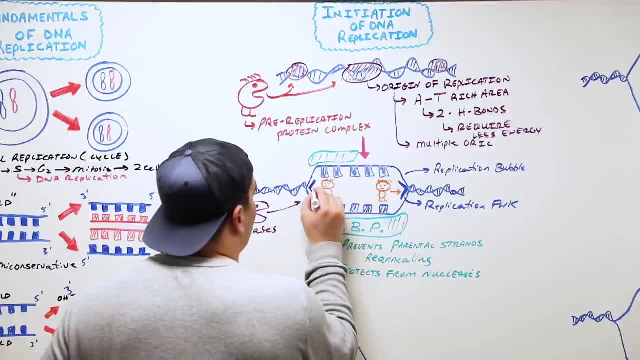 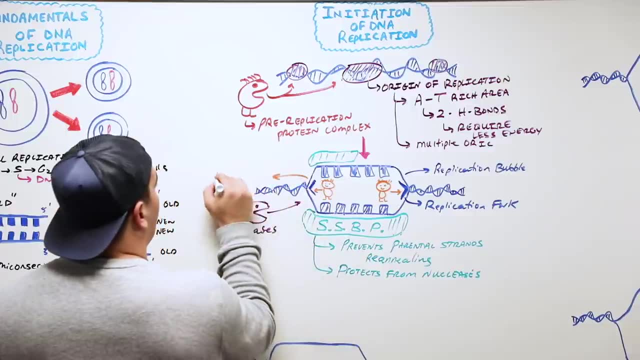 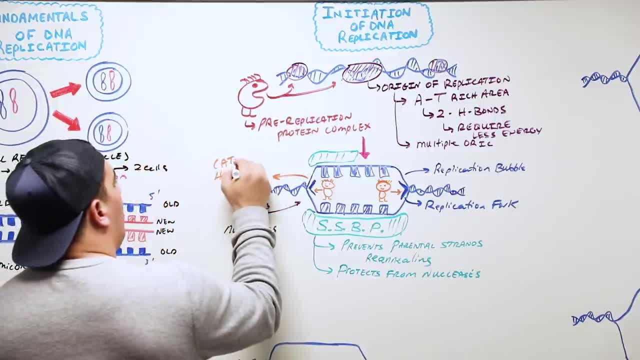 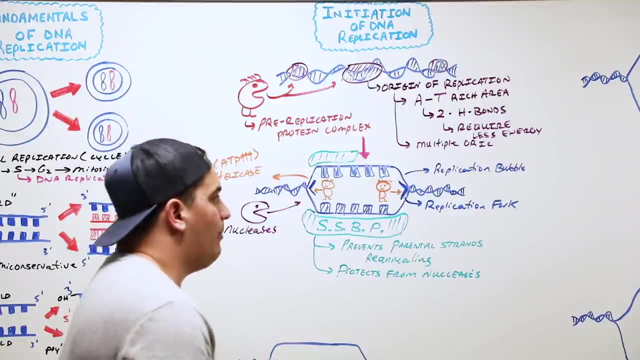 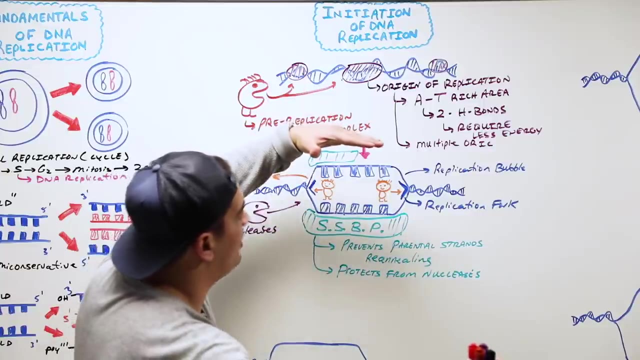 helicase enzyme is that he requires a ton of ATP in order to perform this process. Okay, So step-by-step again, real quick. pre-replication complex: binds to the origin of replication. AT-rich areas. single-stranded binding proteins bind: protect them from exonucleases and endonucleases, prevent. 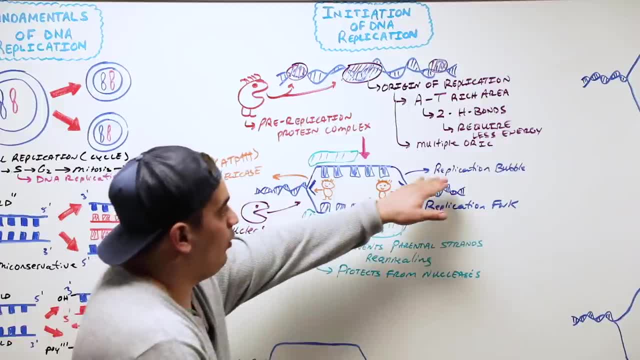 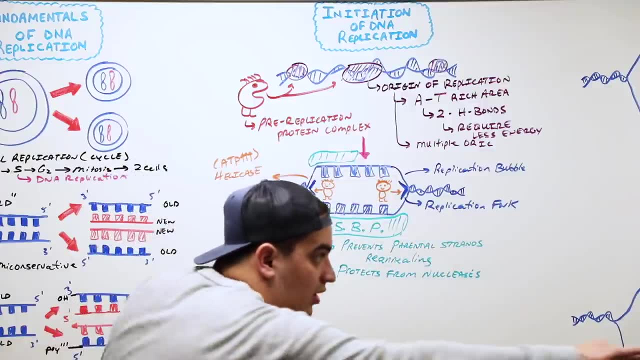 re-annealing. whenever you do that, separating them, you create a replication bubble. at the ends of them you have replication forks, helicases, highly atp dependent. hop in there and start unwinding the dna in front of them. after they do that, something happens, which is really important. 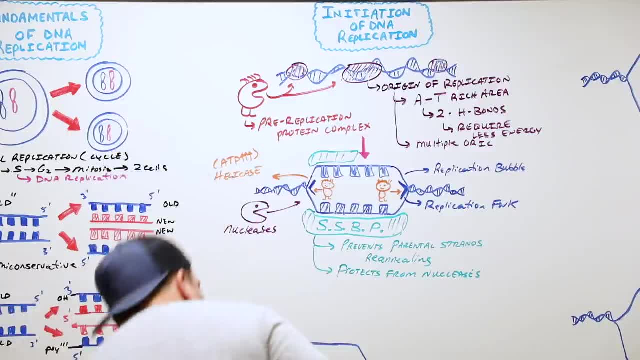 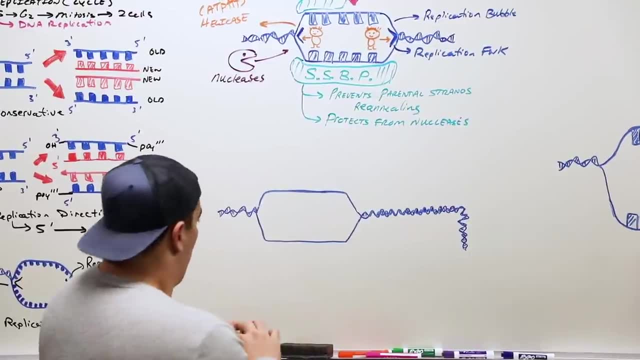 that we definitely need to know. let's come down here- and this is a really important area that i really, really need you guys to understand, so let's say that we come back to this point here again. what will we have? binding right here to these two ends: single-stranded binding proteins. 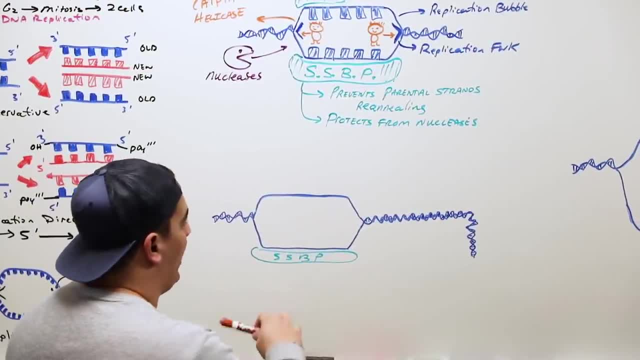 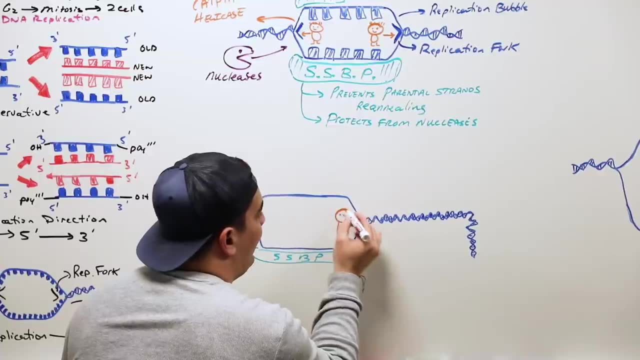 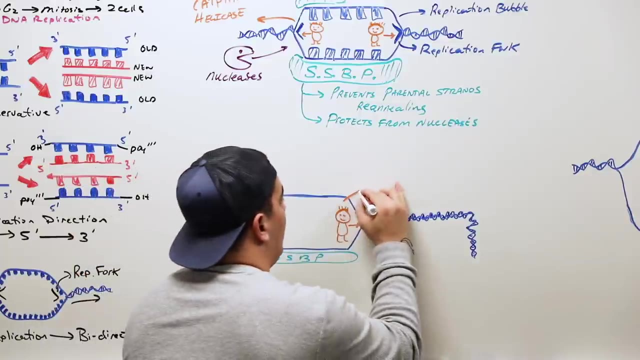 we're not going to show it on the top, but the same thing here. and then again, what enzyme? let's just focus on this area right here, just on this replication fork. what enzyme would be in this area here, really working and unwinding the dna in front of it again? that's called helicase. 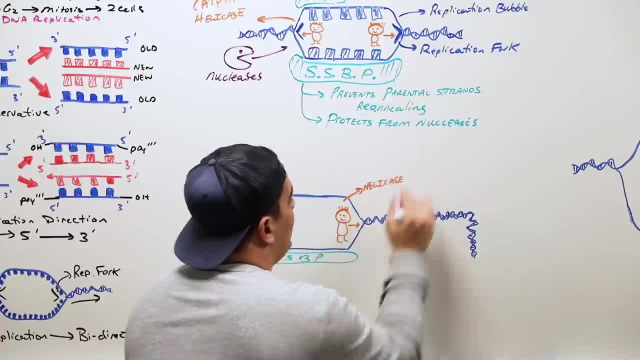 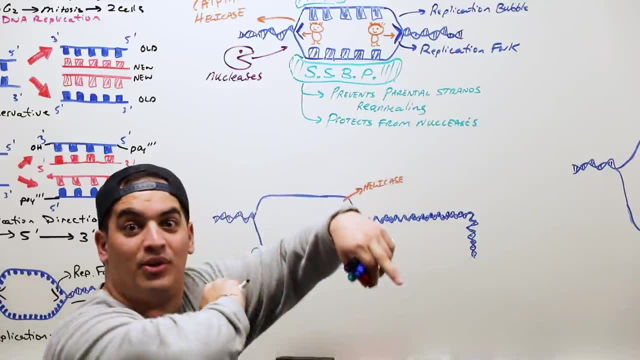 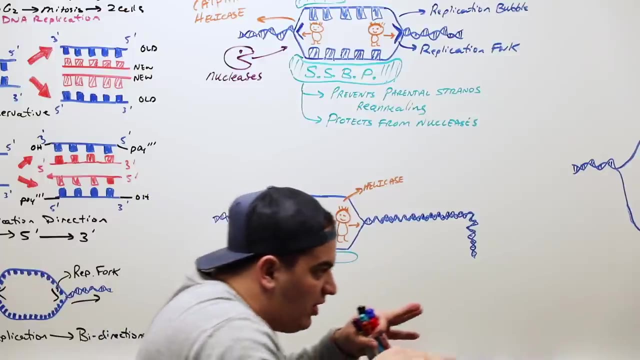 helicase. what happens is, as helicase continues to unwind the dna- the whole purpose of that- as it unwinds the dna separates the strands so that enzymes would be able to use those parental strands to make new dna- okay. but there's a problem. that happens as dna helicase is just, you know, going. 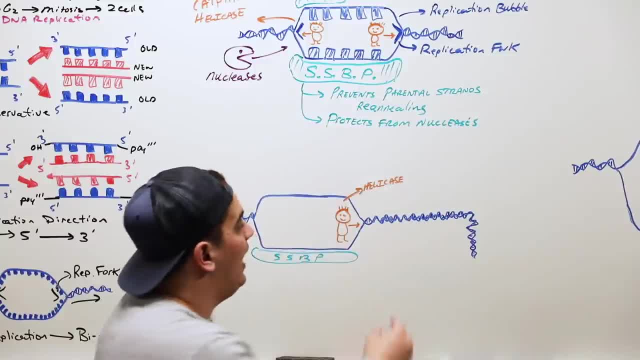 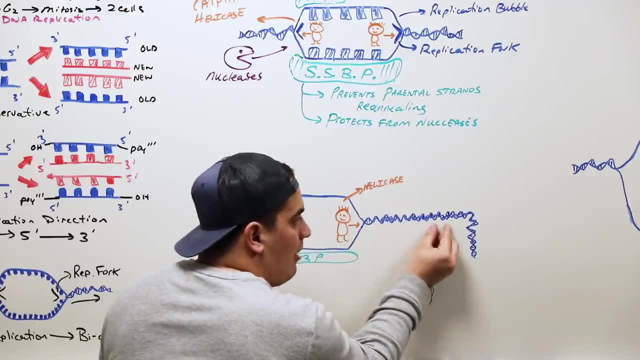 through those mofos and unwinding the dna constantly in front of it, it bunches up the dna in front of it distal to it. okay, from that replication fork so distal to the replication fork downstream, the dna is going to be able to make new dna, so it's going to be able to make new. 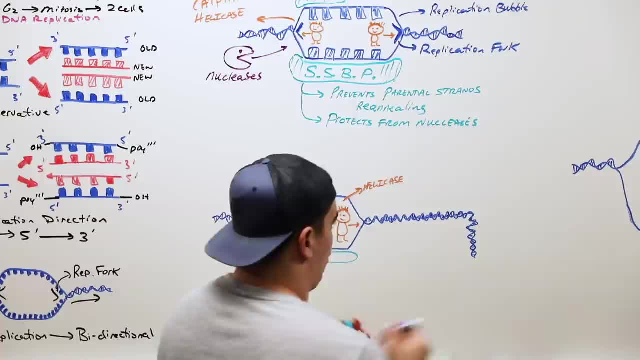 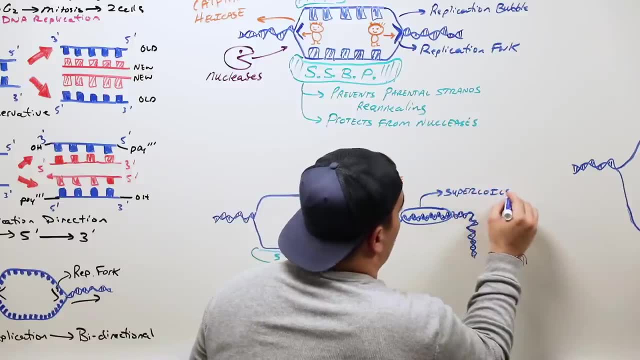 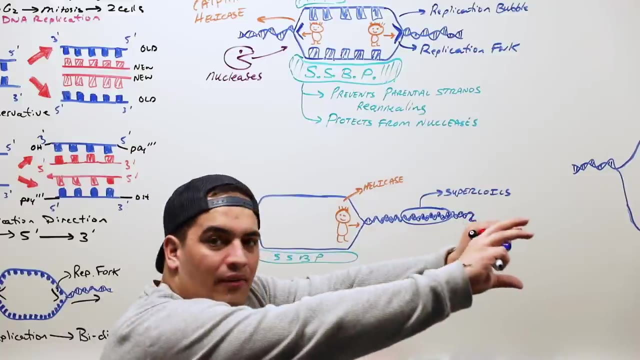 dna. so the dna starts bunching up and it creates things, these things called super coils. okay, it creates these things called super coils and this is caused by the helicase really unwinding the dna. why are super coils bad? if you really bunch up the dna in front of it, it's going to really 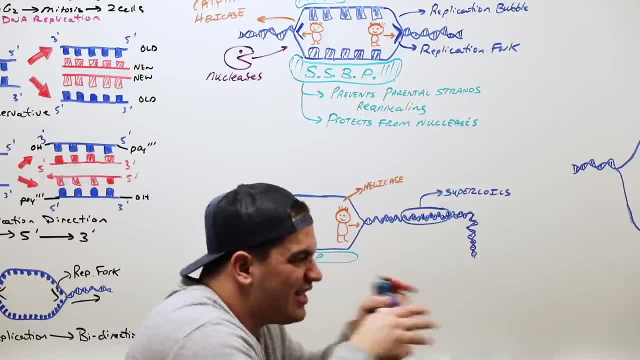 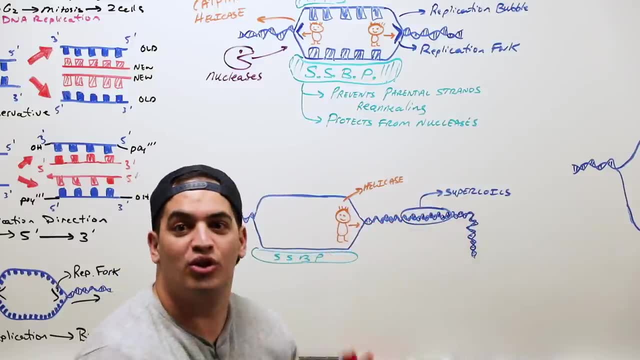 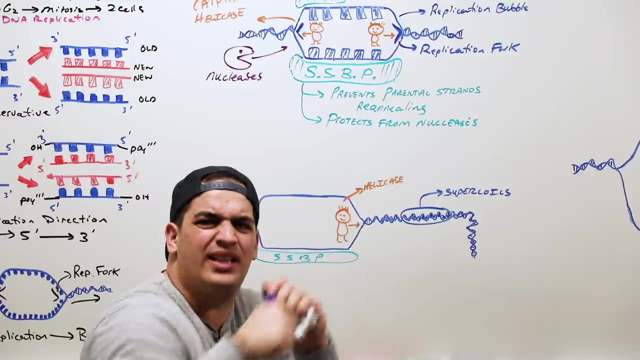 impede the helicase from continuing to unwind the dna. it's going to face a lot of restriction because it's really bunched up here, so to just keep getting bunched up until you relieve those. so we need enzymes that can come in there and fix these super coils where the dna is really, really. 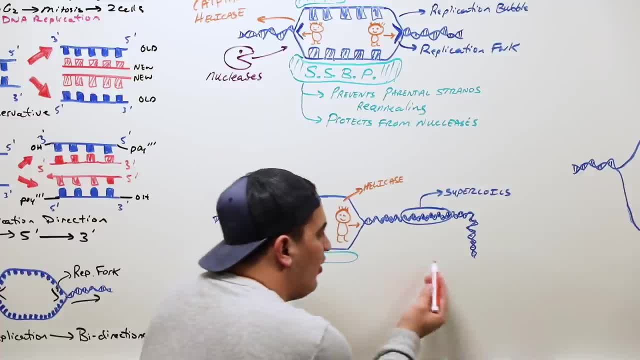 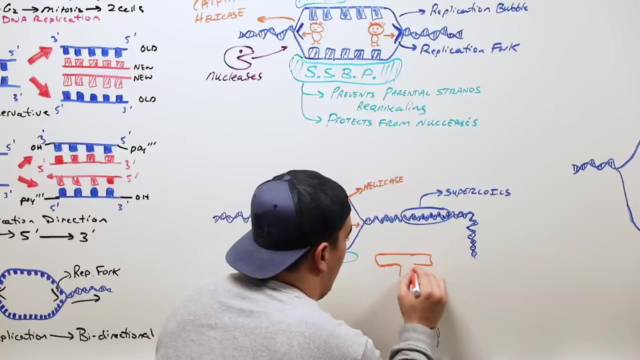 tightly wound. so how do we do that? all right, so what little enzymes do we have? are special little things that come into the play to really alleviate these super coils. these enzymes are crazy interesting. so these guys are really cool and they are called topoisomerases. they're shaped. 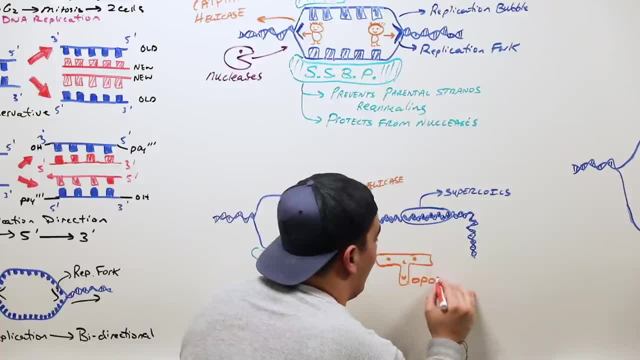 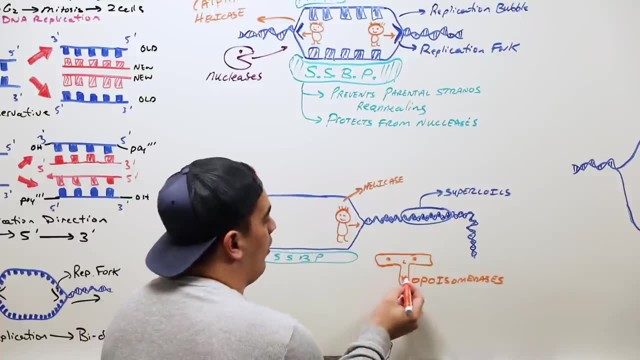 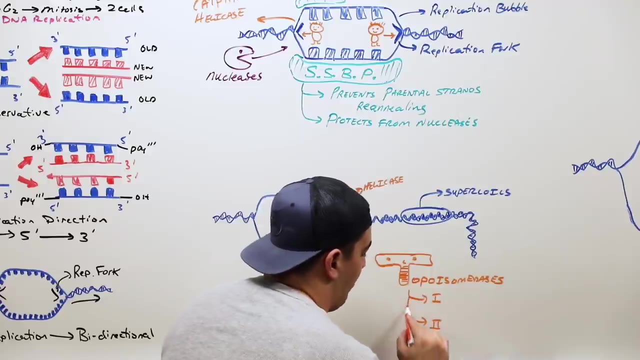 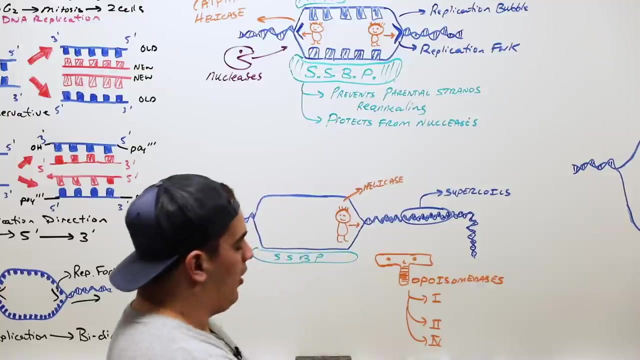 right, so they're called what topoisomerases. now, topoisomerases, there's actually a couple different types, okay. there's particularly type one, type two and then there's type four. for the most part, they all do the same kind of thing. and what is that? okay, this enzyme has two. 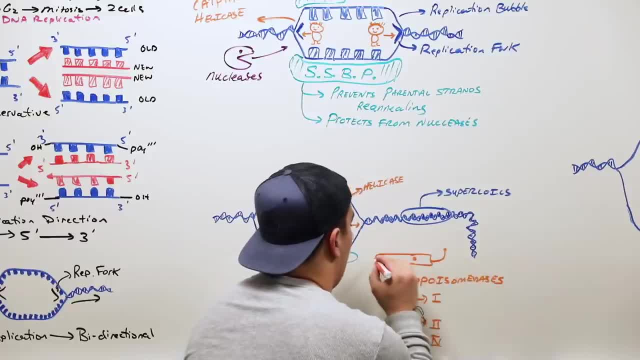 little arms, if you will. let's say, here it has one little arm and another little arm. on one arm it can go to where this area of the super coil is- let's say that the super coils right here. it can use a little enzyme, a little domain of it, and cut. 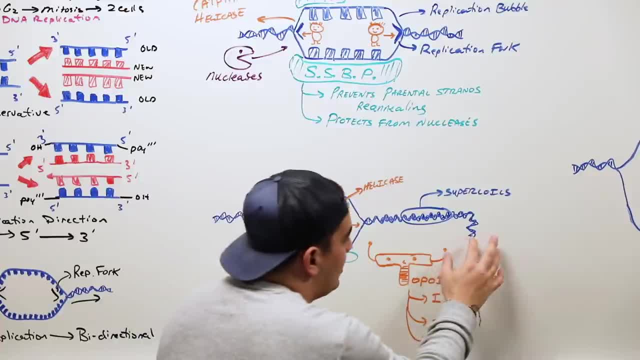 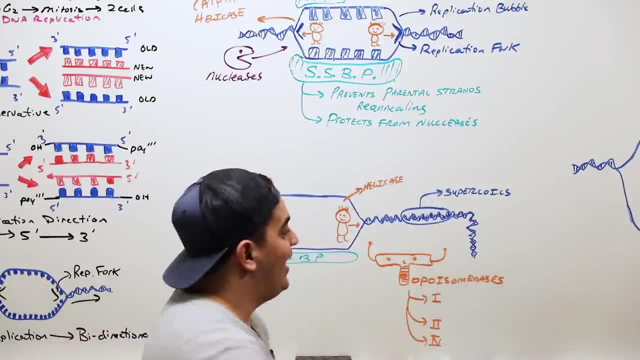 this dna strand. if it cuts the dna strand, what does that allow for it to do? it kind of allows the dna to kind of unwind a little bit and unravel. and so there's a particular name to this domain on that topoisomerase enzyme, it's called a nuclease. 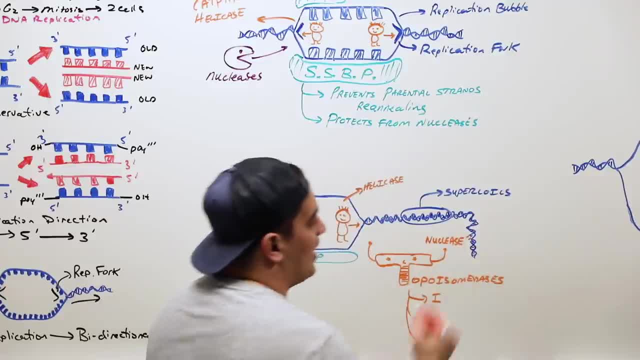 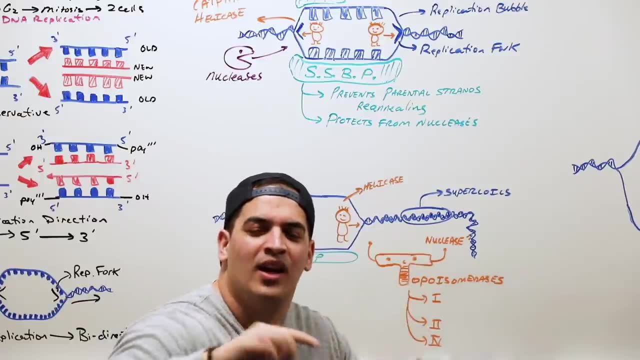 domain, and what does it do? it creates a cut or breaks the phosphodiester bond in the dna strands. one, maybe two dna strands allows it to unwind. there's a problem with that, though. if i just cut the dna strand and allow it to continuously unwind, that may be problematic. the dna could. 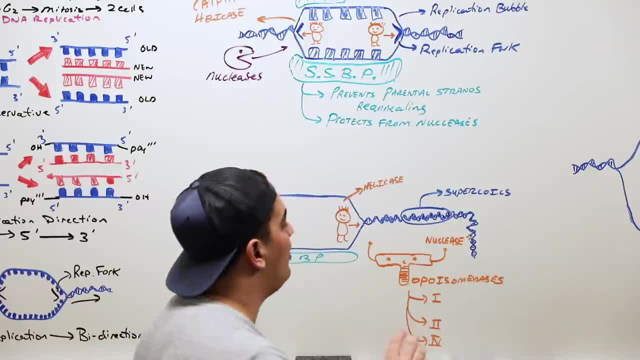 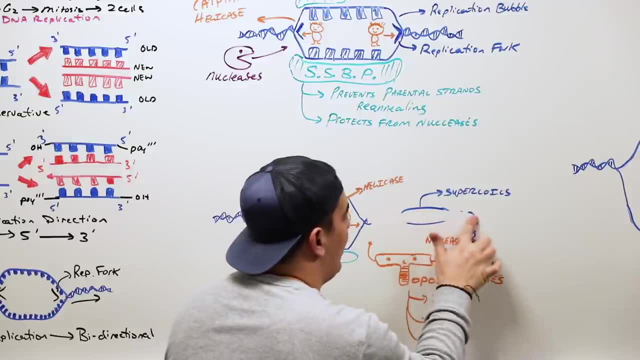 continue to fragment. i don't want that. so what i do is i use this other arm and after the dna super coils have been alleviated, so let's now kind of draw a new dna after the super coils have been alleviated. so we alleviated the super coils, we 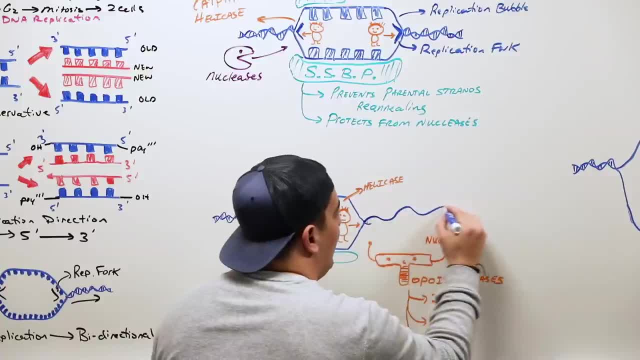 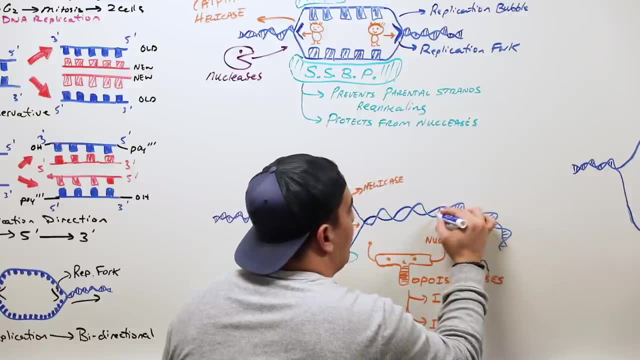 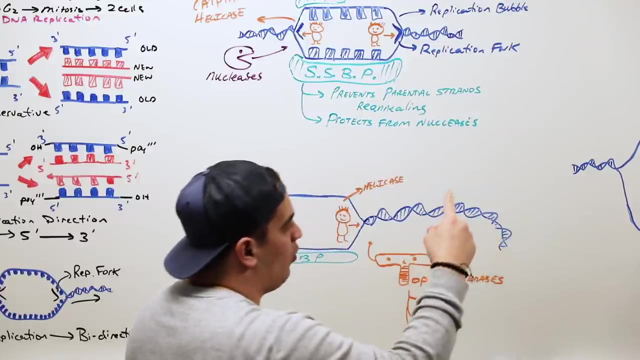 got rid of all of those over winding of the dna. look now it's beautiful, it's not over winded, but we have a break in that dna and that's a problem. so now we need to use the other arm of this topoisomerase, where we cut this portion here and allow it to unwind. we need to use this: 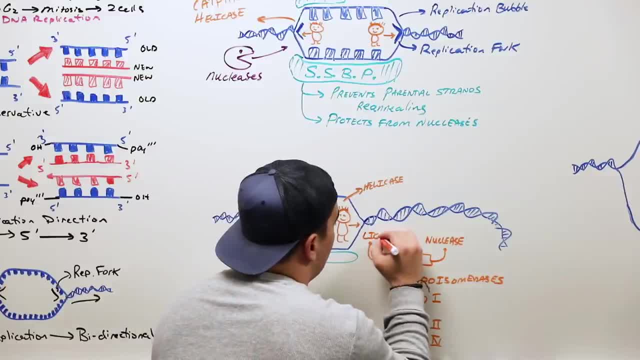 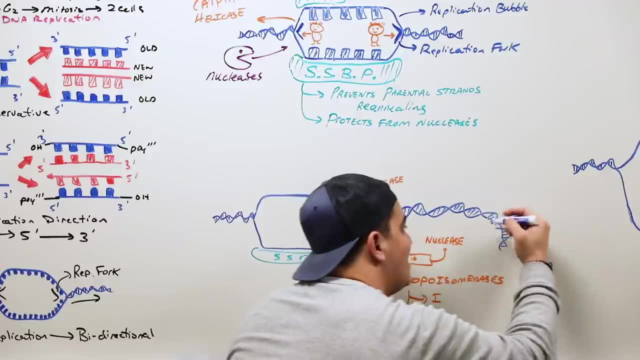 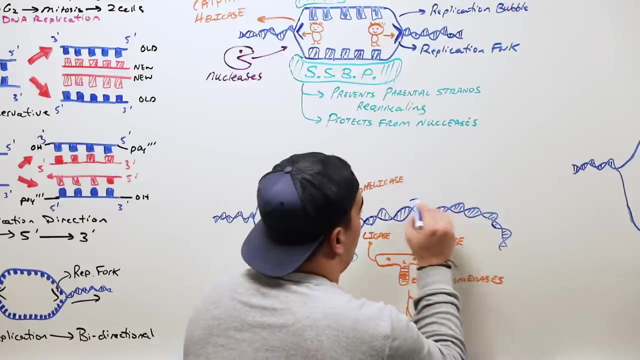 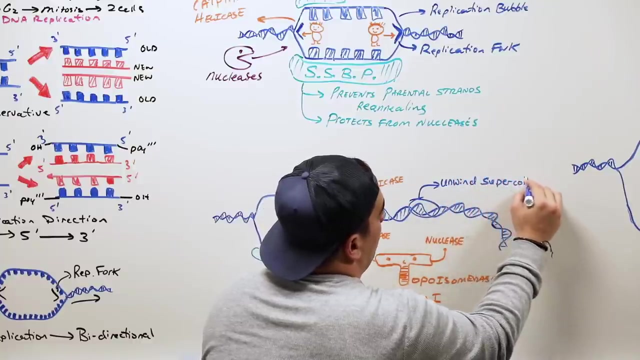 portion called the ligase domain. and once it's unwound this portion here, what does it do? it restitches this area back together after it's unwound the super coils. okay, so again the topoisomerases. what were their function? again to unwind the super coils. now, why in the heck did i take all this time to mention the topoisomerases? 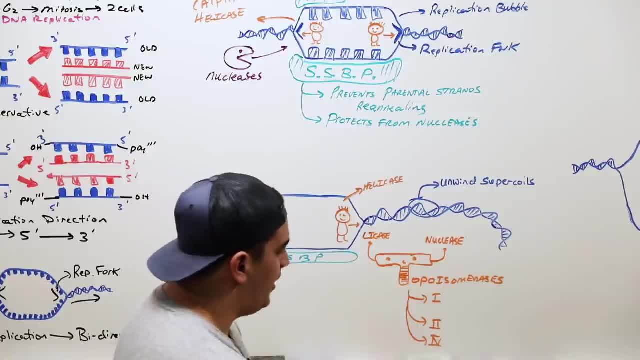 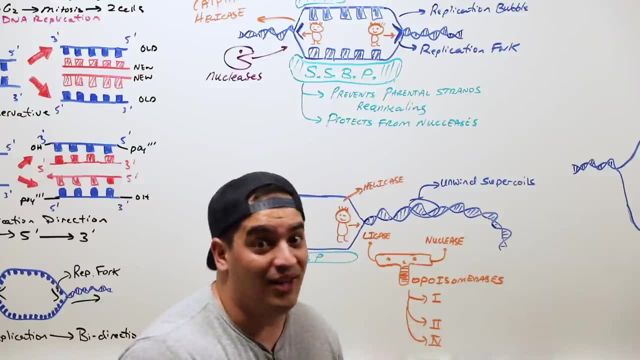 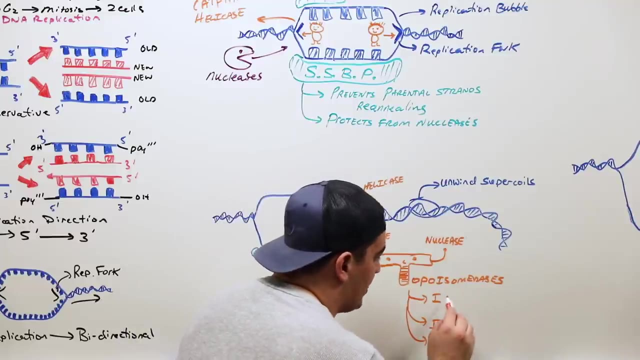 and there's different types. let me explain why. topoisomerases can be in both cells. so we primarily haven't really discussed that. dna replication can occur in bacterial cells and it can occur in eukaryotic cells, or we call it bacterial cells like prokaryotic cells and eukaryotic cells, human cells. primarily they have type 1 and 2. 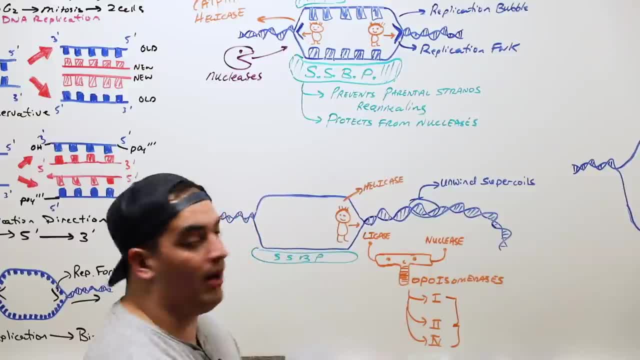 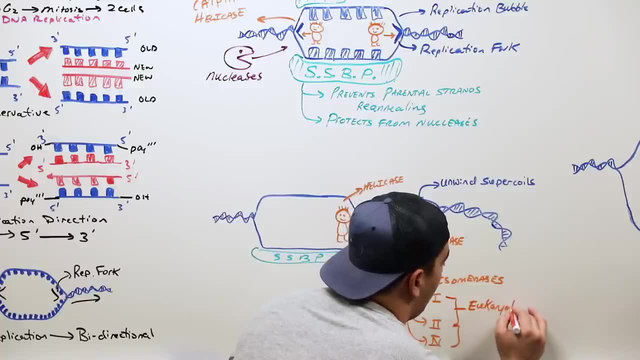 topoisomerases and in prokaryotic cells. they primarily have two and four. so again, type one and two are primarily for eukaryotic cells and then type two and four are primarily for for pro-karyotic cells. Big thing I need you guys to know is: 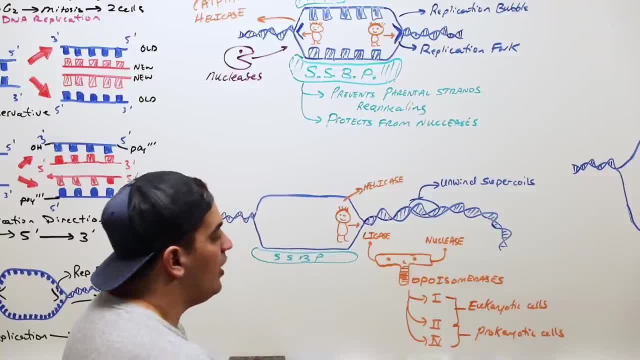 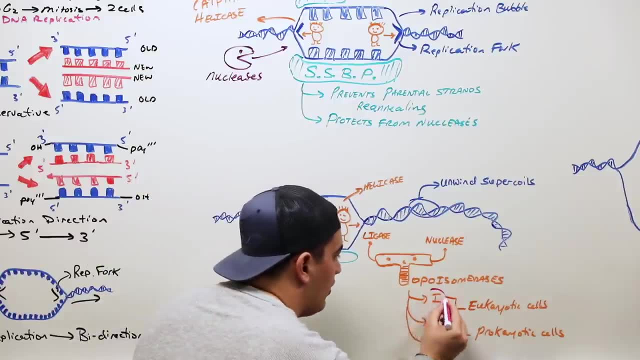 is that type one, topoisomerase, does not require any ATP to unwind the supercoils. So let's put that next to it, that just for this one, just for this one, no ATP is required in order for it to perform this unwinding. 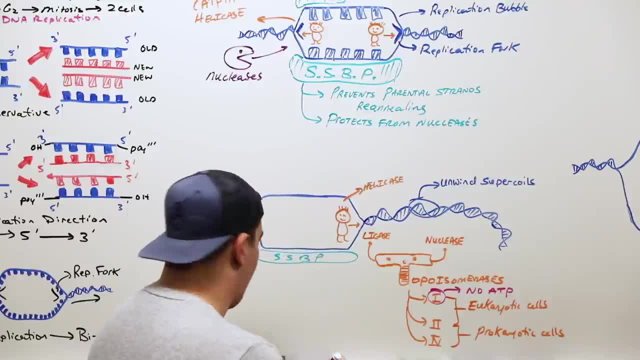 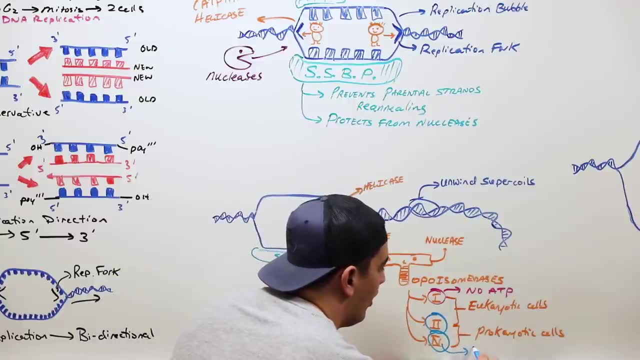 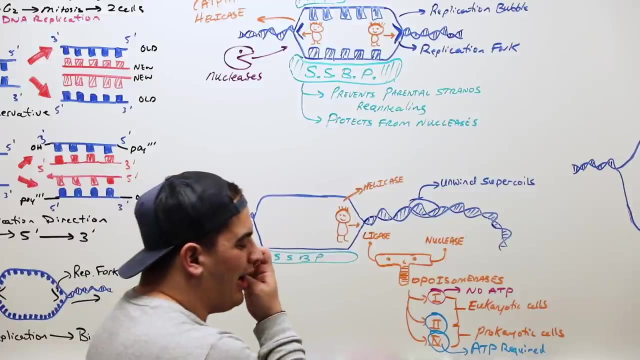 of the supercoils. But for type two and four let's pick a different color so that we don't confuse it here. for type two and type four, these do require ATP in order for them to unwind the supercoils. There's also one more thing. 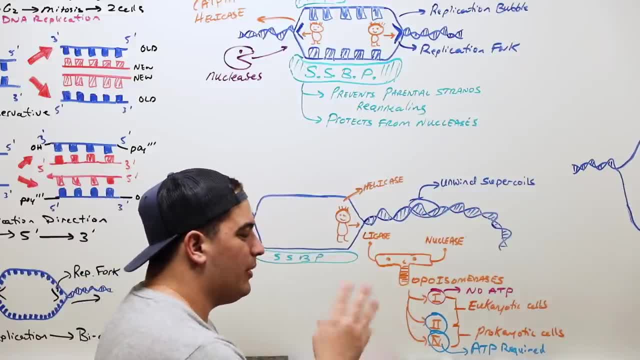 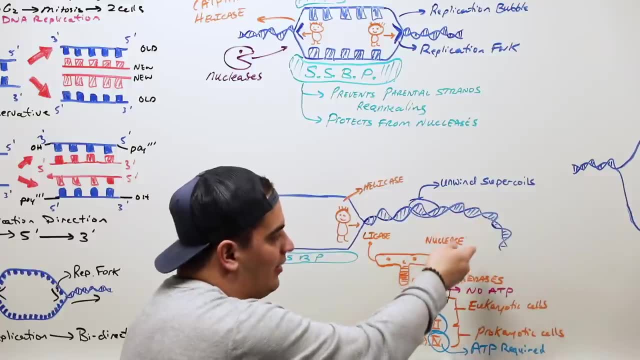 I don't wanna get too far in depth in it- that type two and four can do that are a little bit different from type one, and that's that. if you really look in the textbooks they can actually take and cut that little supercoil area. 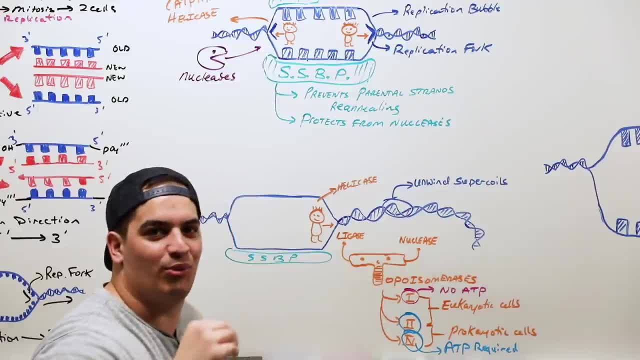 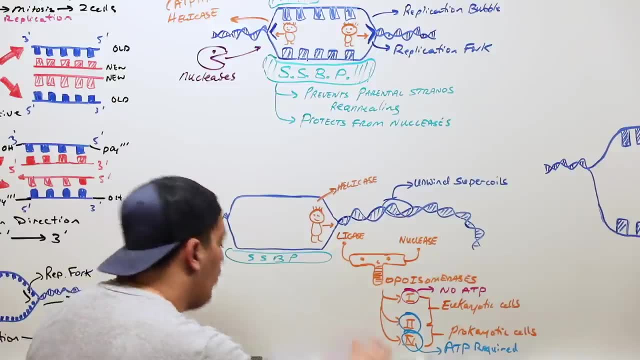 allow for it to unwind and then insert in what's called negative supercoils, which also helps to kind of relax the DNA and prevent that kind of bunching up region. But let's not get too far into depth in that What I really want you guys to know. 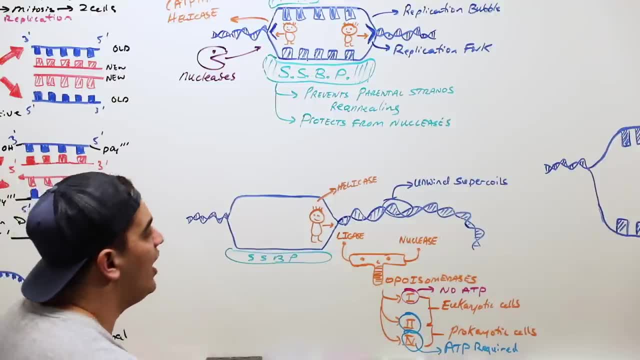 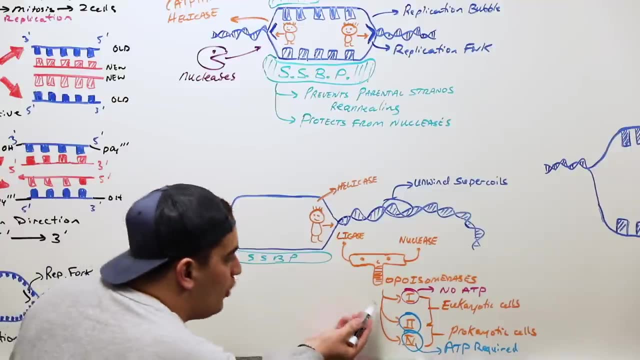 is why in the heck did I spend so much time talking about these topoisomerases In your USMLEs. you have to know particular drugs that we can target on these And eukaryotic cells. I want you to think about a reason. 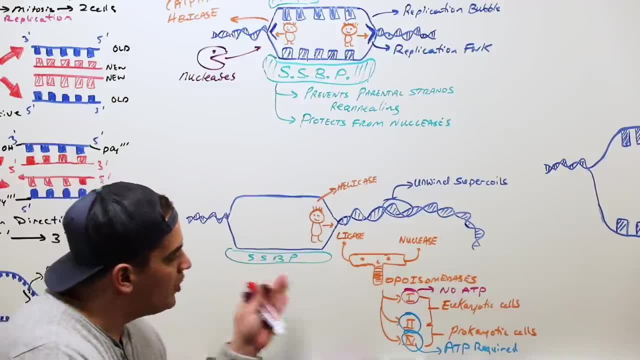 just try to think for a reason. Why would I want to target this enzyme in eukaryotic cells when this is important for DNA replication? Why would I want to target this enzyme in eukaryotic cells when this is important for DNA replication? 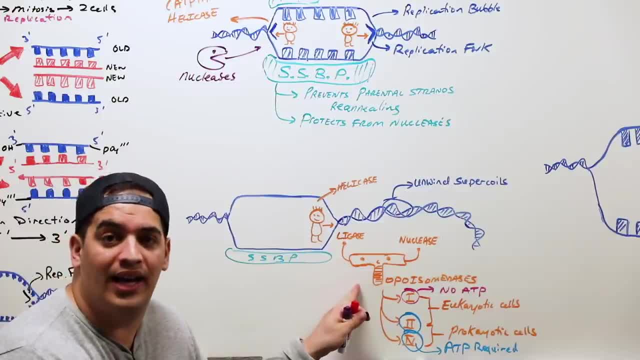 Why would I want to target this enzyme in eukaryotic cells when this is important for DNA replication? If these enzymes aren't really working, DNA replication won't occur Well in a eukaryotic cell. what if I have a cancer cell? 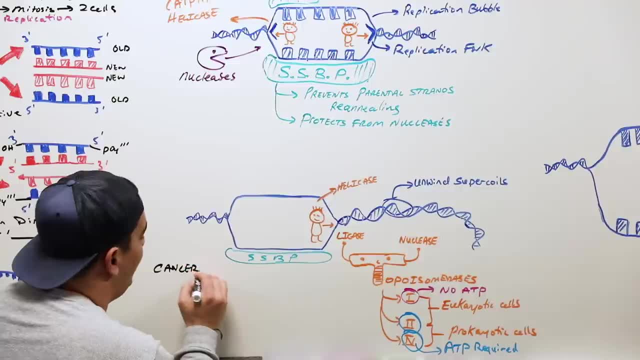 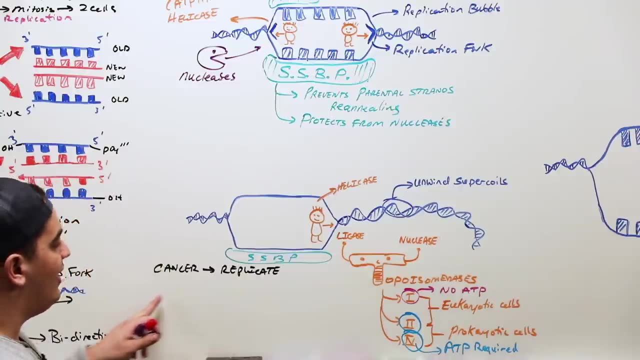 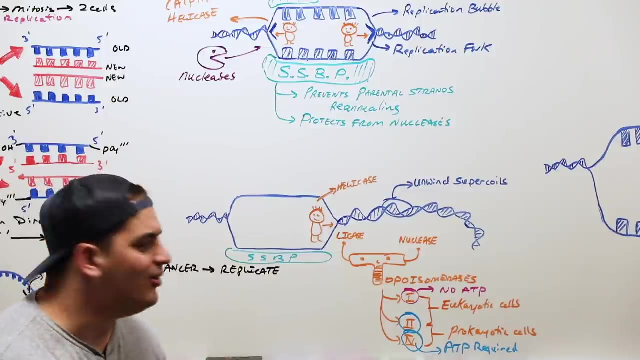 So if I have cancer, the cells will continue to replicate, So they'll replicate and replicate and replicate. Well, I could maybe use some drugs that could target these topoisomerases in my cancer cells and prevent them from replicating. How do I do that? 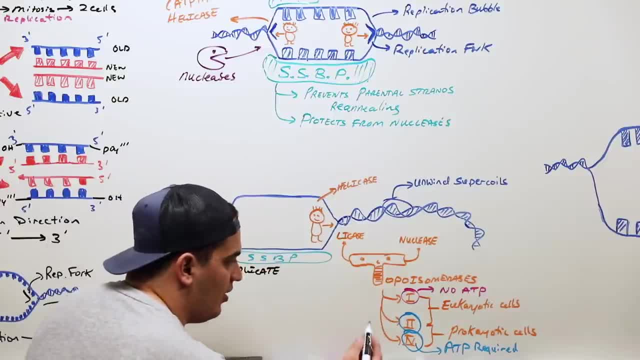 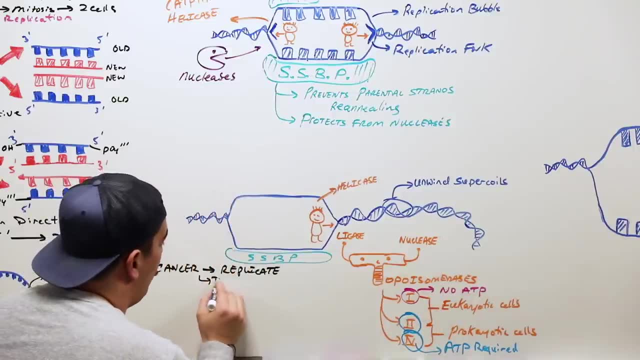 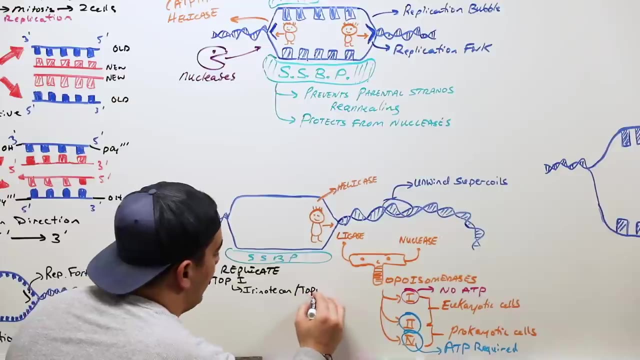 Well, there is a particular name of. there's a couple drugs that you guys definitely need to know For topoisomerase 1 in eukaryotic cells. the cancer drugs that we can use for topoisomerase 1 is called irenotekin and what's called topotekin. 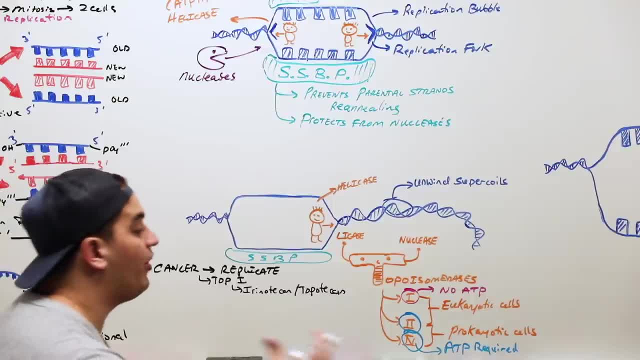 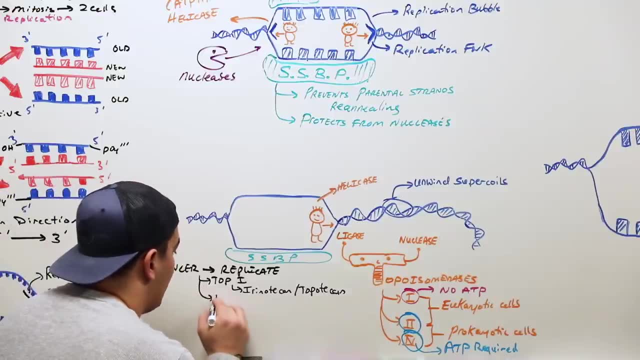 And again, these are anti, like they're chemotherapeutic drugs that are gonna inhibit the topoisomerase 1 in the cancer cells, The type 2 in eukaryotic cells. we can use drugs called the type 2 in eukaryotic cells. we can use drugs called 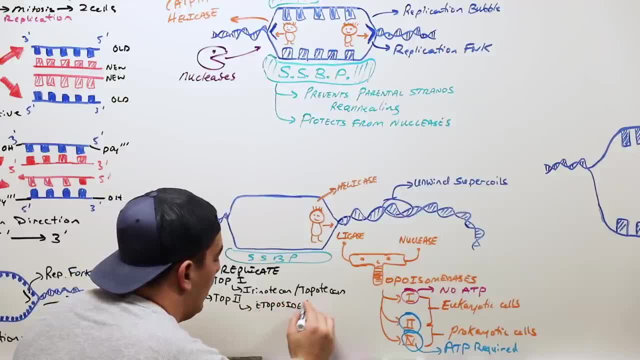 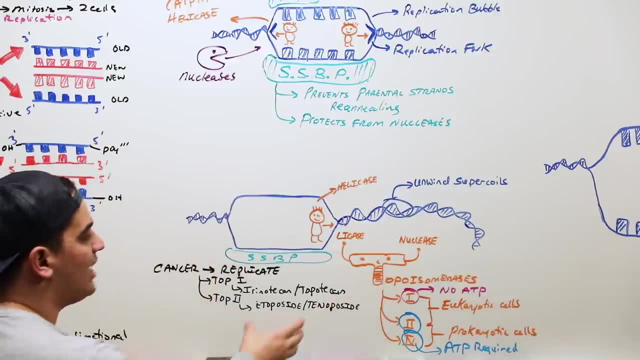 etoposide and tenoposide, And I'm gonna explain how they do that, because that's really important. I really want you to understand how they do this, But that's for the eukaryotic cells. Think about prokaryotic cells. 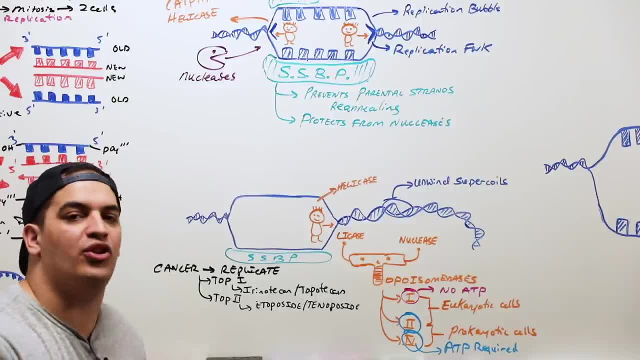 If you were infected by a bacteria and a bacteria infected your lungs and it just kept replicating and replicating within your lungs. could I maybe target the topoisomerase 2 and 4 and prevent that replication process of the bacteria in my lungs? 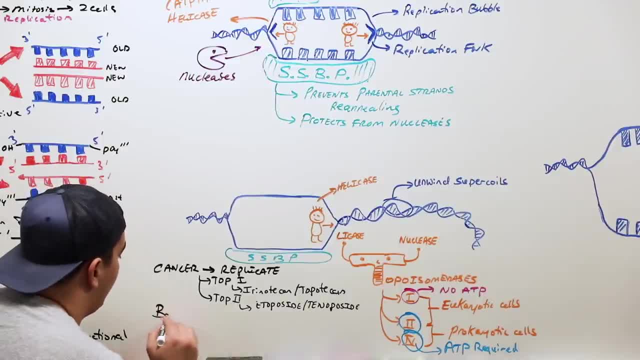 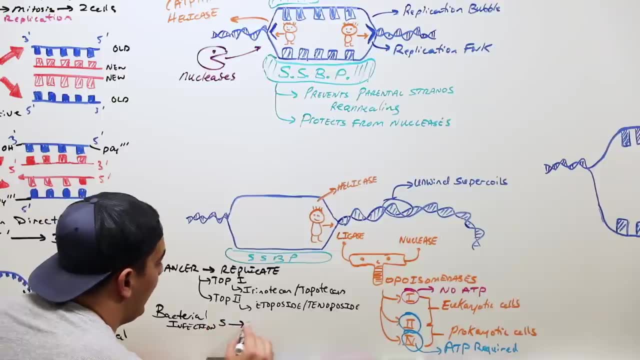 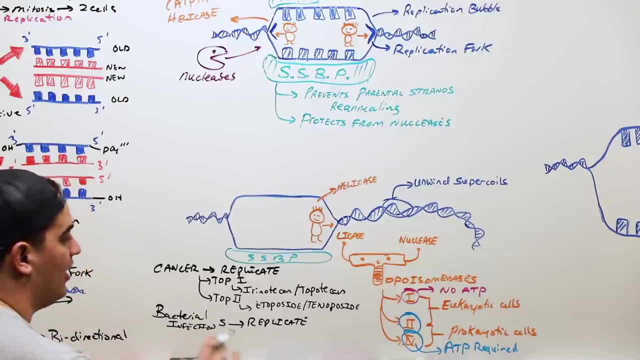 Yes, Bacterial infections, let's say, because it's a prokaryotic cell- and bacterial infections. these bacteria will continue to keep replicating. So if I use particular drugs that can maybe prevent the DNA from replicating in these bacterial cells, 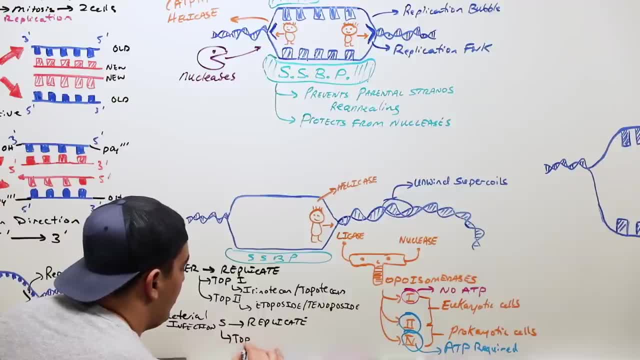 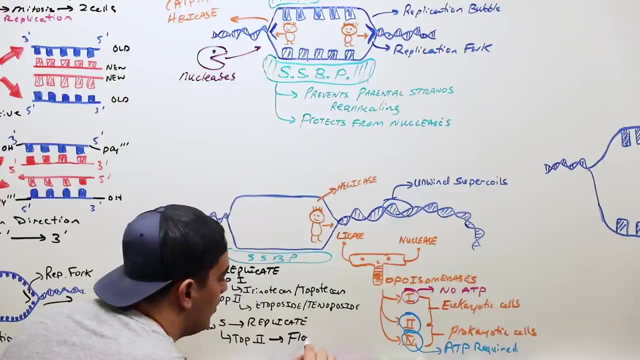 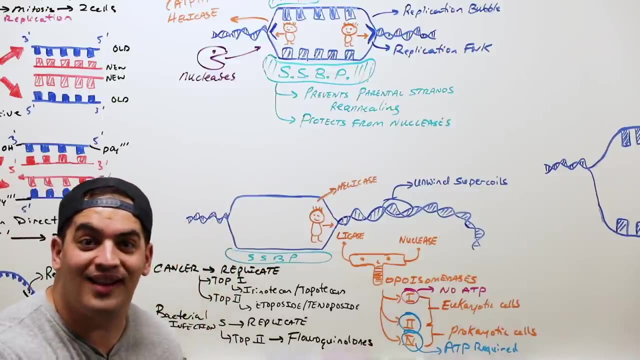 that's important And we can do that via inhibiting the topoisomerase, primarily type 2. And we use the drug called fluoroquinolones. Some of you may have heard of these: ciprofloxacin, levofloxacin, moxifloxacin. 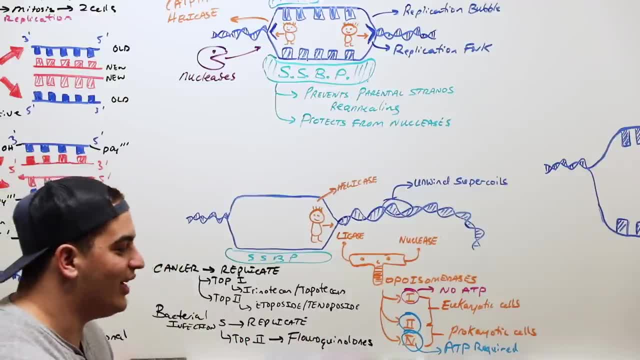 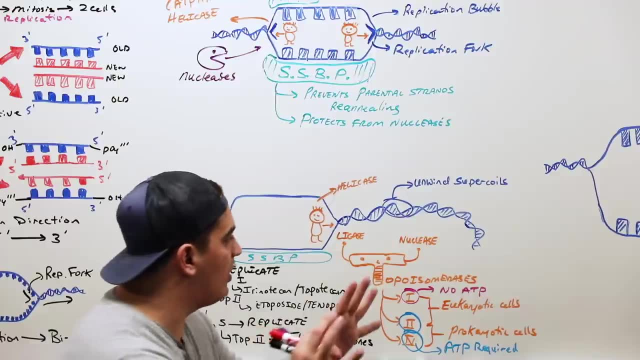 all of those guys. They're inhibiting the topoisomerase 2.. But I really want to take a second, because I never understood this completely until I really dug into the mechanism of how they actually do this. I really want to quickly say how they do it. 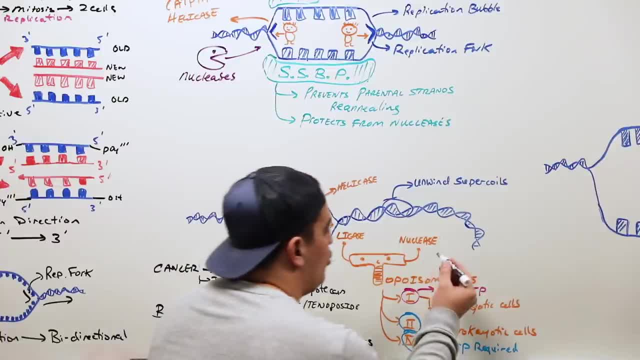 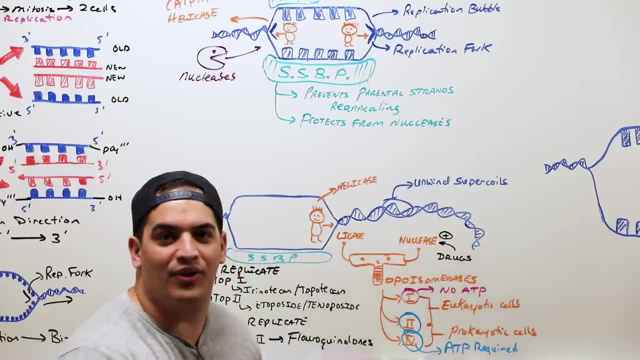 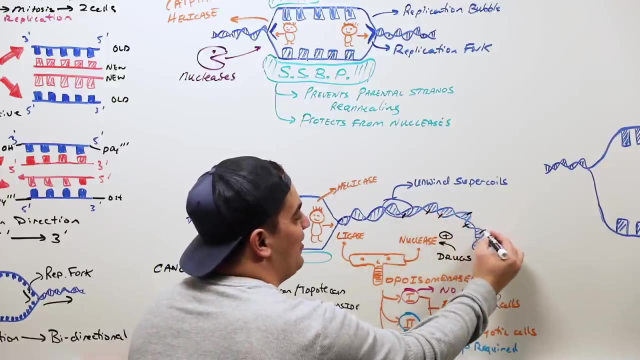 What these drugs are really doing is these drugs? so let's kind of just put here drugs. they're exciting and increasing the activity of the nucleus domain. What the heck is that going to do? That's going to just chop all those portions of the DNA. 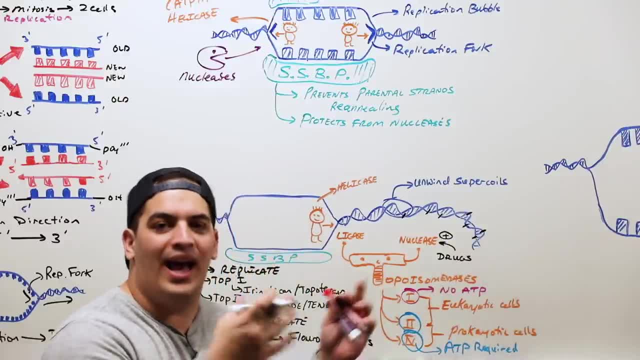 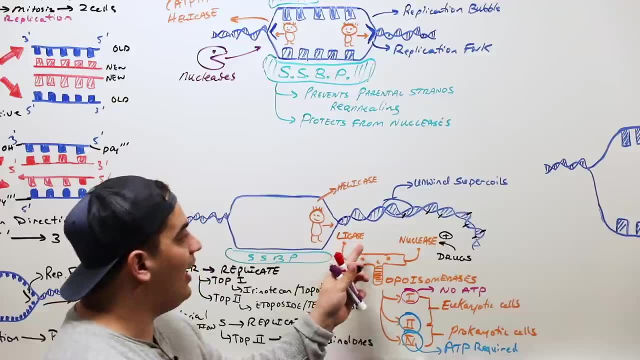 and it's going to continue to fragment them, right? Remember we had another domain of this enzyme that re-annealed them and kind of stitched it back together to prevent that fragmentation. That was the ligase binding domain. What if I use drugs to enhance the nucleus domain? 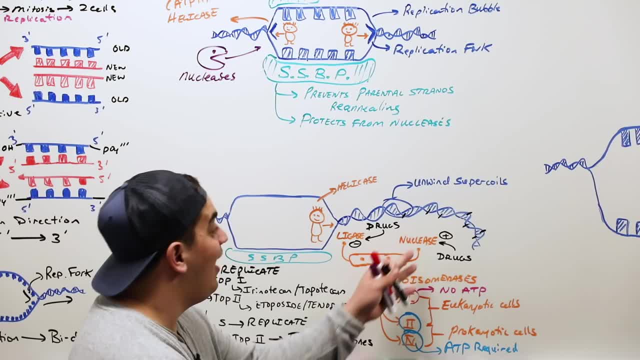 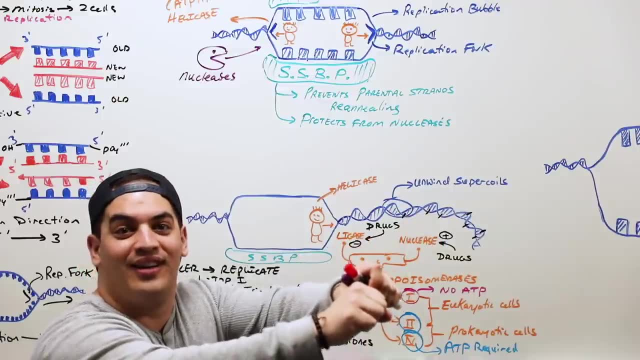 but inhibit the ligase domain. So now I'm going to have this enzyme go in and kind of cut where the supercoils is, but I'm never going to re-stitch it together. The DNA will just fragment over time, And that's important because then you can't replicate. 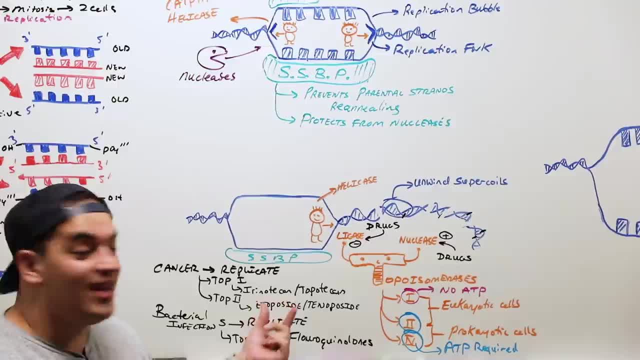 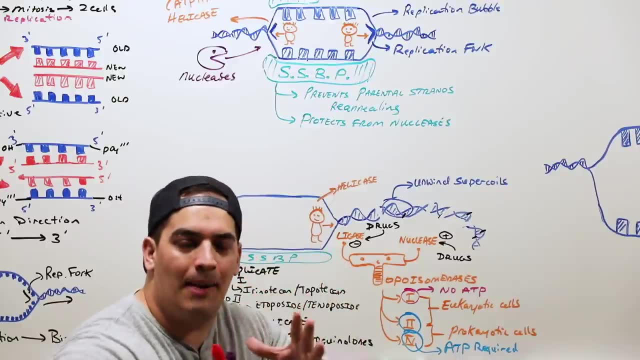 the DNA. within what kind of cells? Eukaryotic cells like cancer cells, or bacterial cells? And that's why those drugs are important. Doesn't that make sense? All right, cool. It's important to take a clinical application and tie it to the basic foundational science. 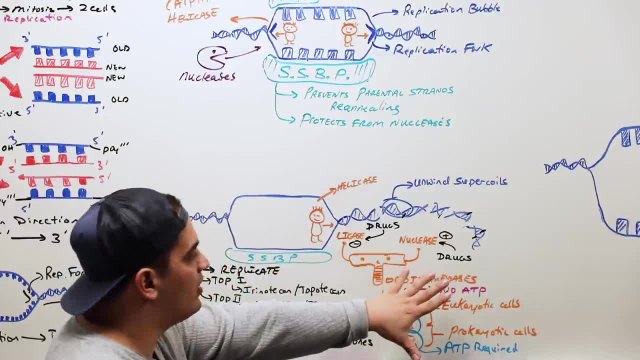 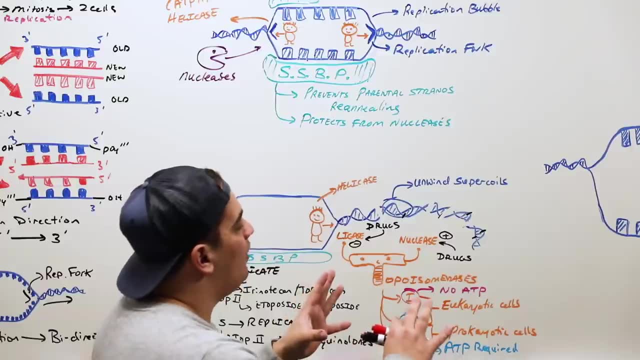 Okay, so we kind of went through, talked about the topoisomerases. the topoisomerases, that was the big thing, and how they unwind the supercoils. Let's get back to the foundational science. And now that we've talked about that, 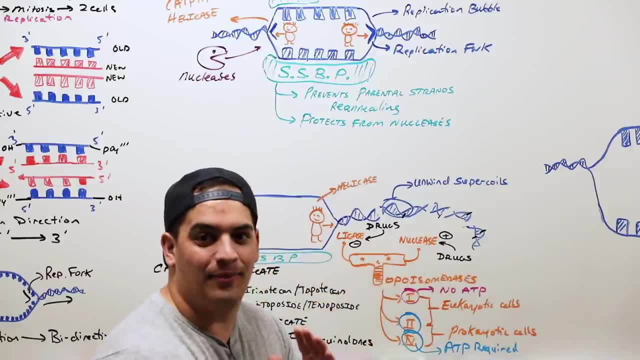 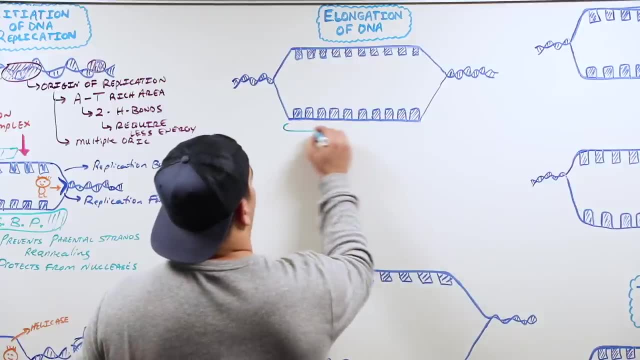 the next thing that we have to go into is elongating the DNA. All right, Ningenerds, so we already know. we have a replication bubble, We got our replication forks, We have our protein here, called the single-stranded binding protein. 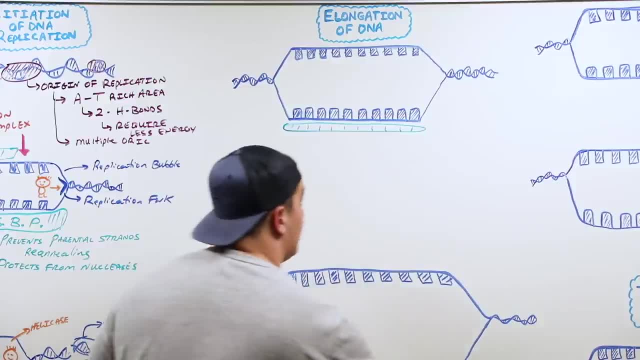 which is stabilizing these single strands. We have the helicase enzymes that are in these replication forks working like a son of a gun to unwind the DNA. We got those topoisomerase over here that are kind of unwinding those supercoils. 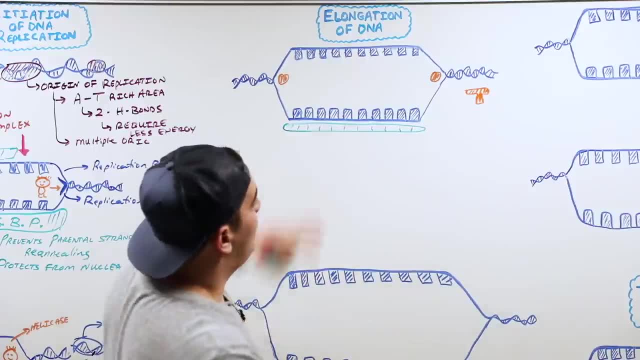 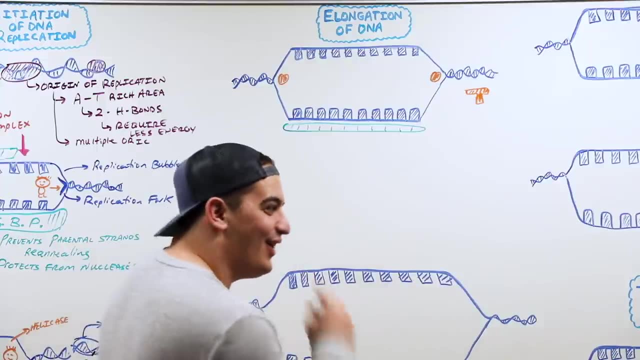 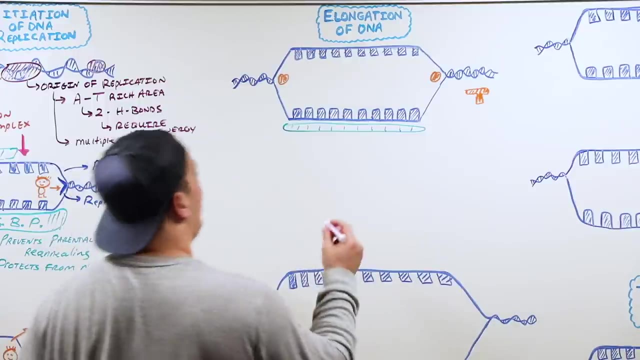 Okay, now we've really separated this, we've stabilized it and we're ready to begin elongating the DNA. Okay, here's what's really interesting. There's an enzyme that comes into play here and it does something really cool. It's called primase. 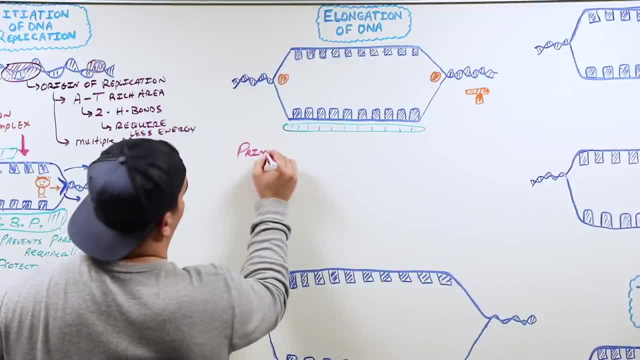 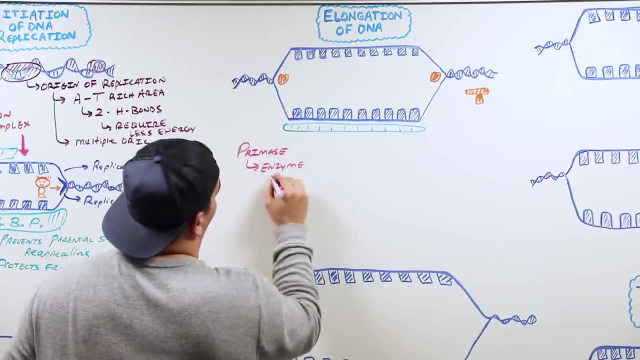 So an enzyme called primase will come into play here. So what primase does is it's an enzyme that's called primase. So what primase does is it's an enzyme that's called primase. So what primase does is it's an enzyme that lays down. 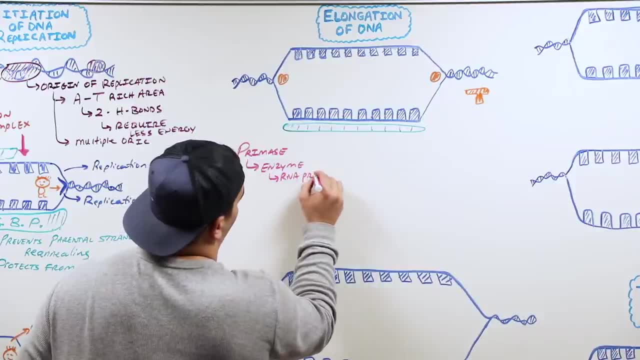 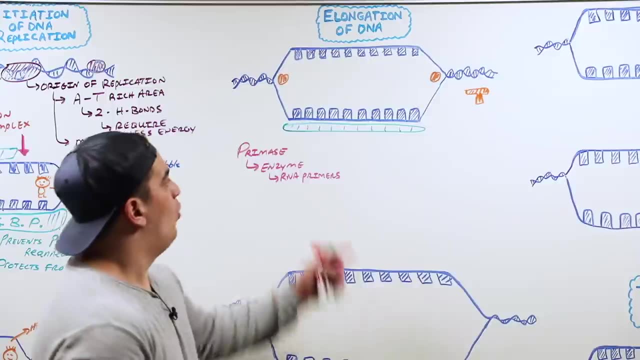 okay, that makes what's called RNA primers. So this takes a really quick turn where we gotta understand. Zach, you just said that we're making DNA. Why the heck would I make RNA? There's a reason why. There's an enzyme that we'll talk about a little bit later. 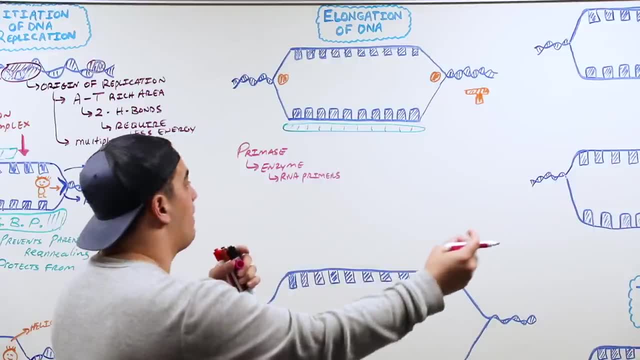 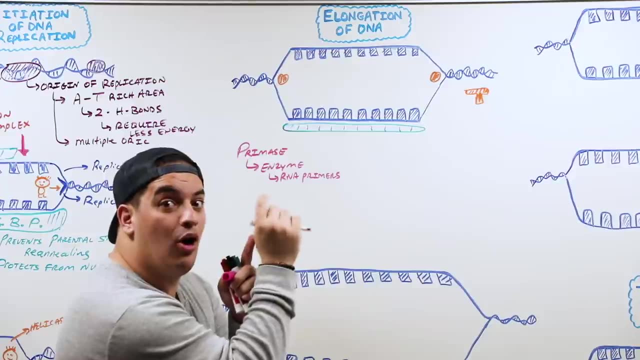 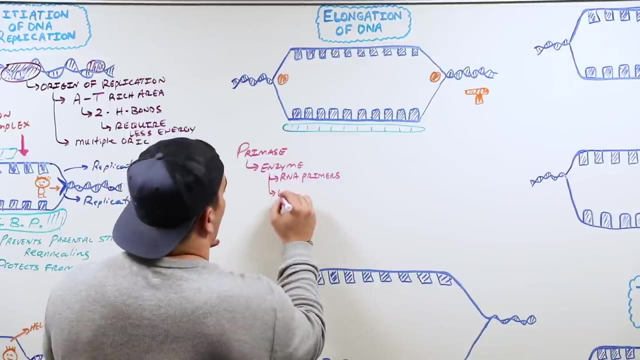 called DNA polymerase III. that will make DNA, But the only way it can do that is if it has some type of primer or a three prime OHN to build off of. So what's the purpose of this primase, this enzyme? It lays down RNA primers which enable 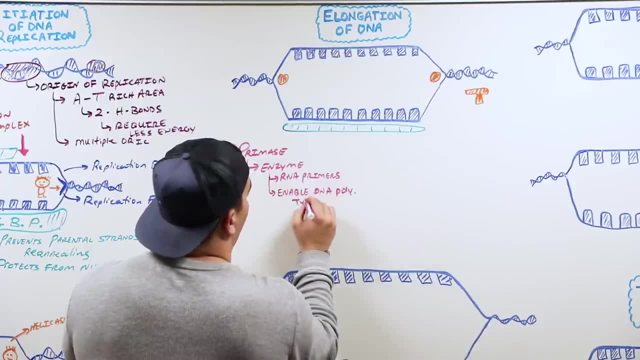 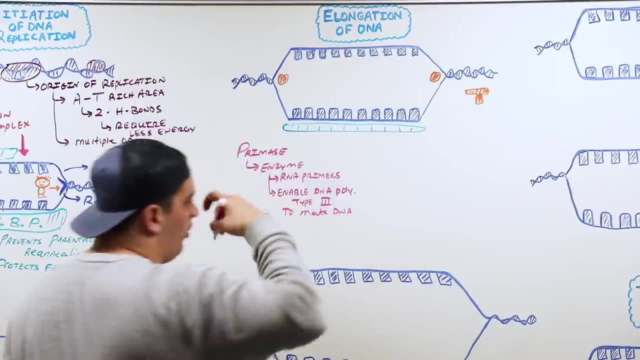 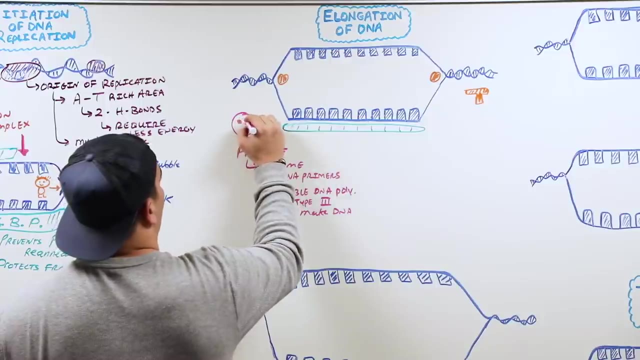 DNA polymerase, particularly type III, to make DNA, And I'll kind of show you that in a little bit, in a second. So primase comes in. So imagine, here I just have this cute little enzyme here called primase. Okay, 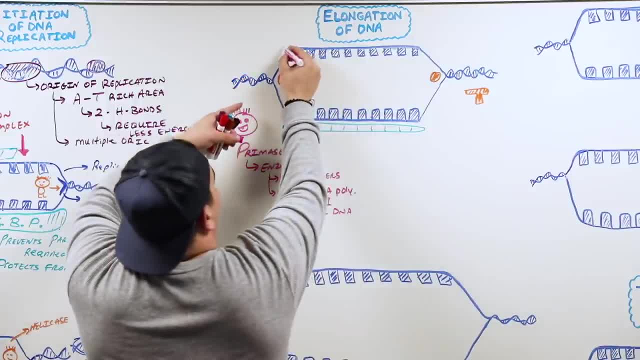 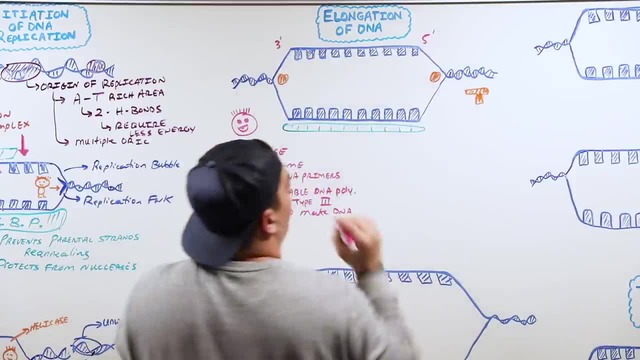 And this cute enzyme comes in here And let's say here, what's this strand up here, This top part? Remember we're gonna say that this is three prime end where the OH would be. This is the five prime end where the phosphate would be. 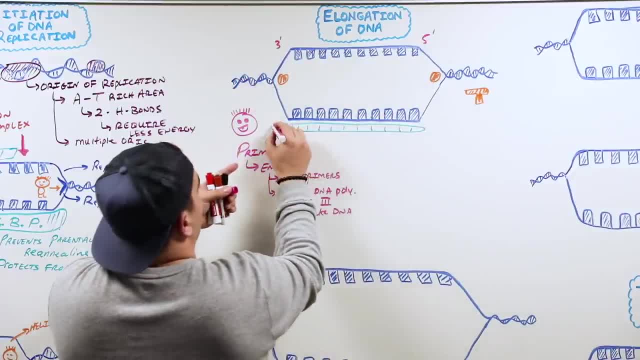 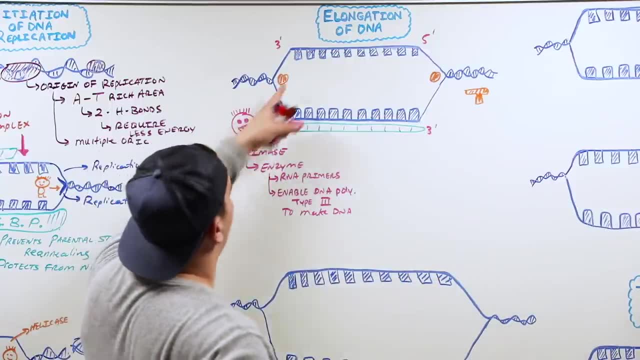 And again the opposite strand here would have to be anti-parallel. So five prime end here. three prime end here. Right, we already know that The primase is gonna come in and it's gonna read the nucleotides and it has to go in a particular fashion. 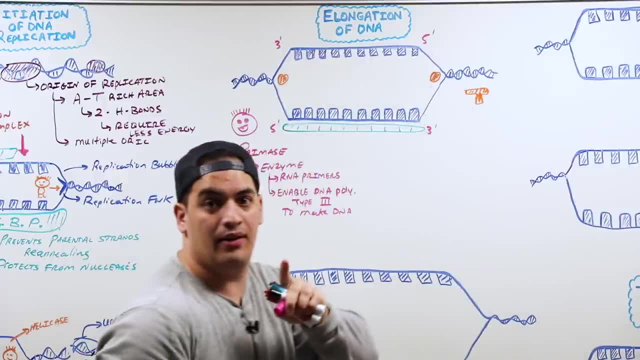 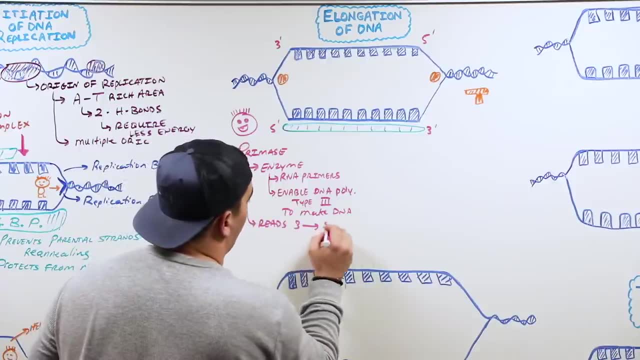 It reads it from the three all the way to the five end. So what does it do? The first thing it does is it reads the DNA strand from three to five. After it reads it from three to five, what did I tell you? that's super important. 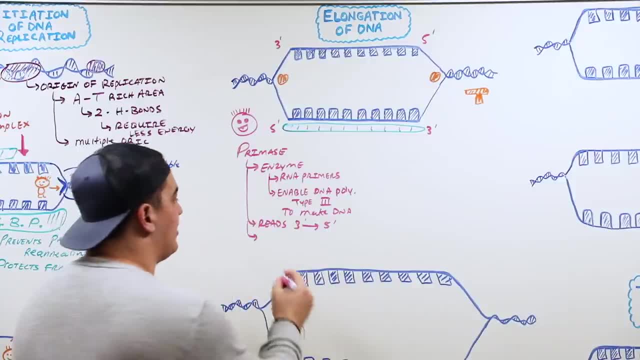 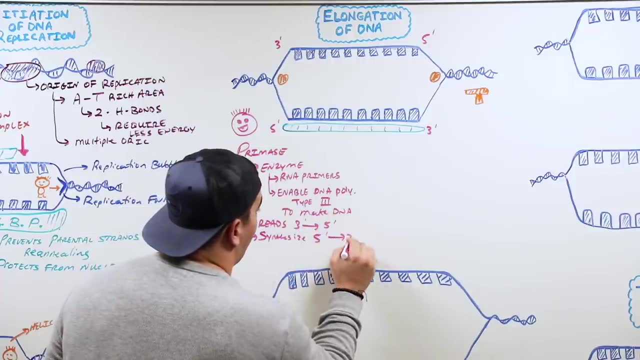 What does DNA replication occur? Even though this isn't DNA, it's the same concept. It synthesizes RNA primers or nucleotides, in a five to three fashion, So it's gonna take and make a couple nucleotides. Generally it's about 10 nucleotides. 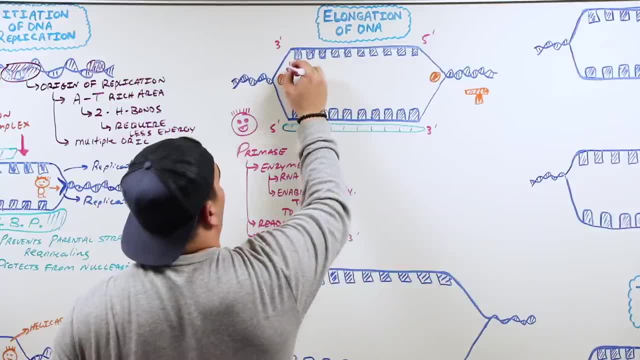 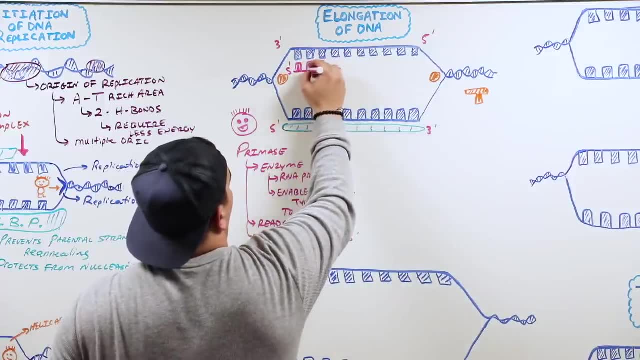 We're only gonna draw a couple here, But it'll have. it has to be again five prime starting here, And I'm just gonna make a couple. I'll make like four nucleotides here, Okay. so here it's gonna have five. 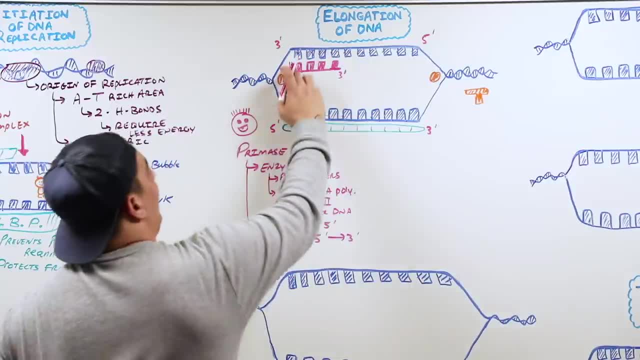 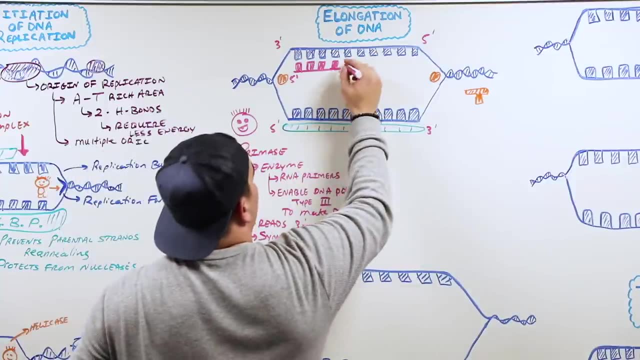 all the way to the three prime end here. okay, That's my five prime end here that I just started with, and I'm synthesizing it in the three direction. Now, the reason why this is important is on that three end. what do we have here? 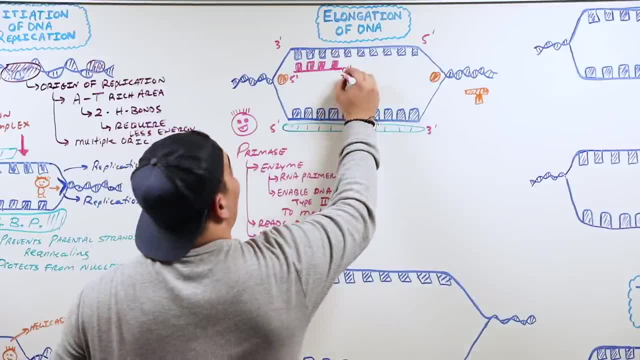 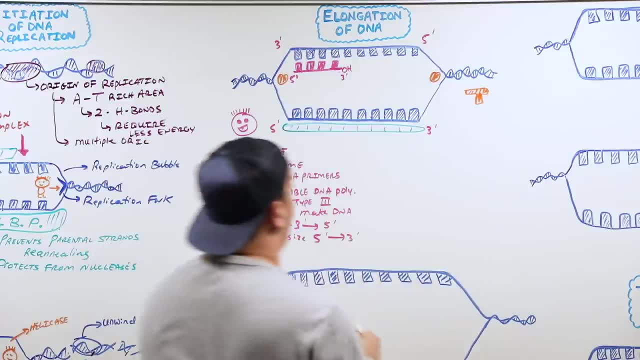 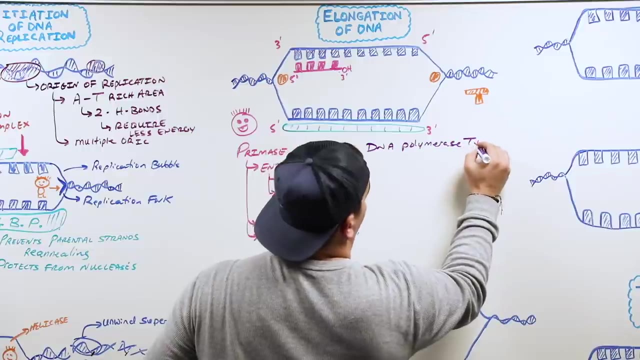 The OH. That's what's on the three prime end. I need that OH. The reason why is another enzyme called DNA polymerase type three comes in. So there's an enzyme called DNA polymerase type three And he comes in and he needs that three prime OH. 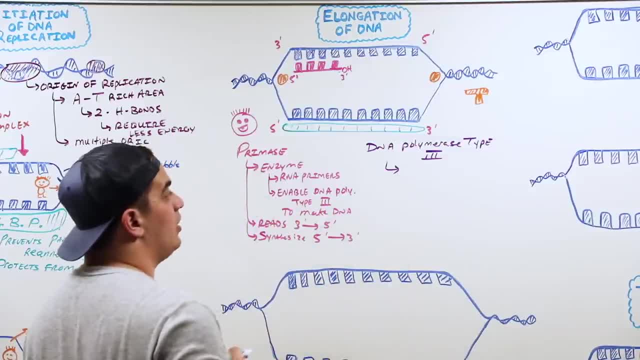 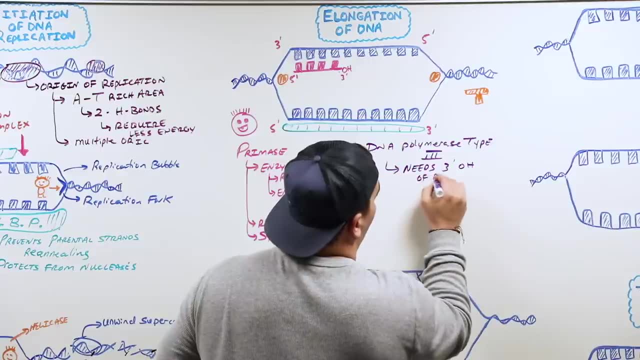 from the RNA primers in order for it to continue to build nucleotides. So again, a big thing I need you to remember is it needs the three prime OH of RNA primer in order to carry out its activity. If it doesn't have it, it can't do it. 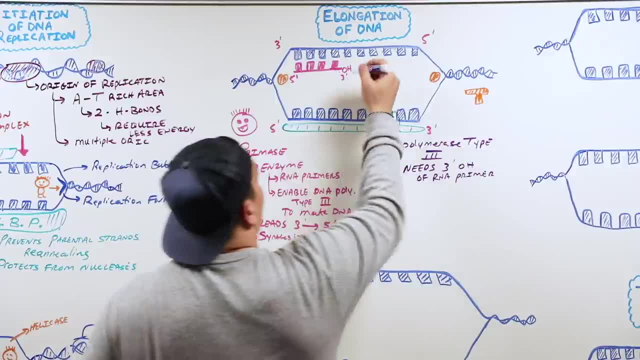 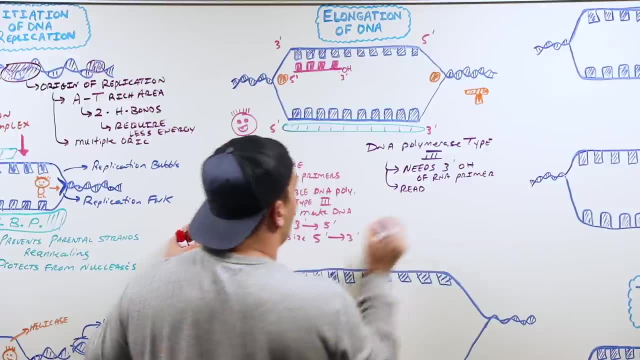 So now that it has that, this DNA polymerase comes in and it says, okay, I have my three prime OH region, Perfect. Now what I'm gonna do is I'm gonna read my DNA and I'm gonna do it the same way that the primase did. 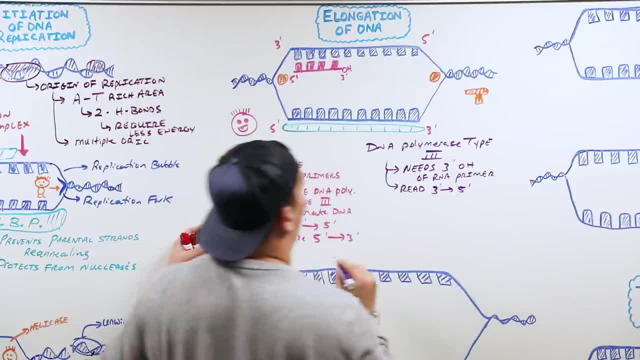 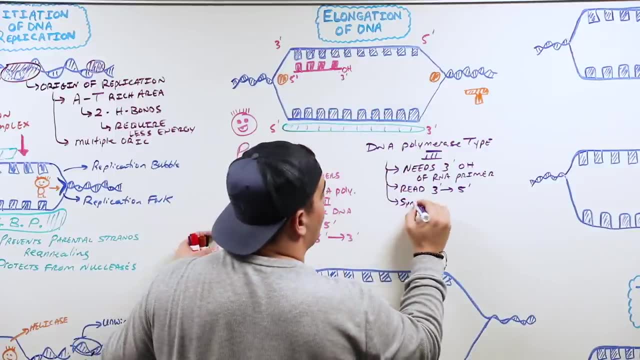 I'm gonna read the DNA from the three direction to the five direction. So I'll read it: Boom, boom boom, Boom, boom boom. Once I read and figure out what kind of nucleotide is, then I'm just gonna synthesize those nucleotides. 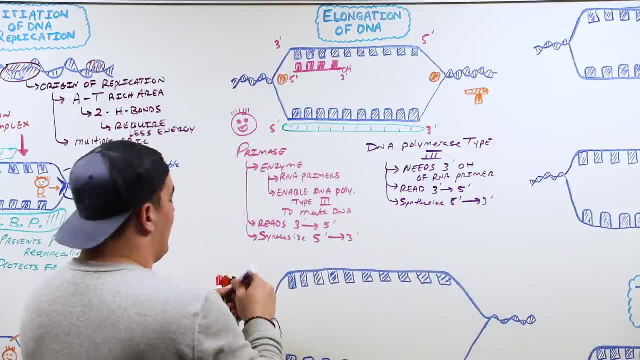 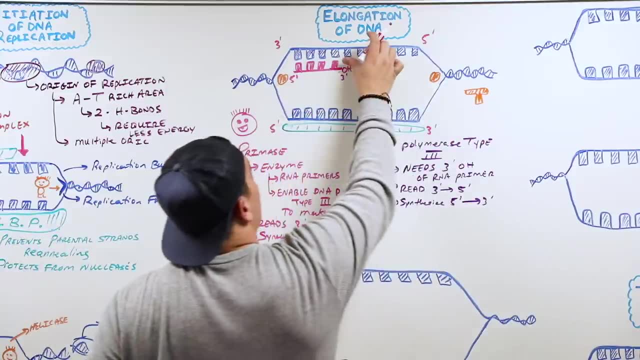 in the five to three direction, And it's the same process here. So now let's make a different color, since it's a different enzyme. We kind of picked red over there. So we're gonna start off and we're gonna say okay. 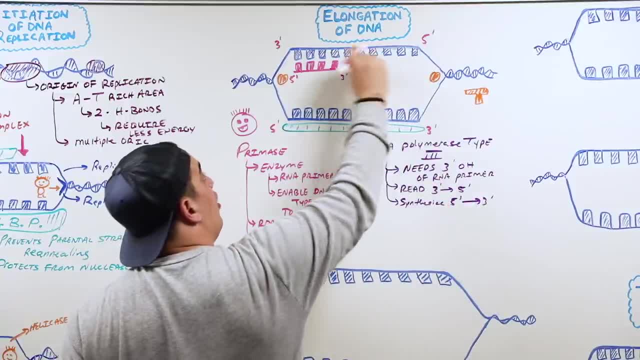 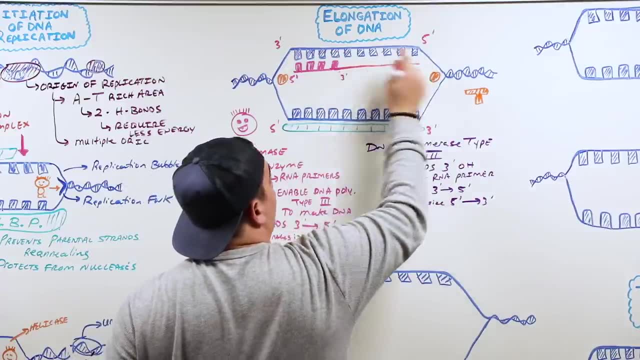 I'm gonna take that OH and I'm gonna add a phosphate group onto it of another nucleotide. So when I do that I'm gonna continue to keep synthesizing and a five to three direction moving towards the replication fork. Again, when I do that, I read it: 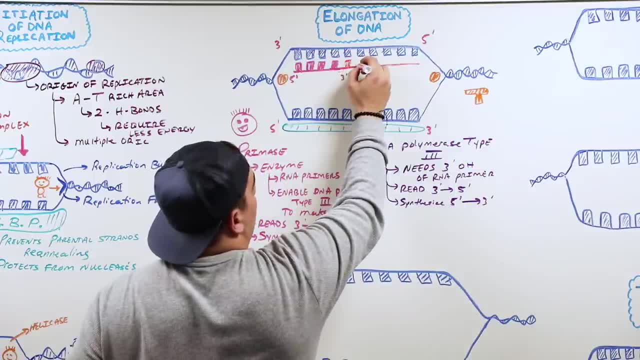 I say, okay, let's say that this is adenine, I'll put a thymine, This is guanine, I'll put a cytosine, This is cytosine, I'll put a guanine, And so on and so forth. 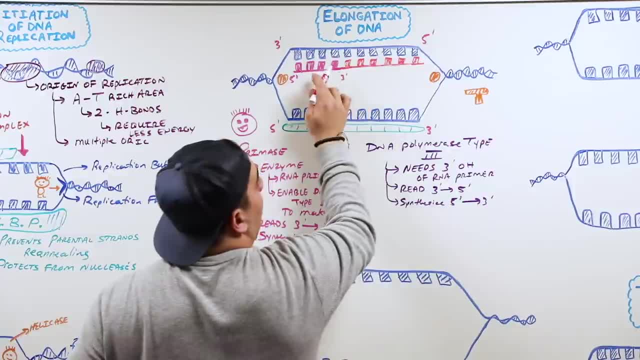 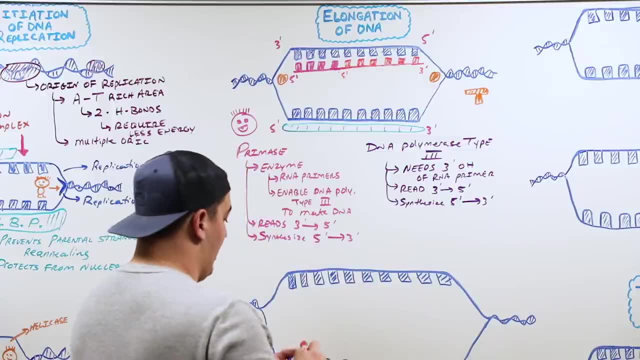 And I'll just keep reading the nucleotides, three to five, and making a DNA strand. in what direction? Five to three, Okay, And again, important to remember, it needed this three prime and of that OH, of the RNA primer, to build off of it. 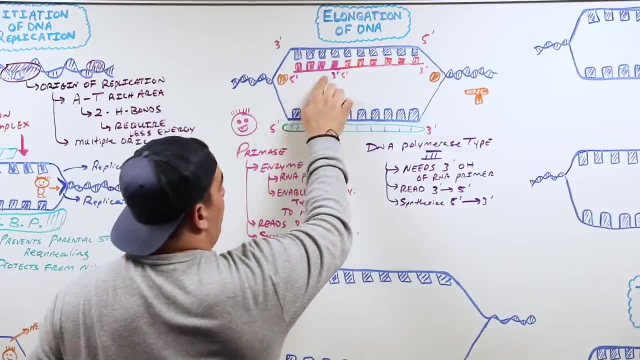 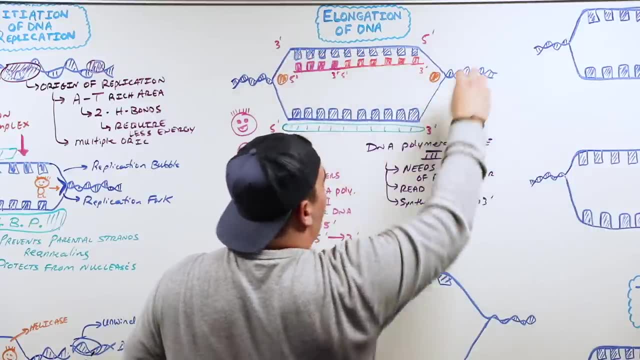 Now here's what's really interesting. The primase will give it kind of a little leading point and the DNA polymerase will just go all the way towards the replication fork. This strand is very continuous, where there's just one RNA primer and then DNA the rest of the way. 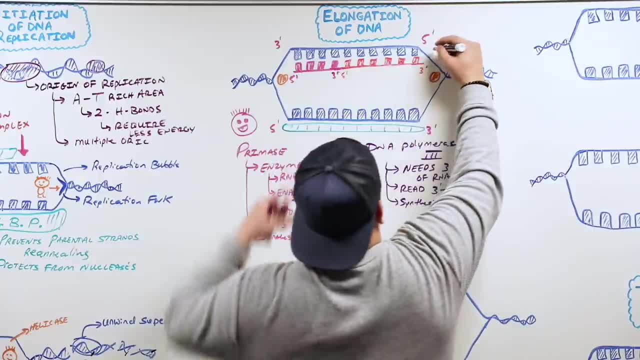 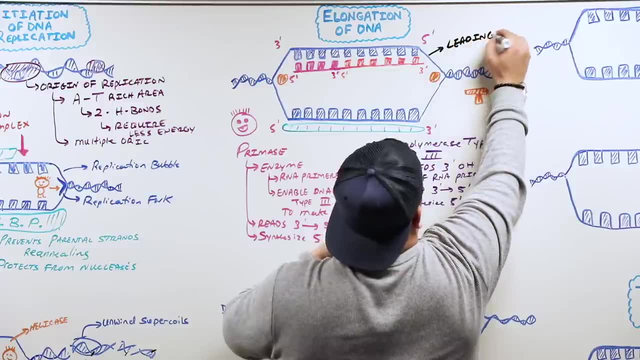 This strand is very important. We give it a particular name. The strand is very continuous. where the DNA polymerase moves towards the replication fork is called the leading strand. Okay, It's called the leading strand On this other strand which we're gonna talk about. 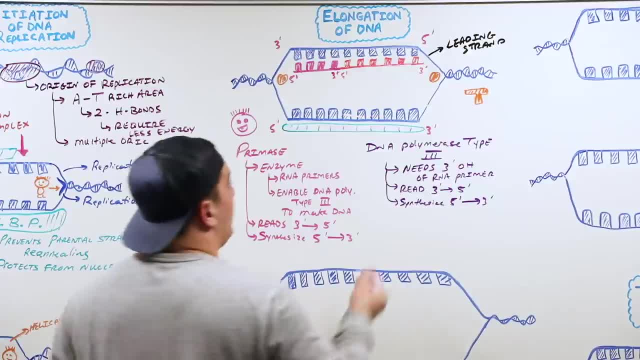 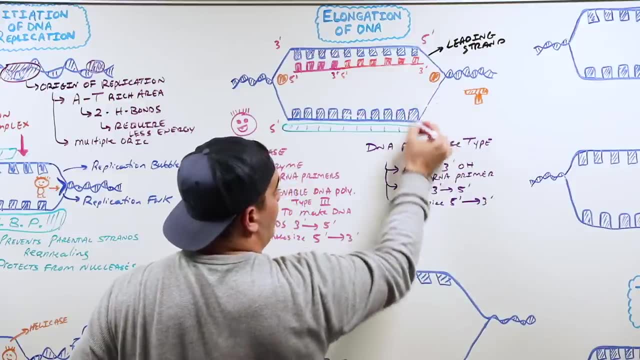 it's called the lagging strand. Something different happens. Where you're still gonna have the primase, it'll come to this area. okay, on this other strand. And again, this is the three. end on this part. five end on this part. 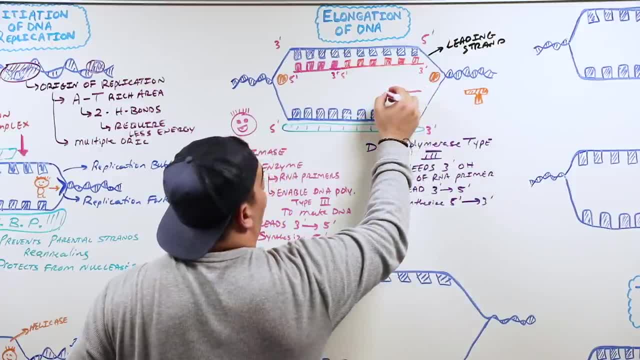 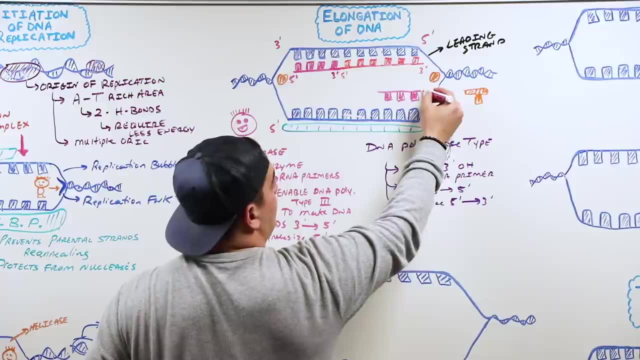 And what it'll do is it'll read it from three to five and then synthesize a couple nucleotides from five to three. So this is the three end. It's gonna synthesize from five to three And again the same thing will happen. 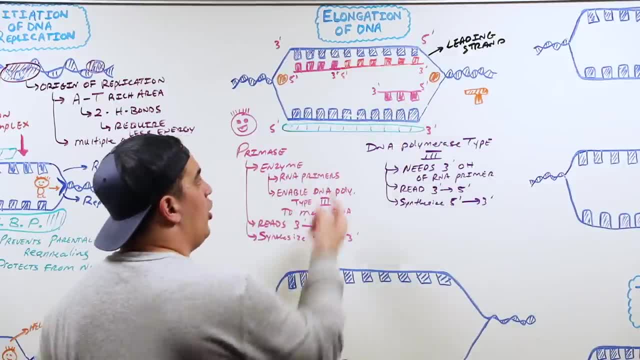 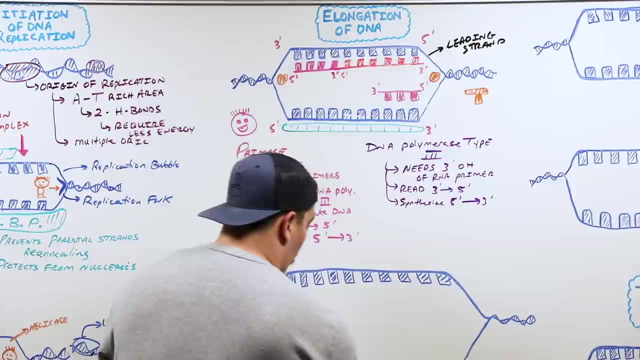 We created a primer of a couple nucleotides with a three prime OH end that the DNA polymerase type three can build off of. So now the DNA polymerase type three will just pop on say: oh perfect, I have my three prime end to use. 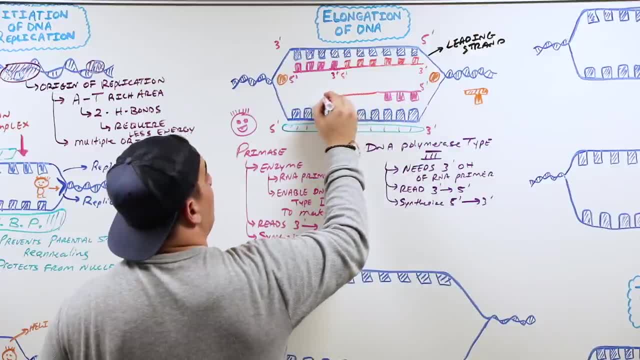 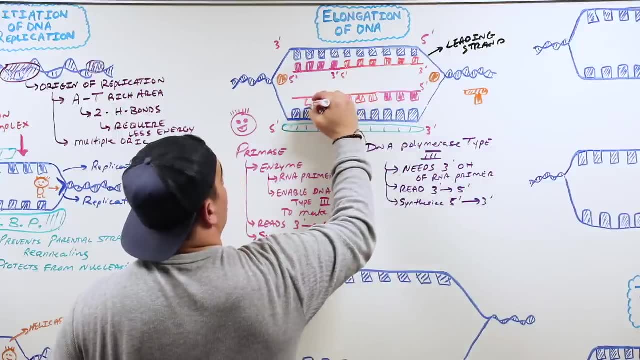 I'm gonna go ahead and just read the DNA from three to five and synthesize it from five to three. Okay, so I'm gonna do all that perfectly. Now something interesting happens. Where it's gonna look, it looks perfectly the same. 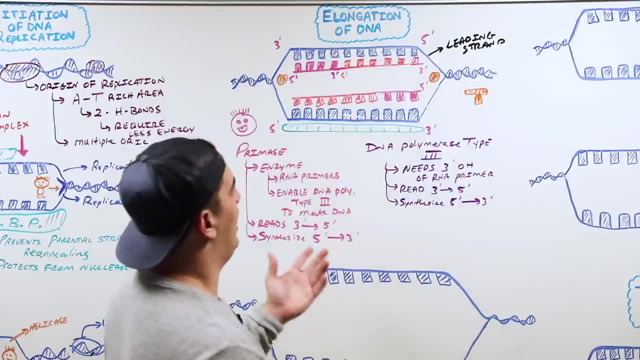 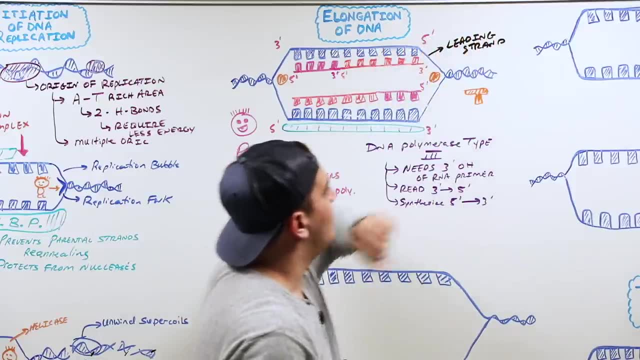 You're like Zach, I don't get the difference here. Let's say that the helicase continues to unwind the DNA, So it continues to unwind the DNA. Something interesting happens that we have to talk about. Okay, so now let's come down here. 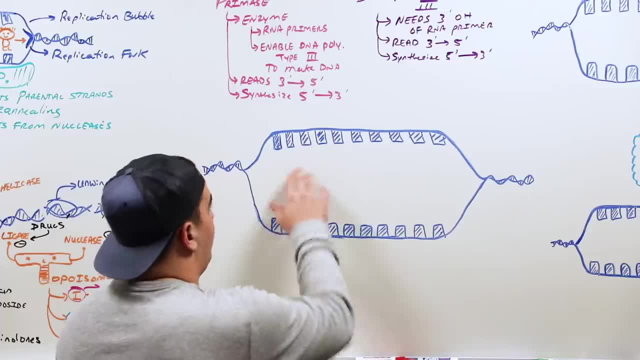 So let's say, let's pretend, right, that for a second here we have that primer. Let's kind of continue off of this. Let's say that the helicase unwound down here, Okay, so now we're gonna do that. 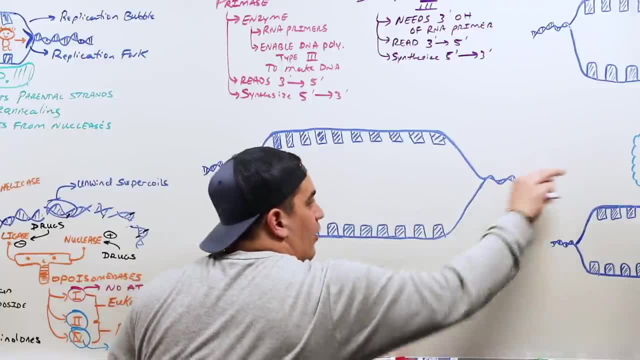 Okay. so now let's come down here. Let's try to unwind the DNA a little bit more, And we kind of opened up the DNA and created a more longer length of nucleotides. So again let's say that here we had that primase. 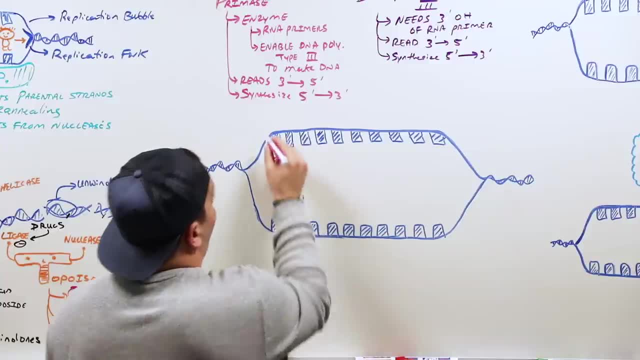 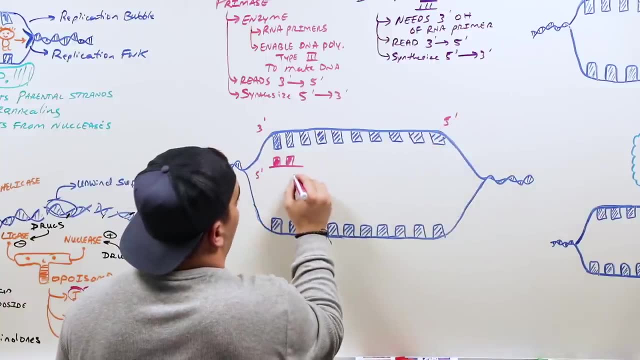 came in here. read this: from what end? Again, this would be your three prime end. This would be your five prime end. So it'll read from three to five and synthesize from five to three. Creates a little primer with a three prime OH end. 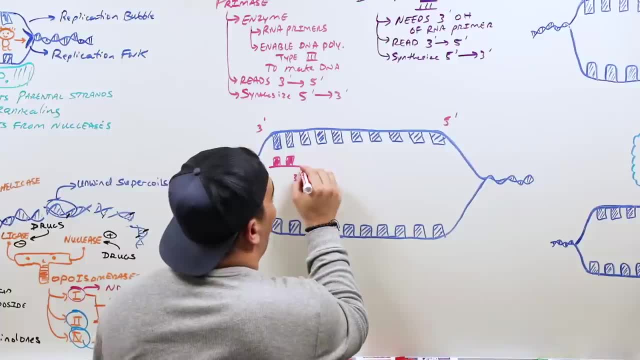 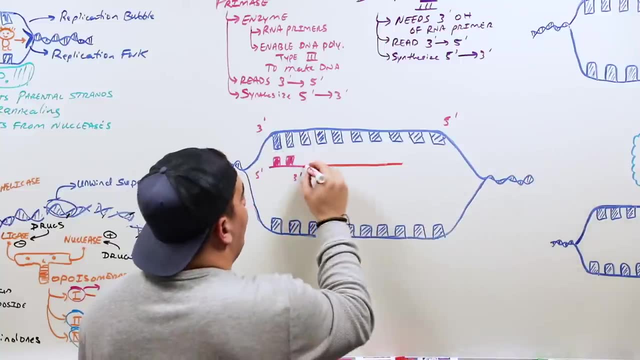 The DNA polymerase III says, okay, perfect, I have everything I need, I can continue to grow, And let's say that again. it just came up to like this point here. But then you kind of unwound the DNA again. 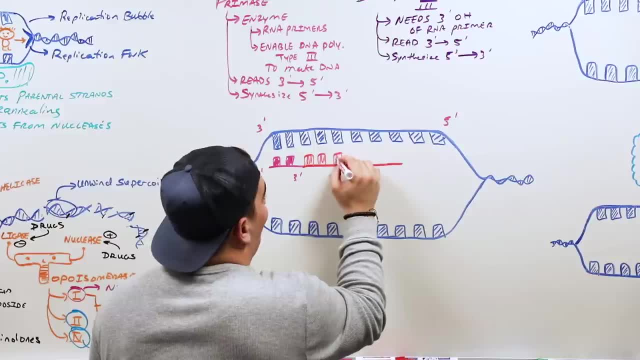 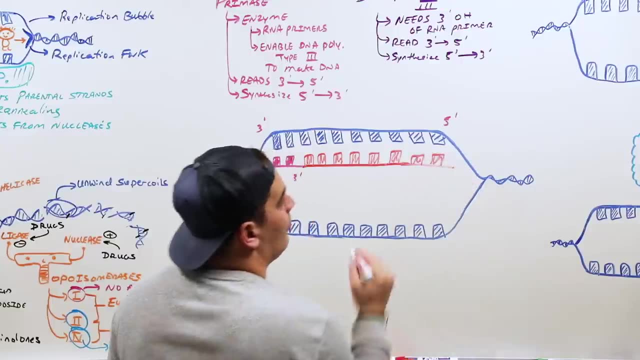 That DNA polymerase three doesn't stop. it just keeps on going and keeps on moving, reading the DNA from three to five and continuously synthesizing nucleotides from five to three. So again, this would be your five prime end. this would be your three prime end. 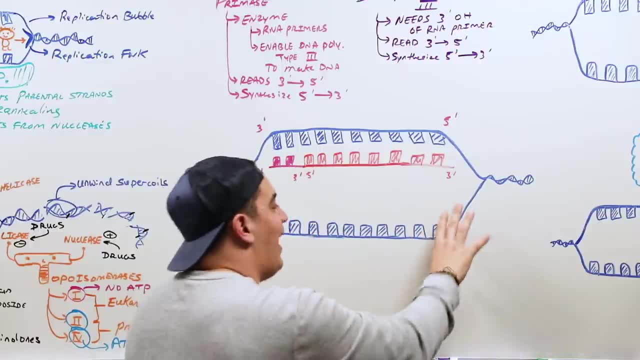 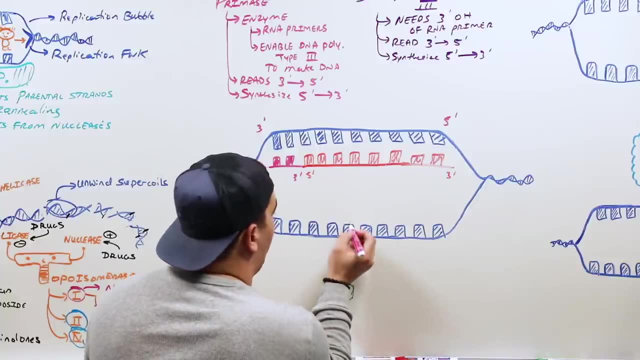 On this other strain. this is on the leading strain. it continues On the lagging strain. here's where it's a little bit different. Let's say that we continue to move on here And let's say that at this point here. 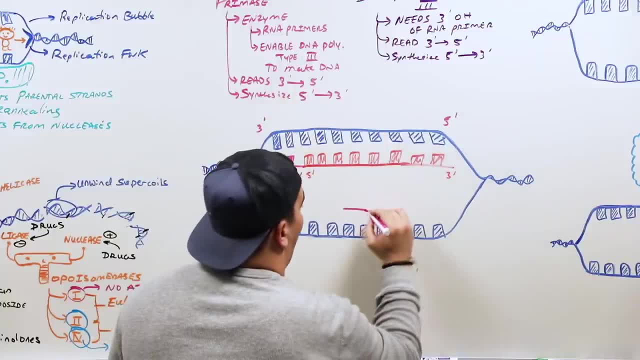 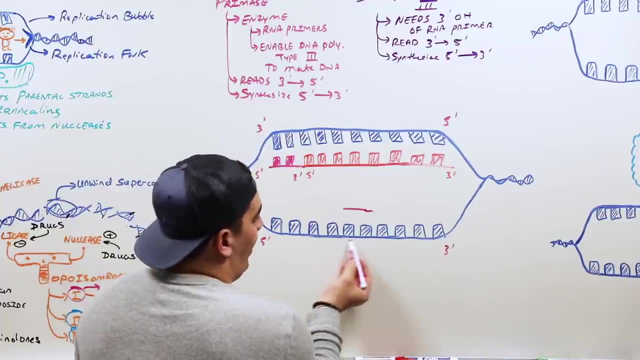 this was where the previous RNA primer was from above, where it had again reading this portion of the DNA. this is the five prime end of this part. three prime end of this part. It read this sequence of DNA from three to five. 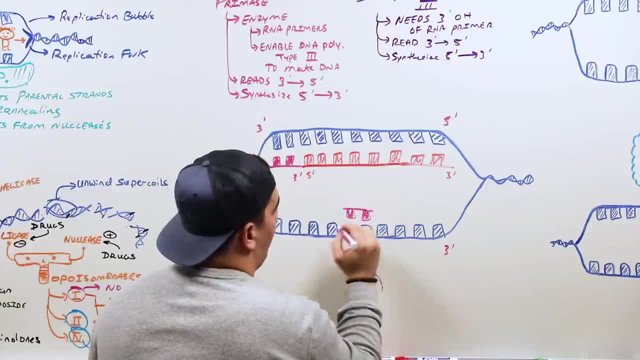 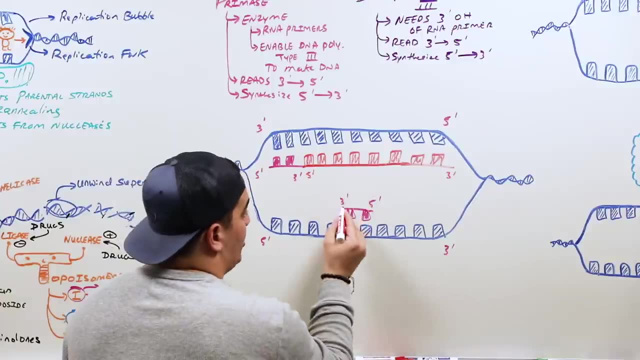 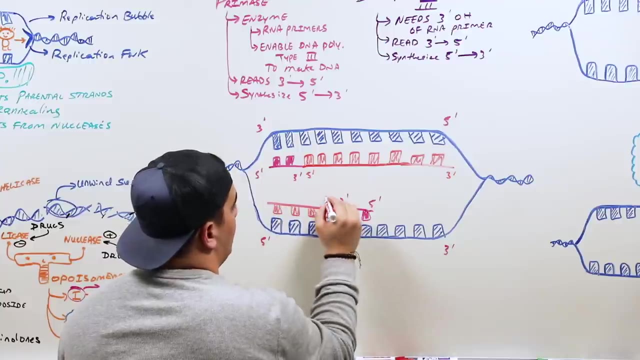 and let's say that it synthesized a couple nucleotides to give you your RNA primer from five to three. And then what do we say happened? from that part above We had the DNA polymerase three. use that three prime OH end to read the DNA from three to five and synthesize the nucleotides. 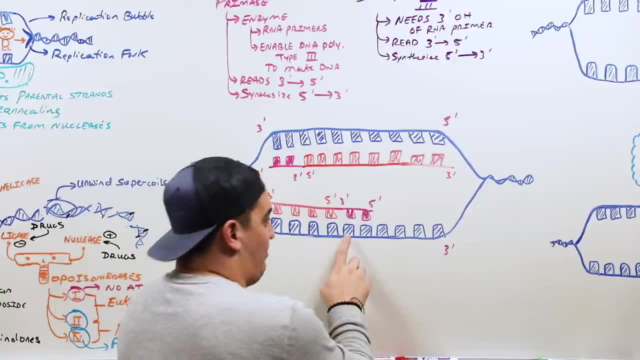 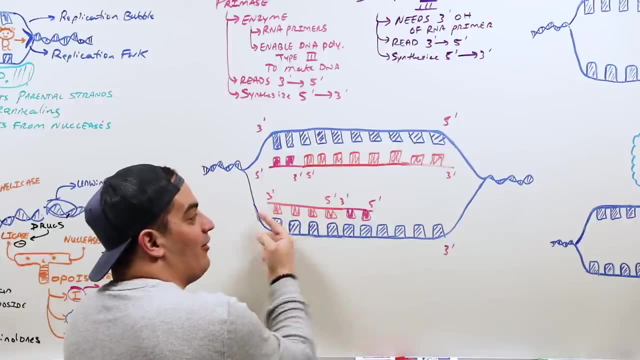 from five to three. Here's what happens. The primase laid down a primer here, but the DNA polymerase three has to use that primer to continue to keep building off. If you unwind the DNA a little bit more now, now you have a couple other nucleotides. 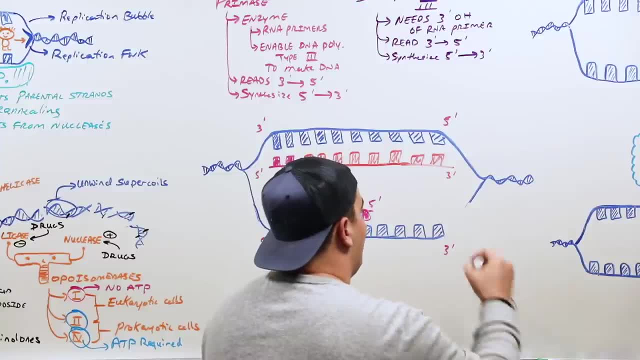 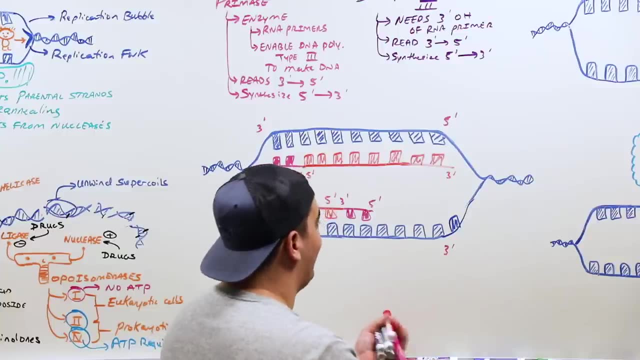 So now let me kind of just so we have enough room here, Let's say I draw a couple more nucleotides. So now here I have a couple more nucleotides, Now that primase, after it just made down this primer for the DNA polymerase three to use. 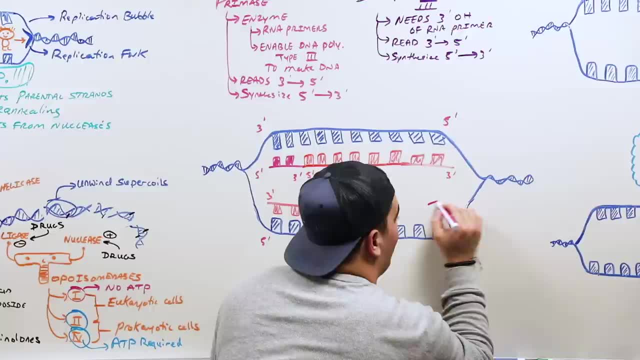 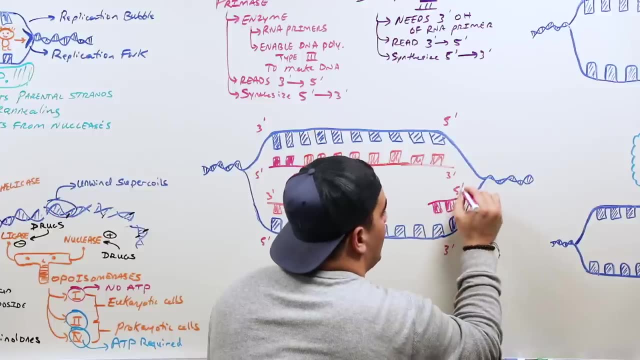 it comes down to the next part of the replication fork And it says: okay, here I got another three prime end here. Let me again read from three to five and synthesize a couple nucleotides from five to three. So I laid down my RNA primer. 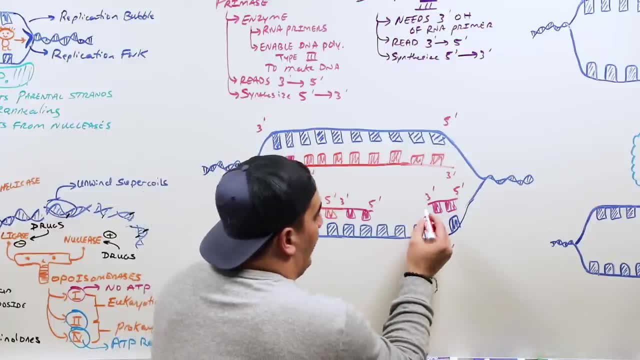 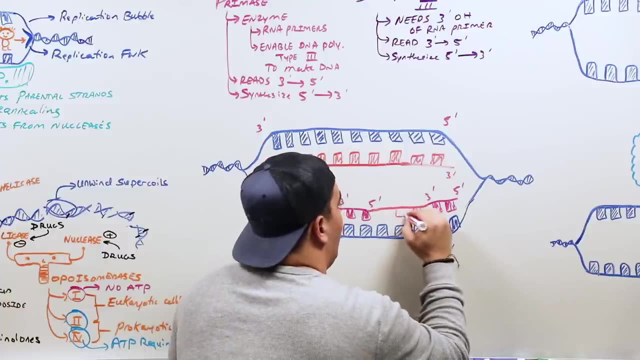 DNA polymerase says: oh okay, cool, I got my three prime OH. end here. Let me go ahead and use that to make my DNA And I'm gonna read the DNA. I'm gonna read the DNA from three to five and synthesize it from five to three. 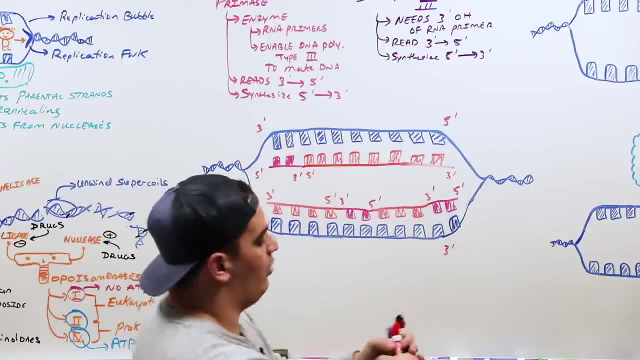 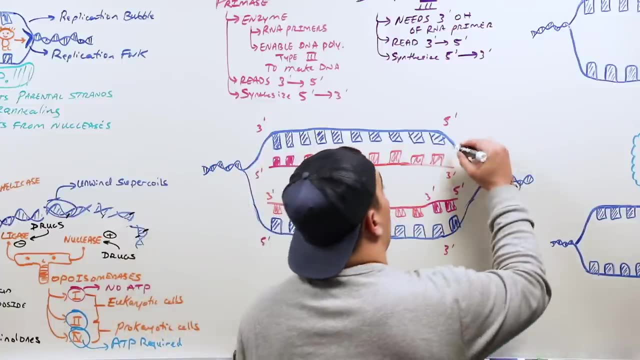 Do you notice something really interesting here On this strand which we called again. what did we call this strand? Well, we had one primer and then DNA for the continuous way towards the replication fork. We called this the leading strand. So the big thing I want you to know. 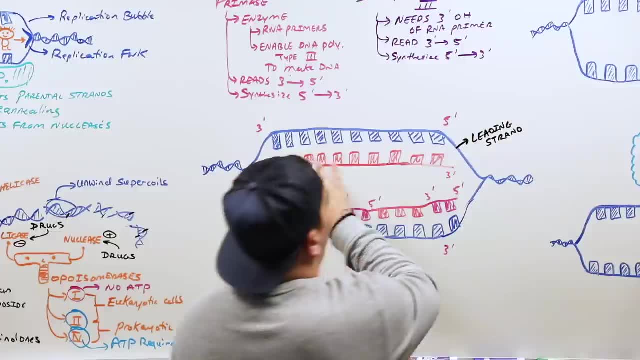 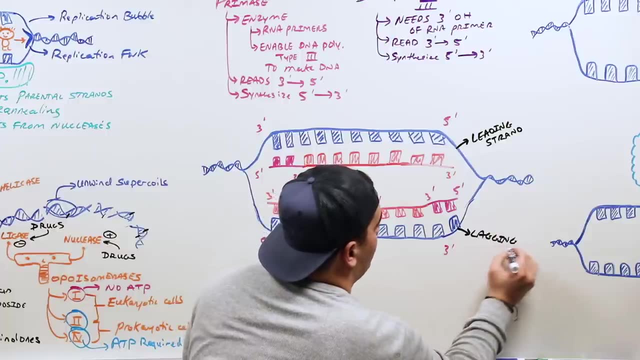 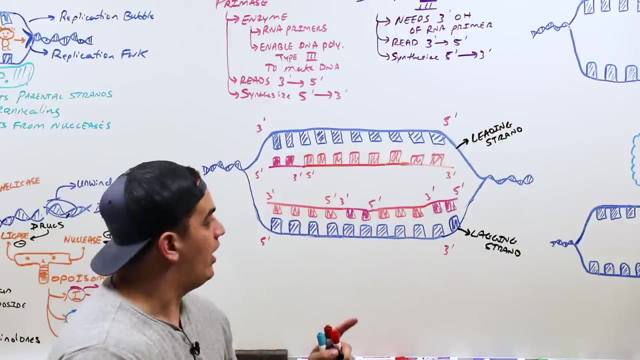 is that you have one RNA primer and then a continuous DNA strand from that point on On this strand called the lagging strand. something different happens here, where you have a couple RNA primers, okay, And then kind of stretches of DNA between those RNA primers. 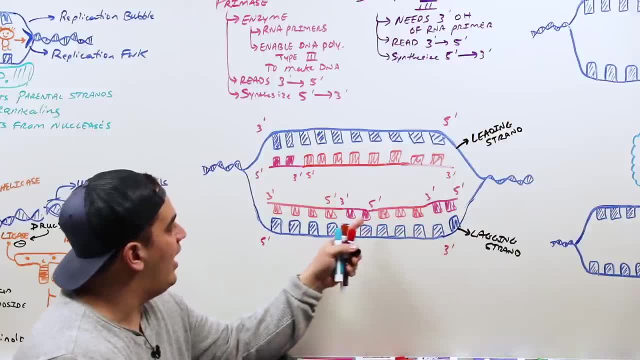 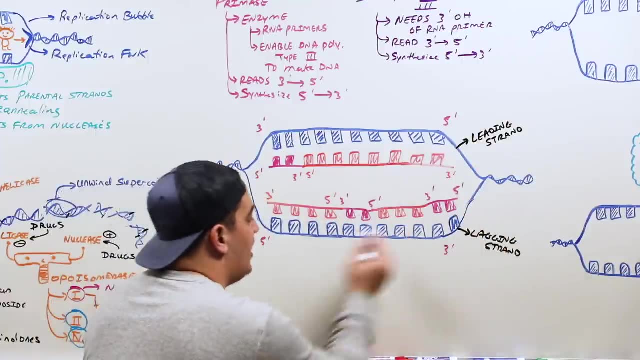 This kind of like broken up portion where there's RNA DNA, RNA DNA, and if we continue to keep elongating it, we'd have more RNA DNA, RNA DNA. This gives a particular name, which is called Okazaki fragments. 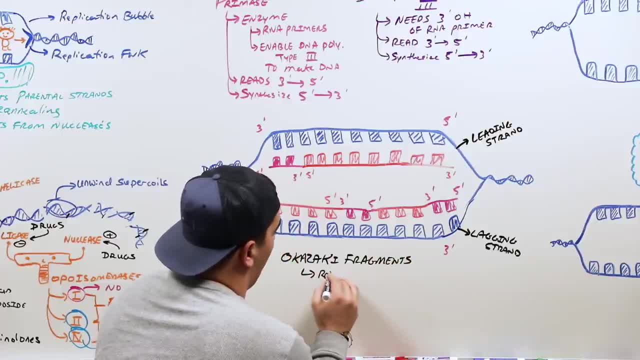 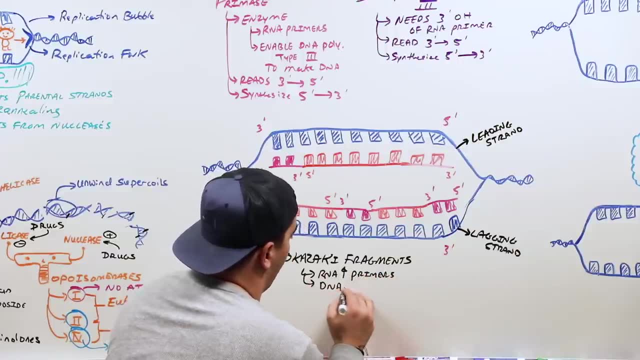 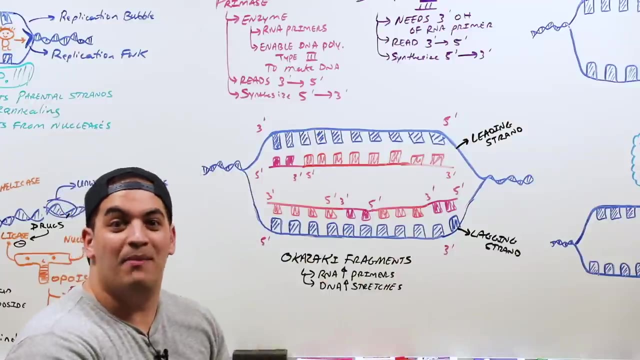 Okazaki fragments And again it's basically where you have multiple RNA primers and multiple stretches of DNA stretches. So multiple DNA stretches and then multiple RNA primers. It's a mix of them And that's a problem, okay. 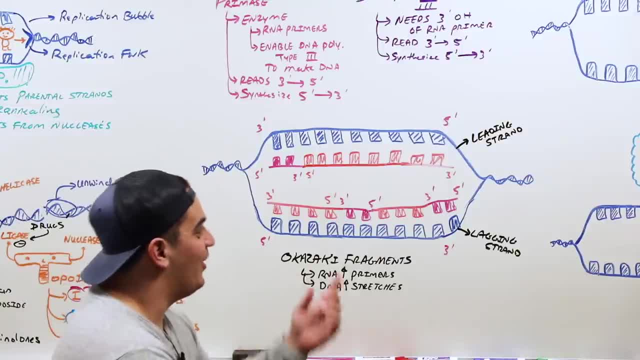 Because you're gonna see now there has to be another thing that we have to do. We want everything. when we replicate DNA, it has to be all DNA. We can't have it be DNA one, DNA, DNA, DNA, DNA, DNA. 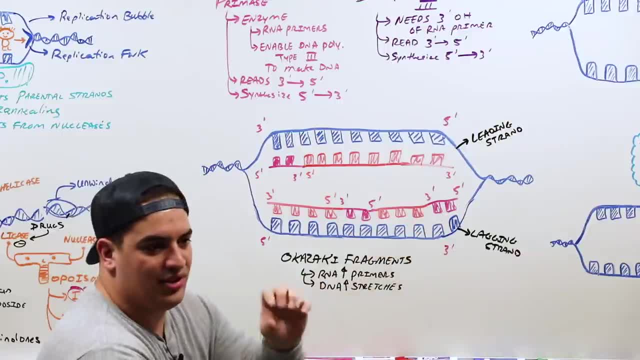 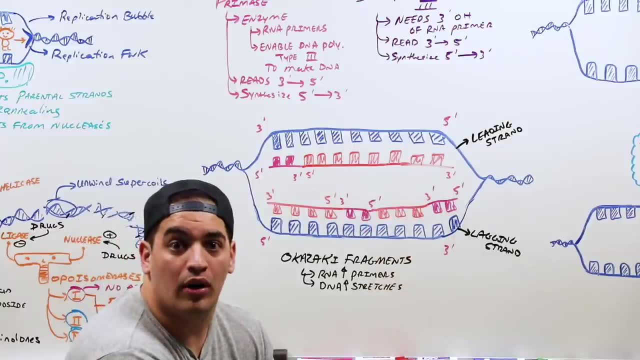 We can't have DNA with a little bit of RNA. So we're only using these primers as just kind of a point to build off of. After we've built some stuff, we're just gonna go in and cut those things out because we don't really need them anymore. 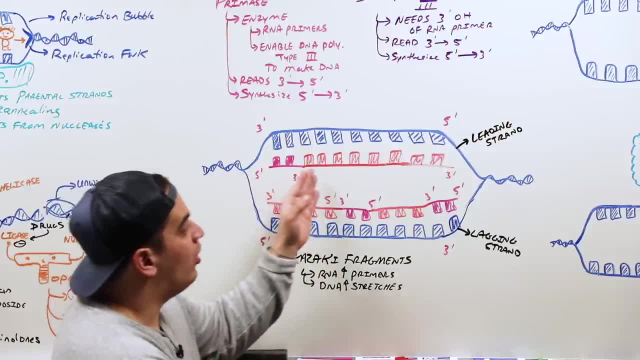 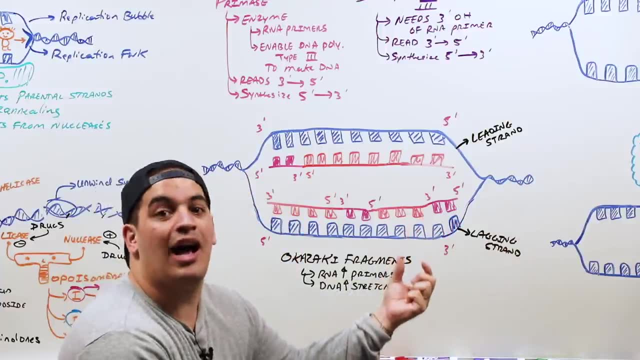 So now let's talk about the next part, which is, we've started to kind of create these primers that we needed to build the DNA off of. Now we don't need the primers and we gotta get rid of it. How do we do that? 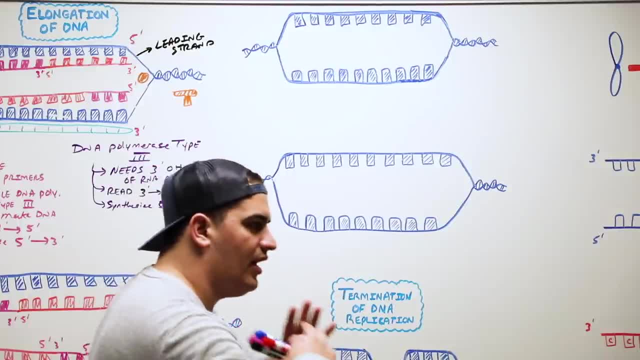 The next thing that you guys need to understand is: okay, we've used our RNA primers for the DNA polymerase III to kind of build off of and make DNA from. We don't need those primers anymore. We gotta get rid of them. 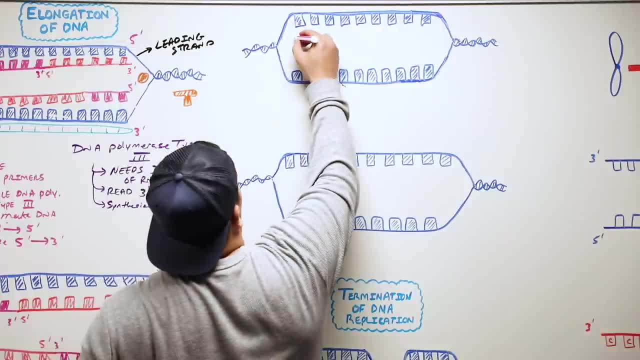 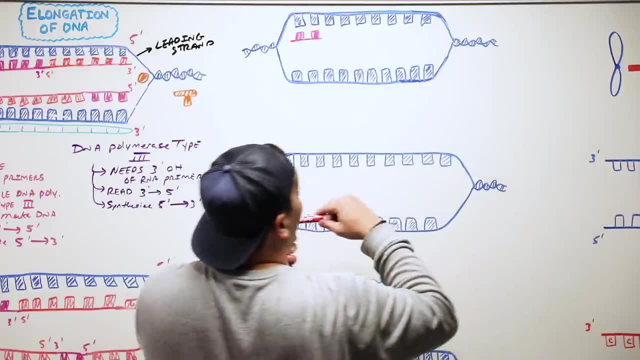 So let's draw the diagram that we had previously, which, again, we only had what A little stretch of RNA, primer here, and then the rest of the length down, going towards the replication fork, which, again, what is this strand here called? 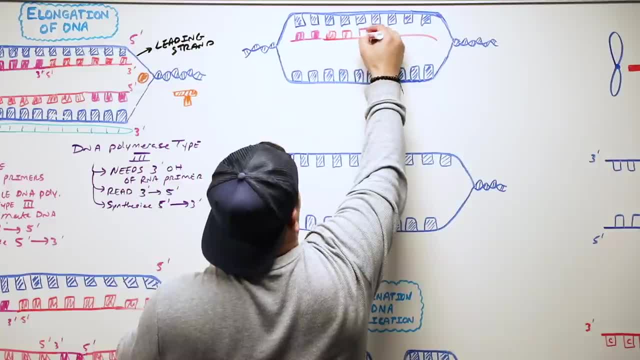 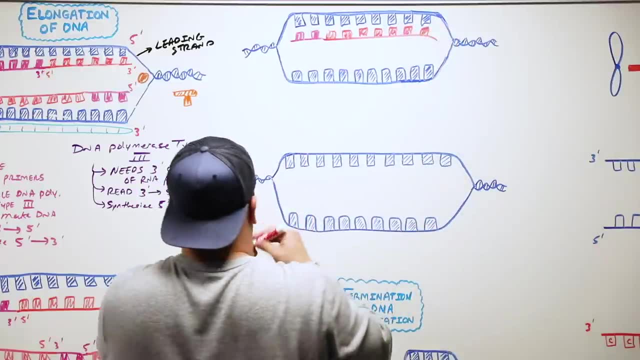 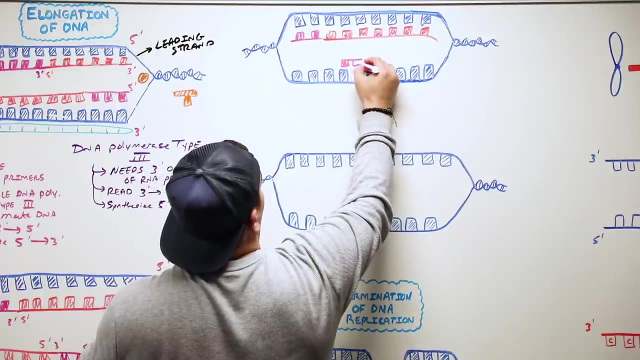 The leading strand is gonna be all DNA. Okay, So now this is really important, where we gotta talk about one more thing in just a second. And again, if you guys remember, on this strand, on the lagging strand, we had a couple RNA primers. 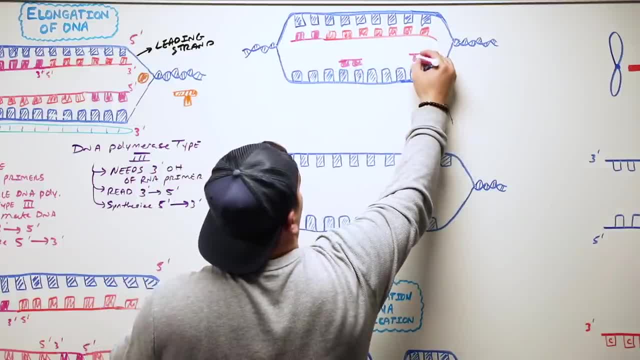 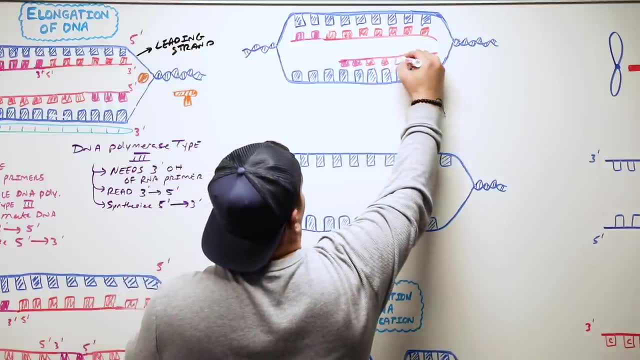 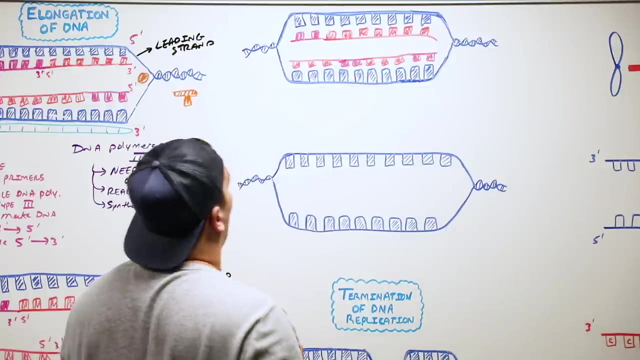 that were in between the stretches of DNA, creating what's called Okazaki fragments on the lagging strand. right, We talked about that. So now the next goal here is that we have to remove those RNA primers. But before we do that, I gotta mention one more thing. 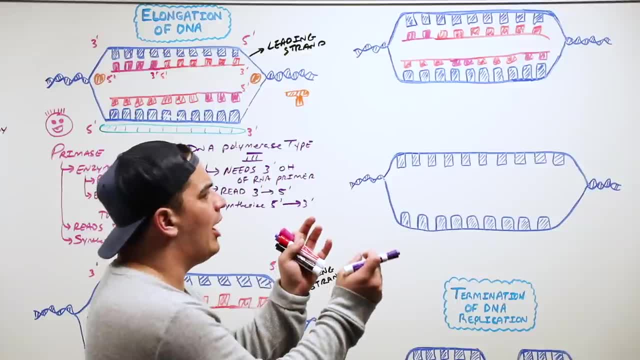 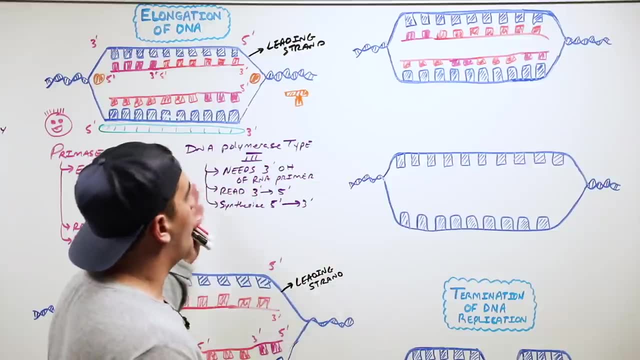 So before we talk about how we remove these RNA primers, I really wanna take a quick second here to explain something else that DNA polymerase type three can do. So we know that it reads the DNA okay, from three to five. 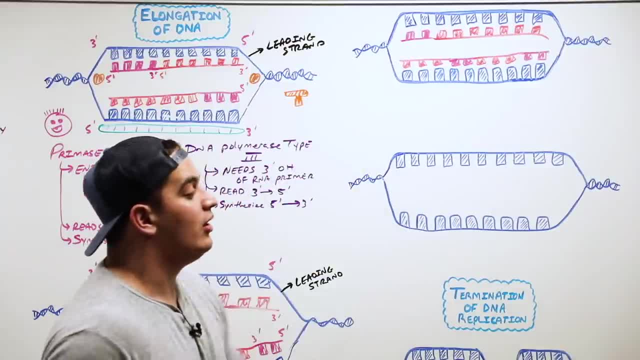 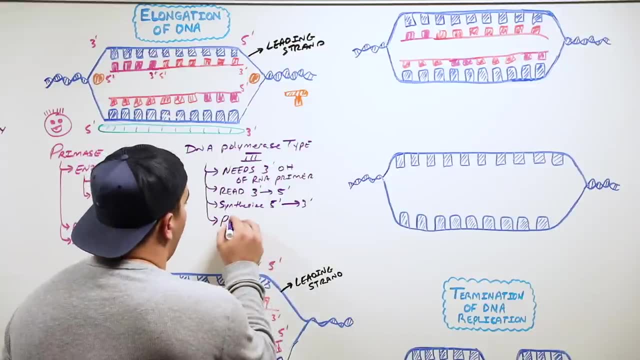 and then synthesizes nucleotides off of the RNA primer from five to three. But it also has one other function- It's called a proofreading function- which is very important before we talk about the RNA primers, And this proofreading function is helpful to prevent mistakes. 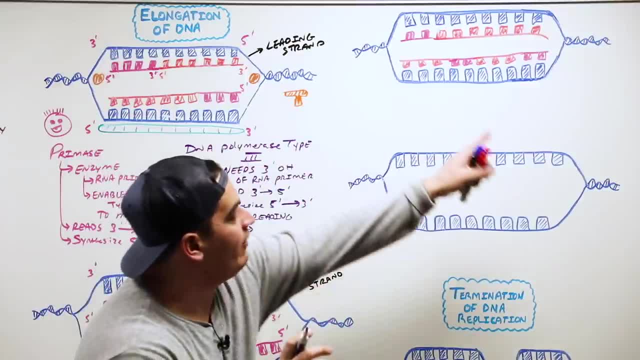 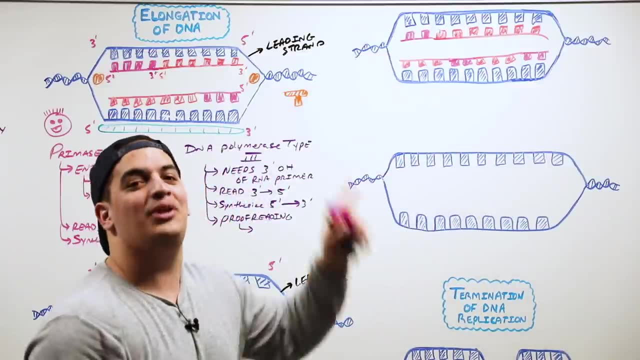 And what it does is, let's say: okay, it reads three to five, reads all the nucleotides from a three to five direction, And then synthesizes nucleotides in a five to three. After it does that, it says: okay, let me check my work. 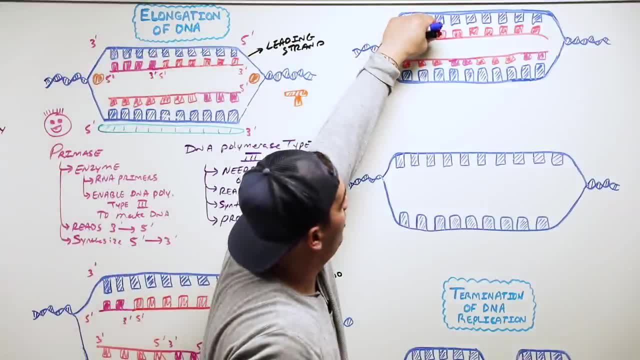 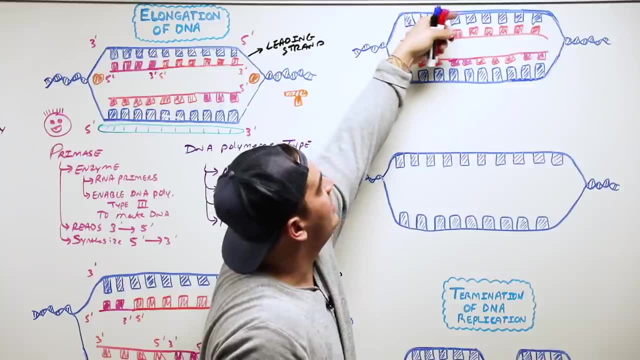 It goes back and it finds the connection between this point and says, okay, is this a good connection? Yeah, that's a good one. A and T are connected together. Oh, G and C are connected together. A and G. oh, this isn't a correct. 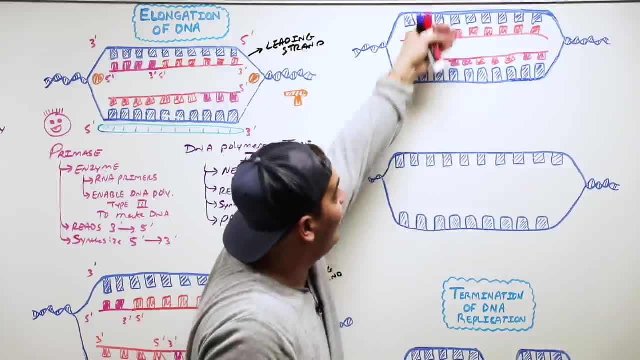 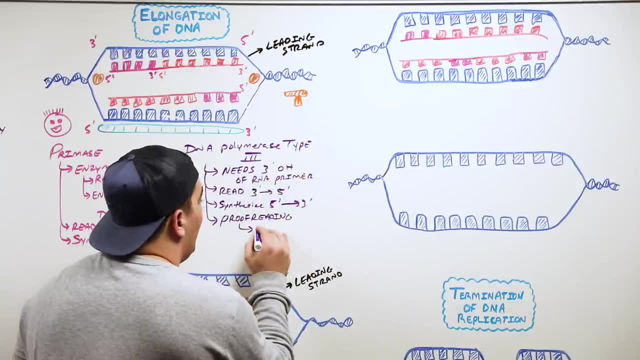 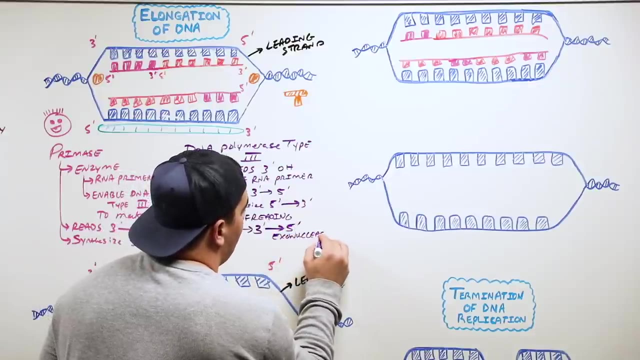 complementary kind of base pair. I need to cut that out. So it reads from three to five and if it finds any mistakes, it reads: okay, it uses what's called a three prime to five prime exonuclease activity, where it says: okay, let me read here: 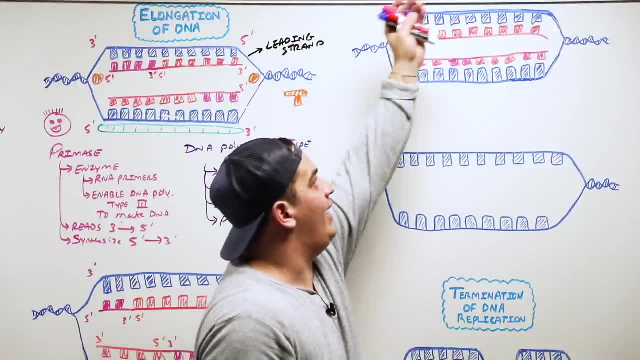 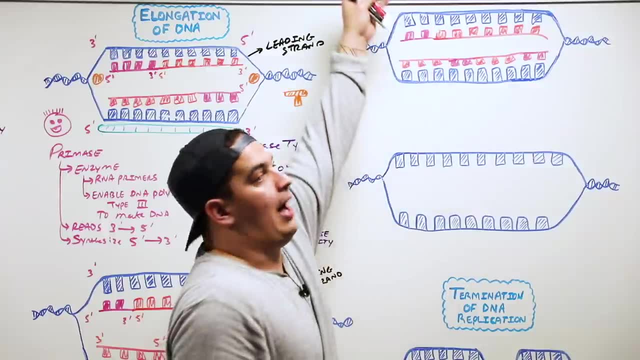 I'm gonna read it and it says: okay, three to five. I'm reading A, T and again it's complementary base. It should be T, it should be A, G, A. ooh, not a correct one. 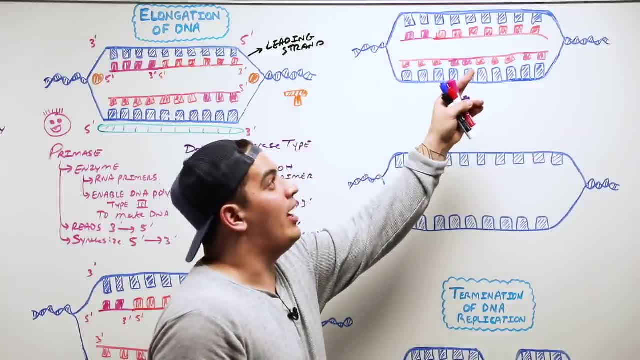 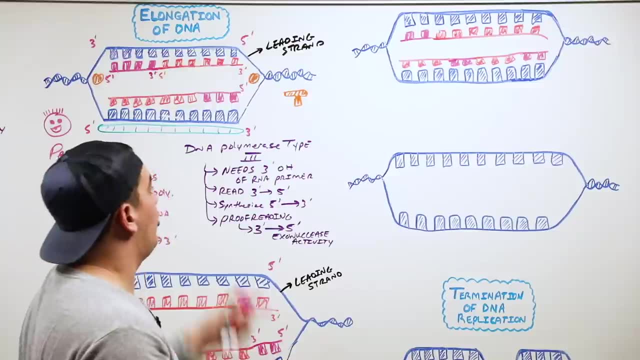 I'm gonna cut that out. read it again, make sure I have it. Okay, it was G, it has to be C, and synthesize the correct nucleotide in the five to three direction. So big thing I need you to remember. 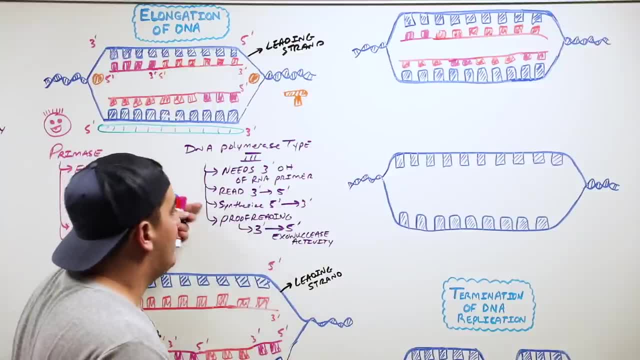 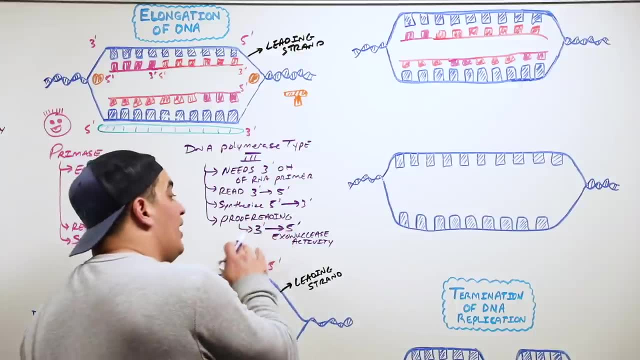 for DNA polymerase type three reads DNA three to five. synthesizes nucleotides five to three. proof reads back in three to five and, if that's incorrect, uses a three to five prime exonuclease to cut it out and put in the correct complementary nucleotide. 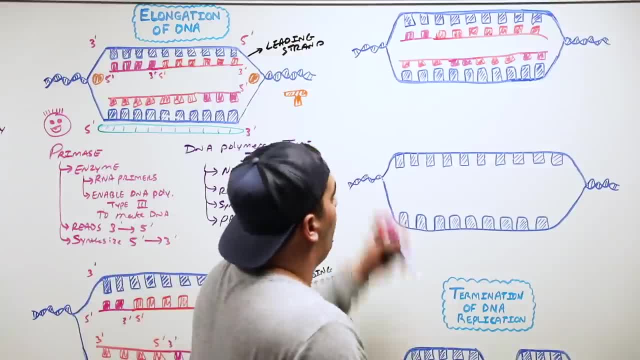 Very important. Okay, now we gotta get rid of these RNA primers. How do we get rid of the RNA primers? Well, the DNA polymerase three is not the answer. Okay, so we're gonna get rid of the RNA primers. Well, the DNA polymerase three is not the answer. 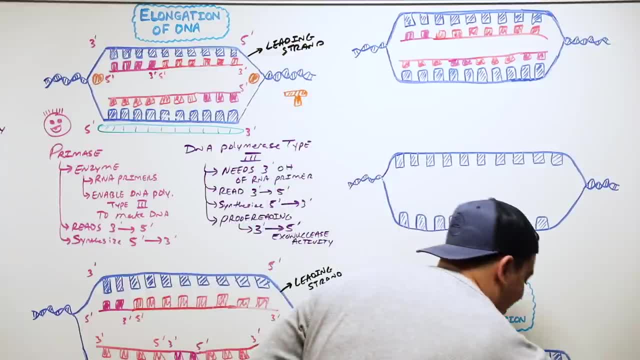 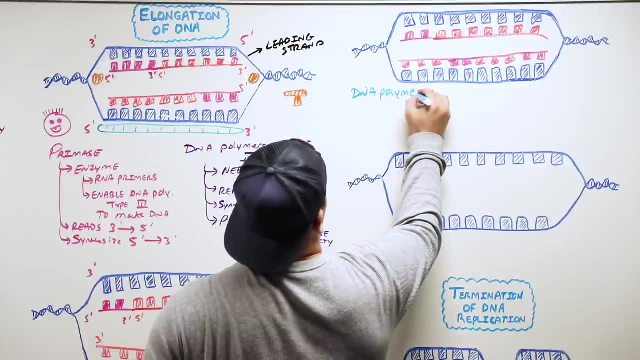 Okay, so we're gonna get rid of the RNA primers. Well, the DNA polymerase three is not the answer. The next enzyme- as if there isn't enough enzymes- is called DNA polymerase type one. So DNA polymerase type one comes to the rescue. 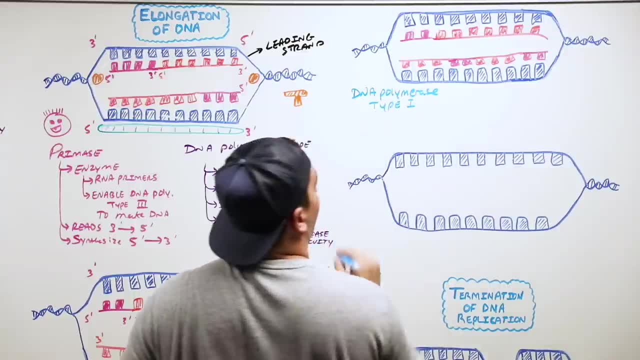 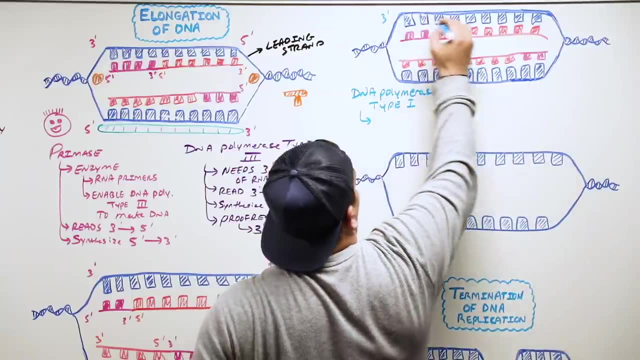 So DNA polymerase type one comes to the rescue And what it does is it starts here and it finds this. And what it does is it starts here and it finds this. Okay, so let's say here we had our three prime end here. 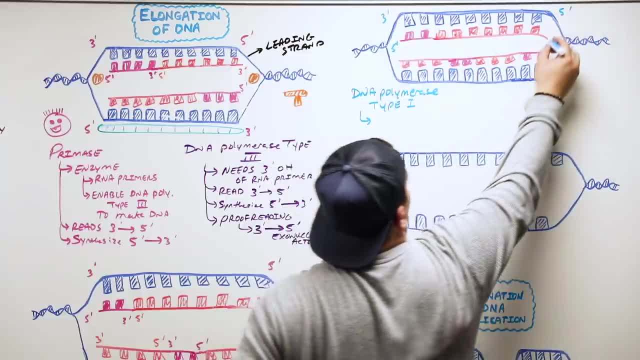 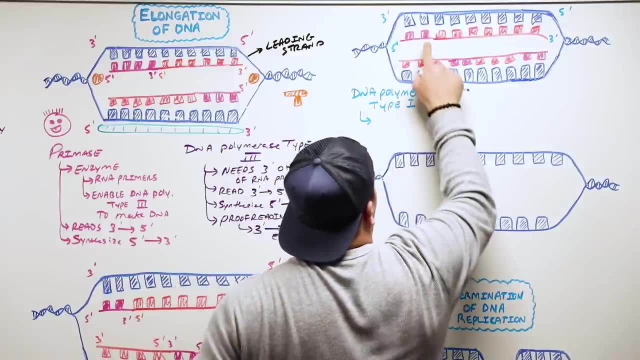 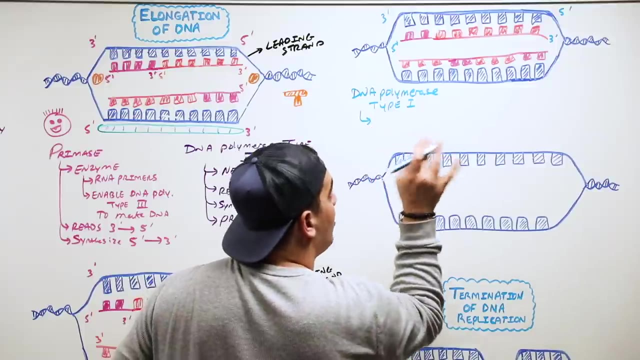 five, prime end here. The new strand would be synthesized from five to three. What this enzyme will do is it'll come in and it'll cut out these primers going from the five to three direction. So it removes primers or it plucks those little primers out. 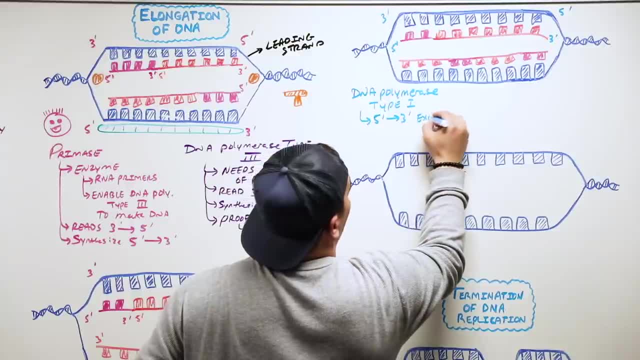 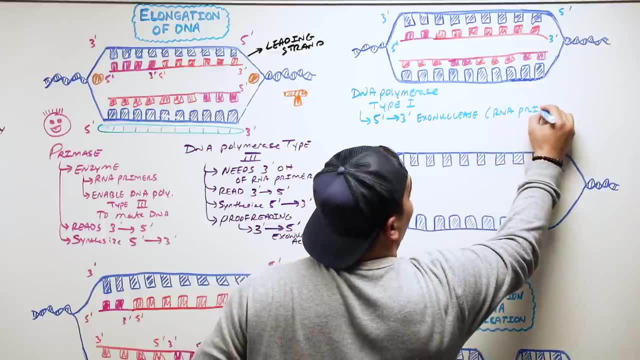 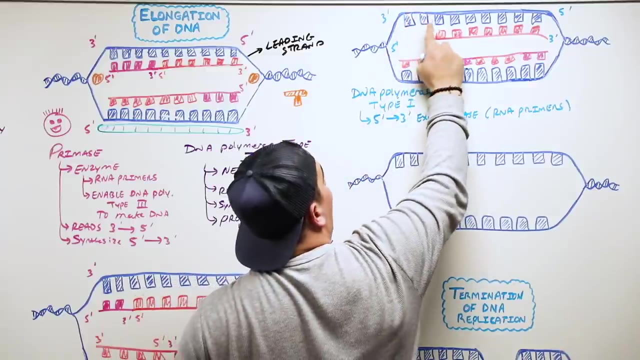 in a five to three exonuclease activity right, Particularly for what? To pluck out the RNA primers. So this guy will come in and it'll say, okay, pluck, remove that one, Pluck, remove that one. 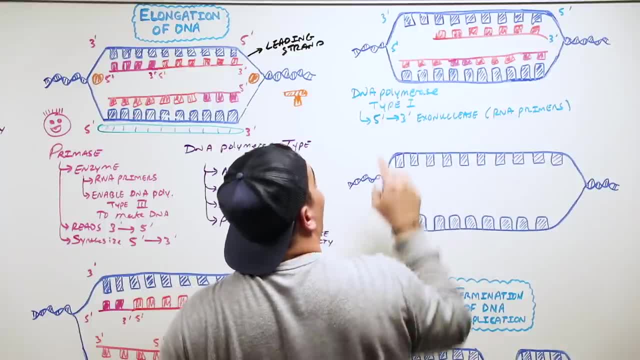 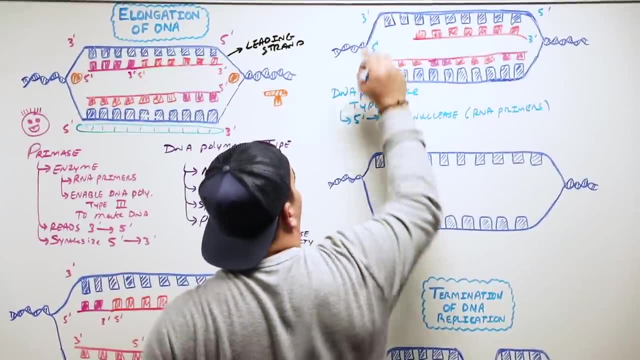 And then what it'll do is, once it plucks those out, it then says, okay, I'm gonna read this strand from three to five. So it reads the one that it plucked out and says, okay, that's an adenine. 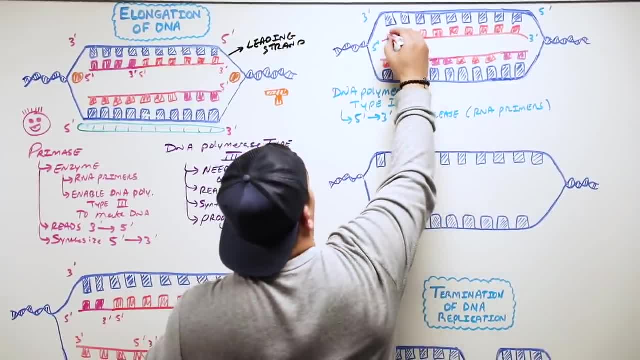 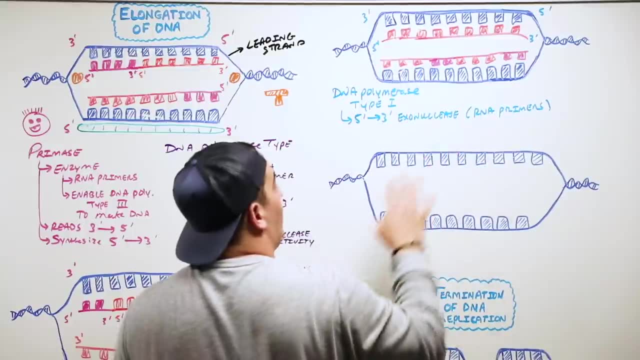 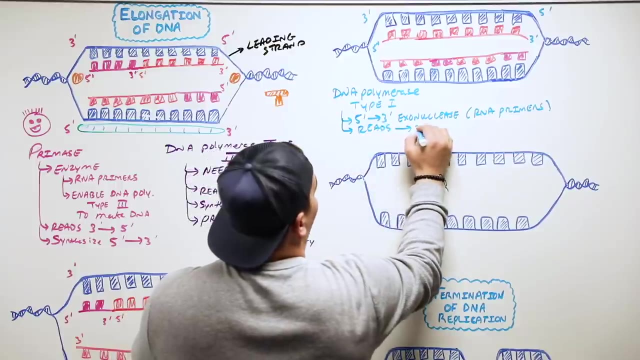 What do I need to add here? I need to add in thymine- Oh, this is thymine. I need to add in here adenine, So it plucks off the primers. Then what does it do? It reads the DNA from three to five. 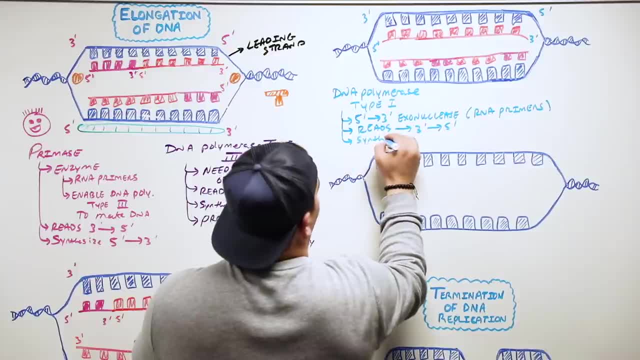 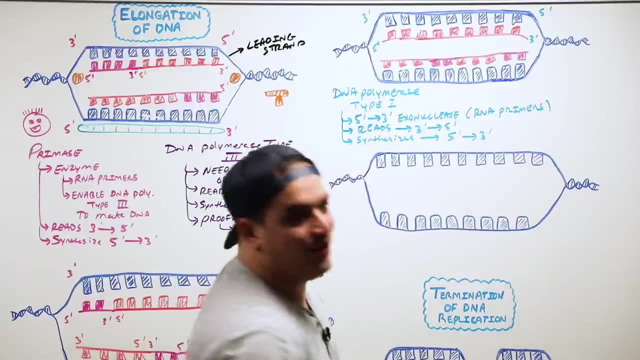 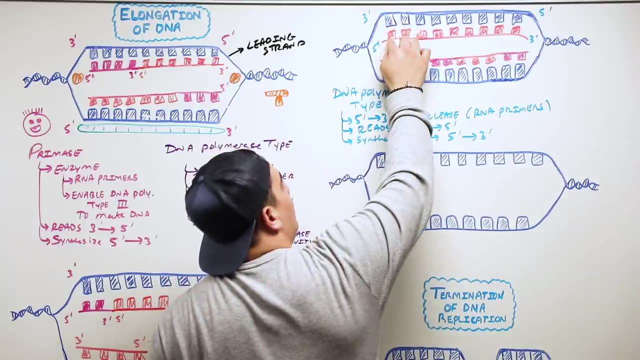 and then it synthesizes from five to three. You know what else it can do. One more function. Let's say: okay, it plucked off the RNA primer. reads it as adenine puts a thymine. Reads it as guanine accidentally puts an adenine. 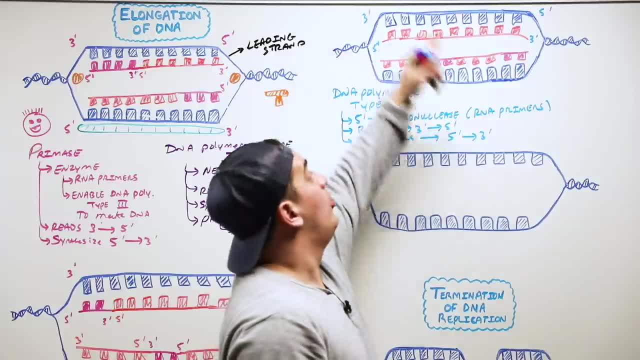 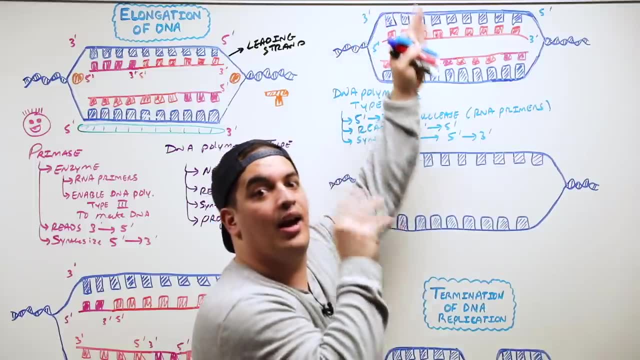 Has to go back and proofread it though, because that's always a thing that they have to do- Proofreads it and says: ooh, not a good connection. I don't want that. What do I need to do? I need to pluck that thing out of there. 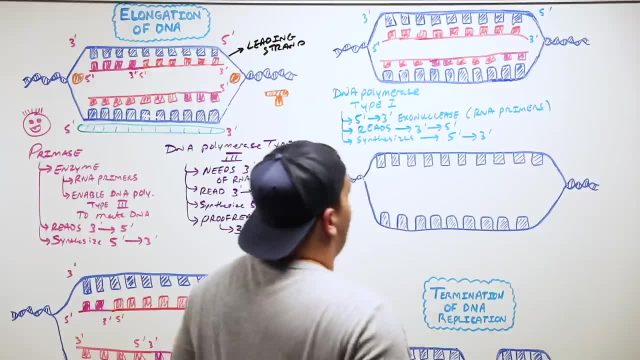 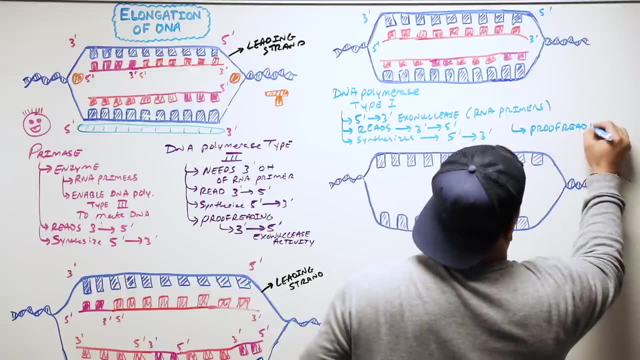 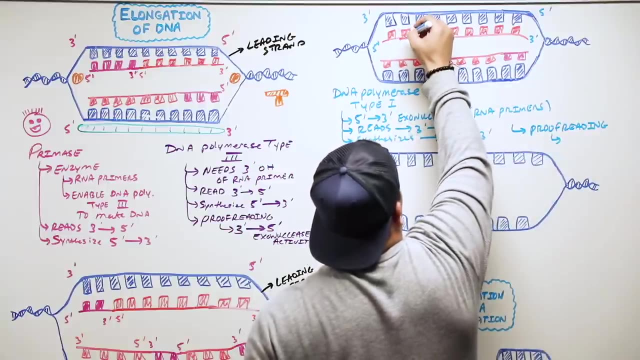 and put the correct nucleotide. So the last thing DNA polymerase type one can do is, again, it has that proofreading type of activity Where it can do what It can read from three to five If it finds an incorrect base pair connection. 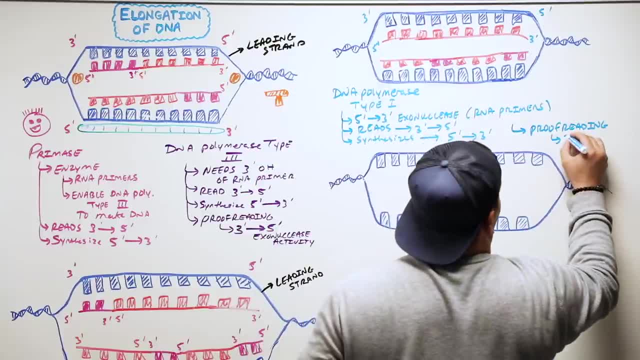 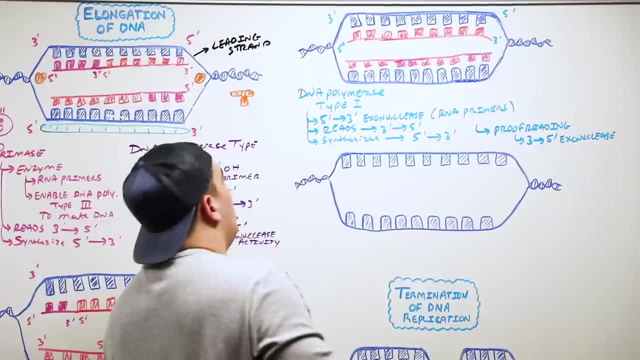 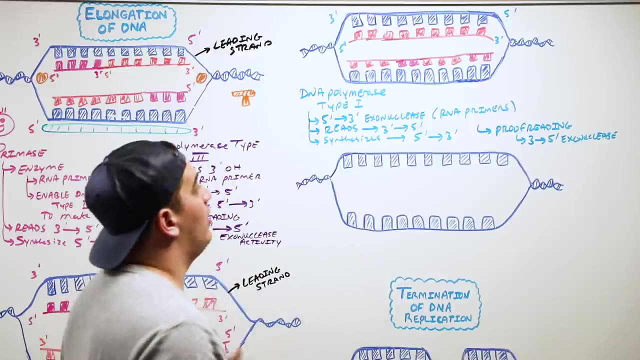 it cuts it out. and when it cuts it out it cuts that at a three to five exonuclease type of fashion. Okay, So the big difference that, if you ever get asked between, what in the heck is the difference between DNA polymerase type one and DNA polymerase type three? 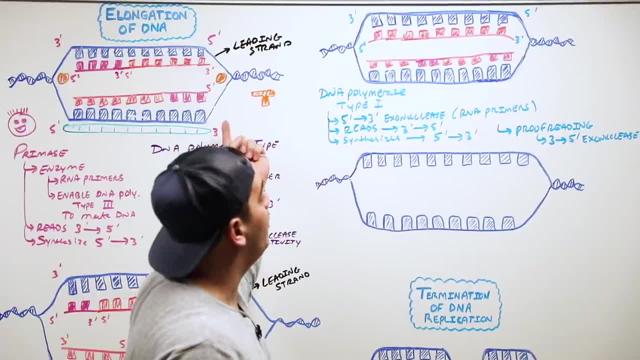 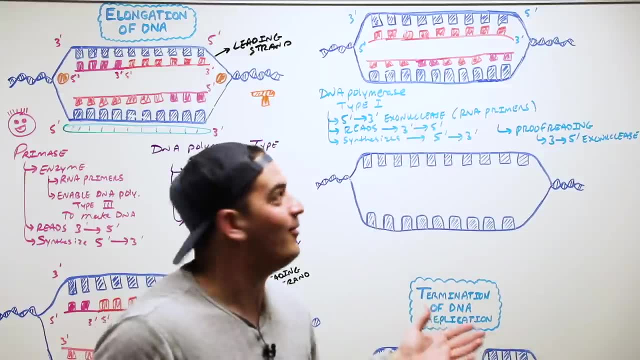 really. the big difference is that this guy can do everything type three can do. It's just it has that five to three prime exonuclease activity, where it plucks out the RNA primers. Everything else is the same, though. Now the next thing is DNA polymerase, type one. 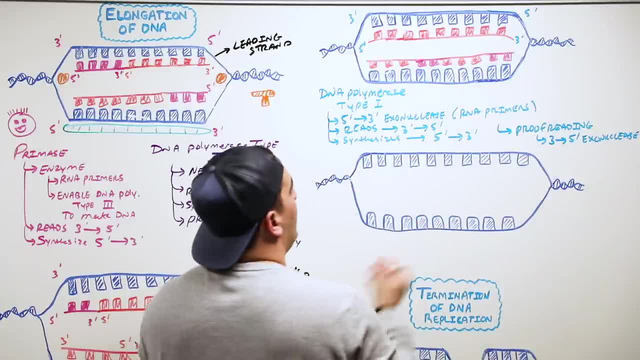 We talked about on this leading strand, On the lacking strand. it's a little interesting. It'll come in and again it'll use its five to three primers. It'll come in and again it'll use its five to three primers. 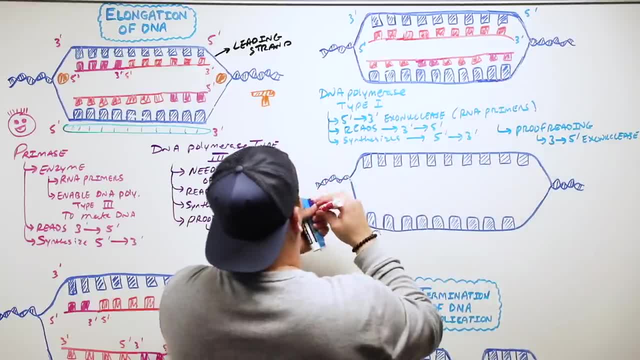 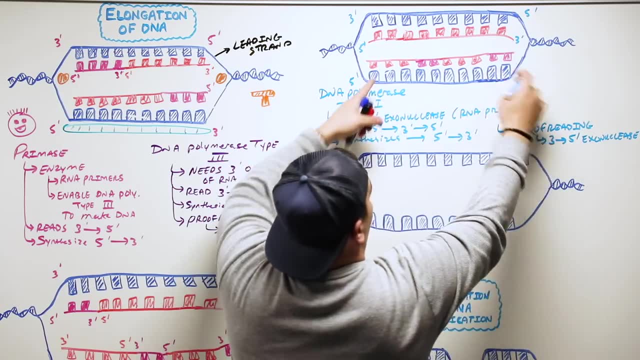 It'll come in and again it'll use its five to three primers exonuclease activity. so again, let's use our combination here of what we know. this was three, this was five, so anti-parallel. this has to be five to three for the old strand. the new strand would then be what read: three to five. 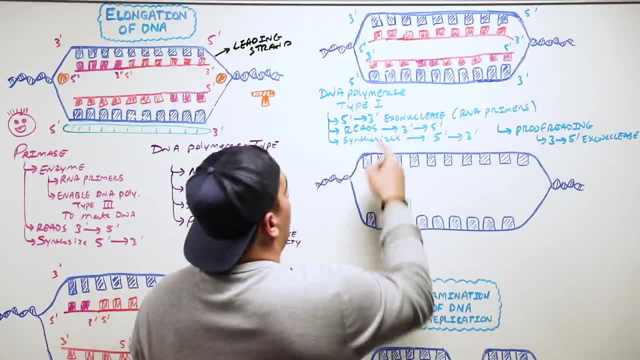 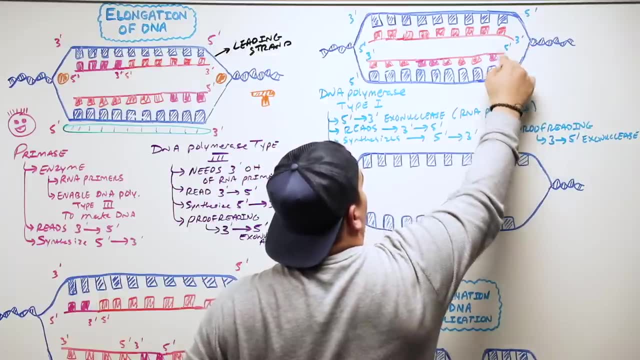 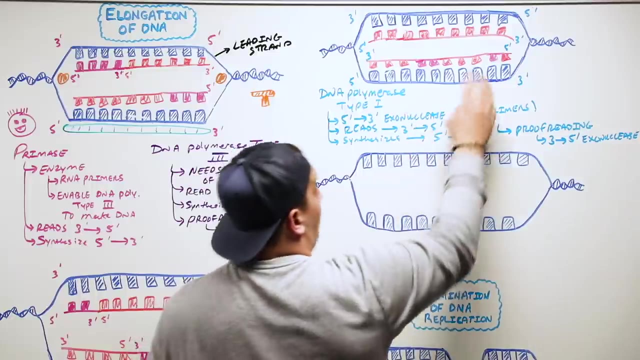 synthesize five to three. so this DNA polymerase will come in and it'll start moving down and at this point it'll pluck off an RNA primer. and then what will it do? read three to five and synthesize five to three, come to the and then proof read: it is it correct? oh, it is okay if it's not use my three to 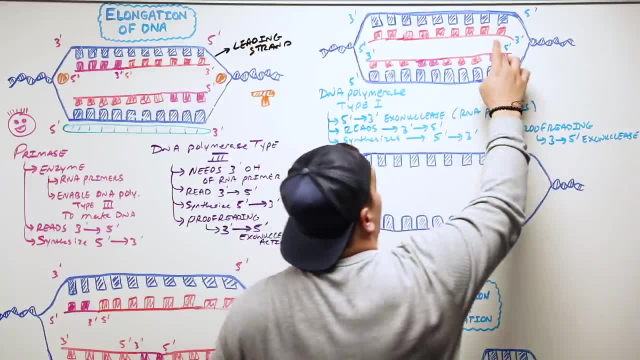 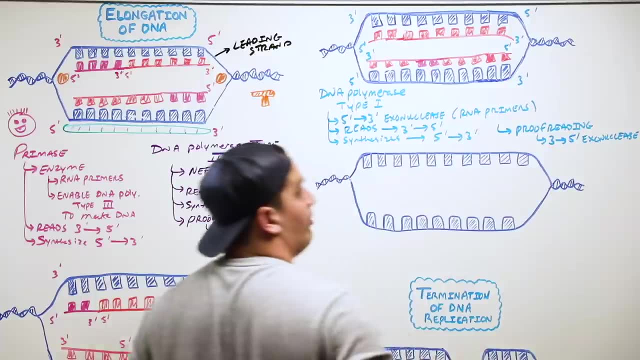 five prime exonuclease to cut it out and then put in a new one, goes to the next one, plucks off the RNA primer and does the same thing, reads three or five, synthesizes five to three, proof reads three to five, then it just keeps doing. 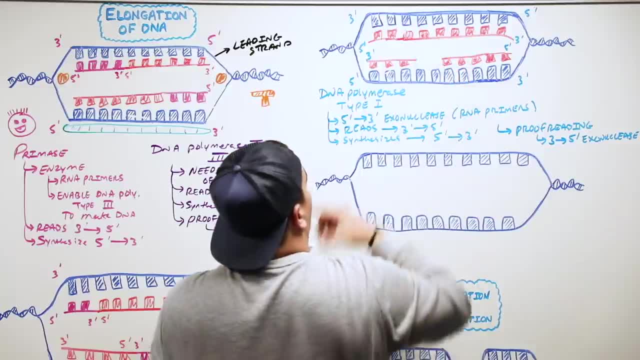 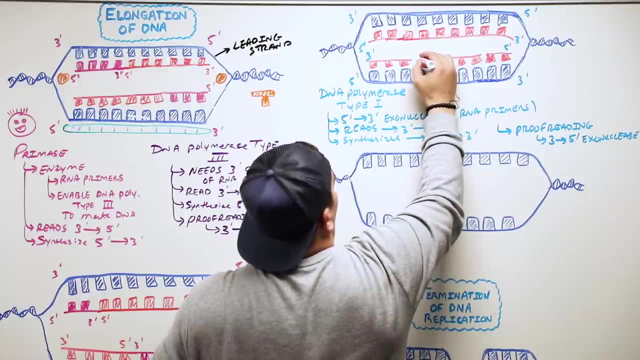 that and plucking these things off. here's the difference, though, and the lagging strain. it creates like a couple gaps. these actually don't contain any of the RNAs that are present in the DNA, and so the DNAs that are completely kind of fused together. So let's kind of draw where we had this here And we'll create. 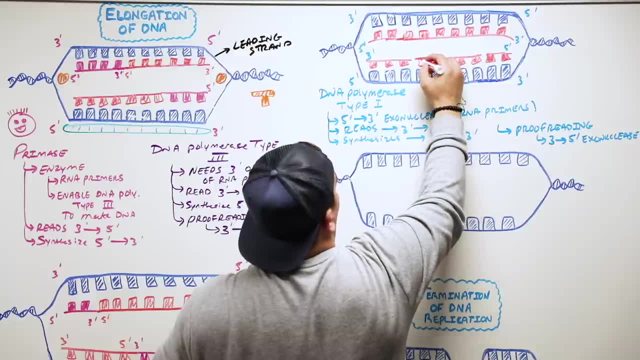 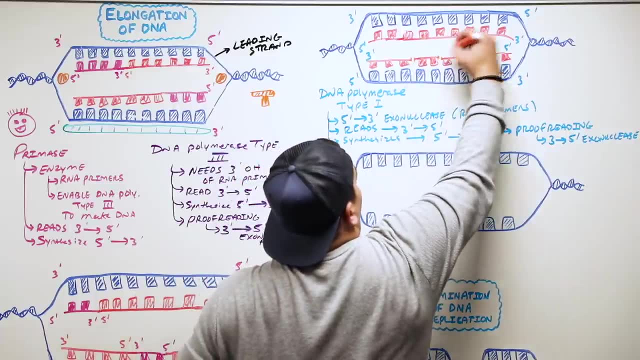 a little space between these points here where the RNA primers were. So there's kind of a little space here. Let's draw it here in orange, So on the lagging strand it creates like a little space where it can't like really fuse these ends where the primers were to the original DNA. Okay so, 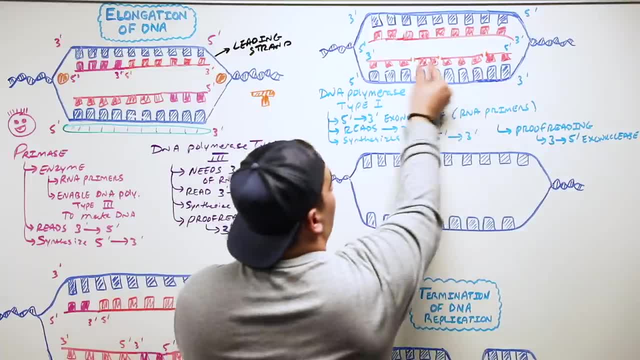 it plucked the RNA primers off and put nucleotides, but it wasn't able to perfectly fuse these ends on the lagging strand. One more enzyme. You're like dude, I can't do no more. I promise One. 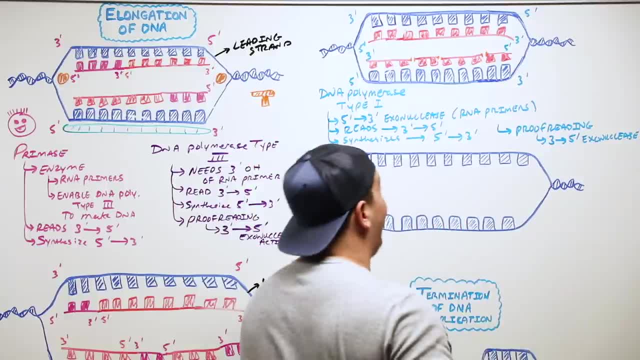 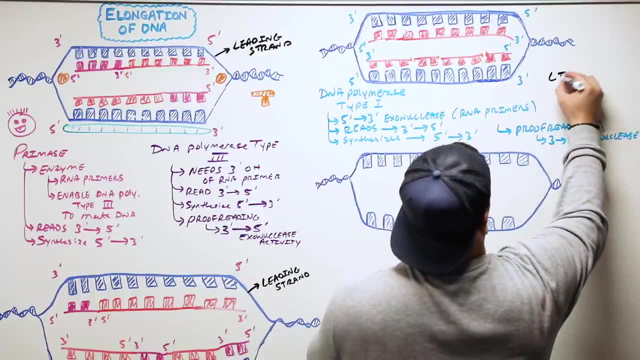 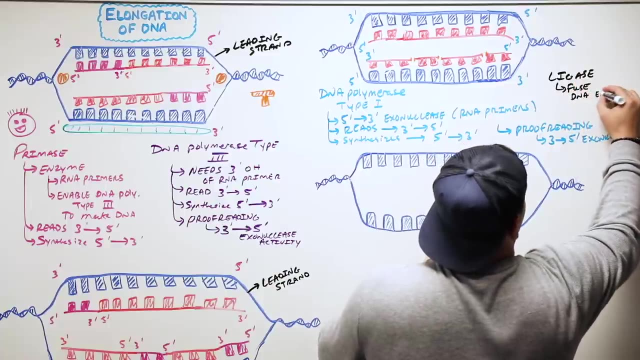 more. This enzyme is called ligase, So it's called ligase. Now ligase will come in on that lagging strand and fuse the DNA ends together- Okay, those basically where those Okazaki strands are. So it's called ligase. So it's called ligase. Now ligase will come in on that. 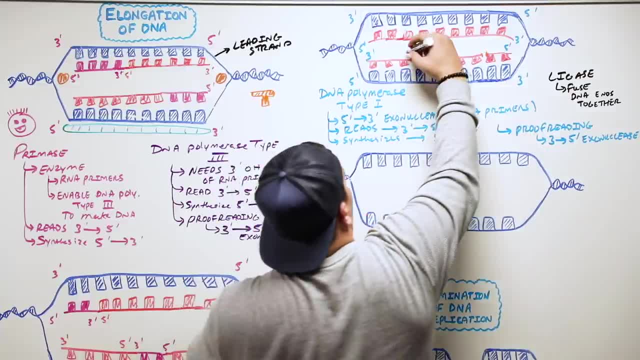 ligase, So it's called ligase, So it's called ligase, So it's called ligase. Now ligase will come in and it'll say: okay, here's these ends, here. I'm going to fuse these points together so that 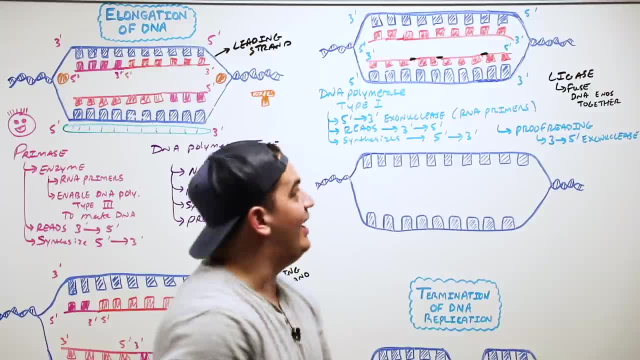 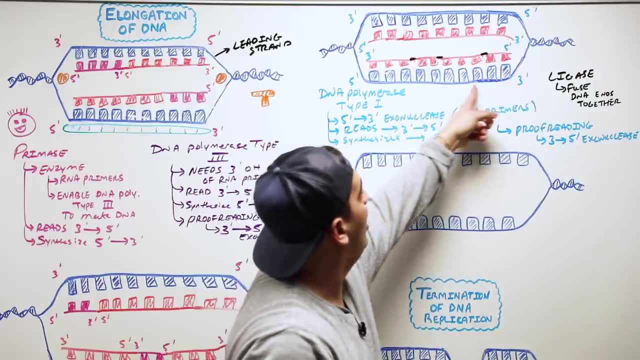 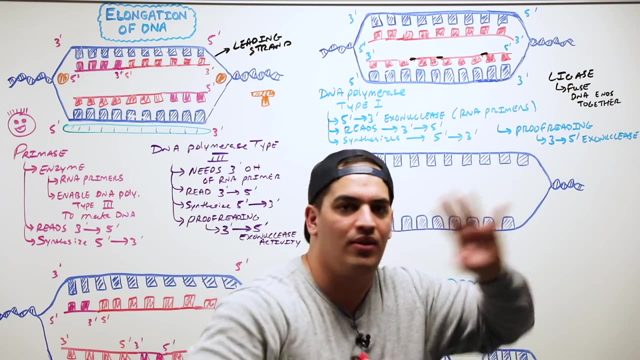 it's perfectly connected and continuous. And now we have a parental DNA with a new daughter DNA strand, Again a parental DNA strand with a whole new daughter DNA strand. that is all continuous and all in sequence. No RNA primers, no, nothing, no breaks. It's perfectly set. now The last thing. 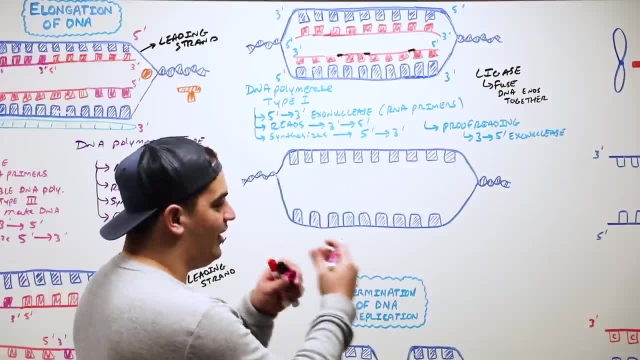 that I want to talk about is the DNA strand. So I'm going to talk about the DNA strand, So I'm here before we go on to termination is we've elongated our DNA. We now took the old parental DNA and made new DNA. The reason why I want you to remember this is that it's very important for 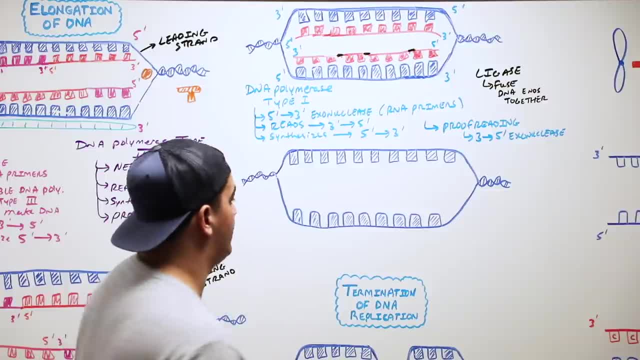 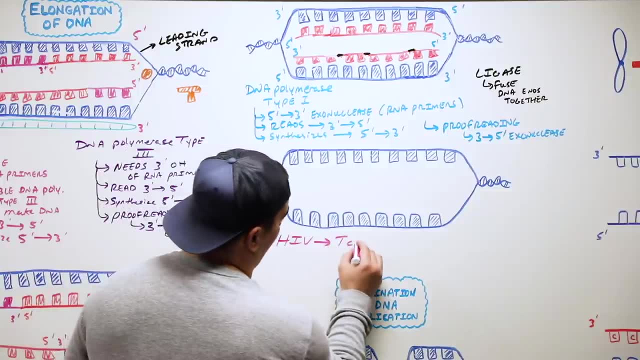 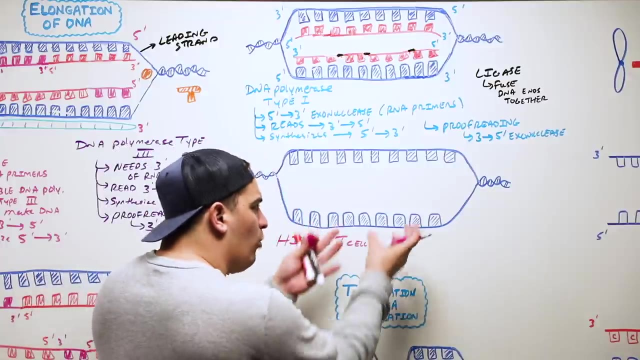 USMLEs to connect foundational sciences with clinical significance. And so in people who have HIV, their T cells are infected with a particular virus called a retrovirus And it's causing this virus to get incorporated into the DNA And then from every point that on that. 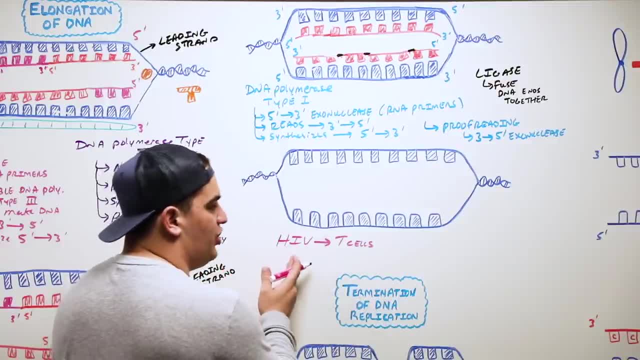 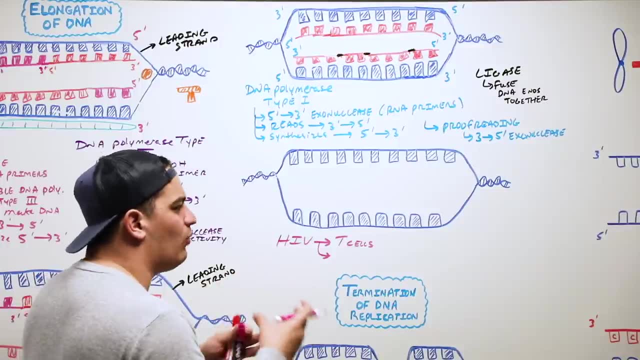 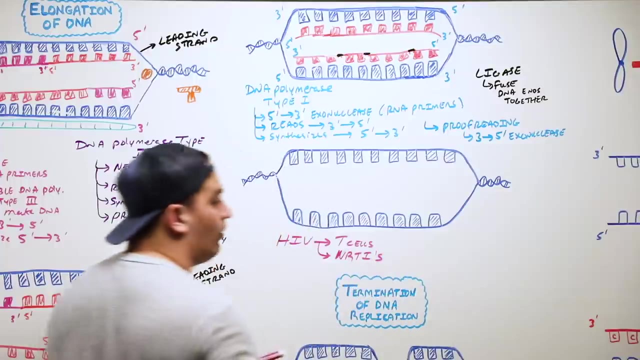 these T cells replicate. they continue to replicate more of the HIV genome. So there's drugs that we use to target this HIV virus and particularly the T cell replication process, And these drugs are called nucleoside reverse transcriptase inhibitors. You're like, holy crap. 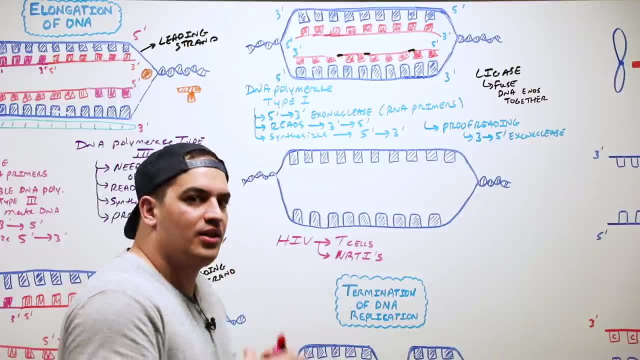 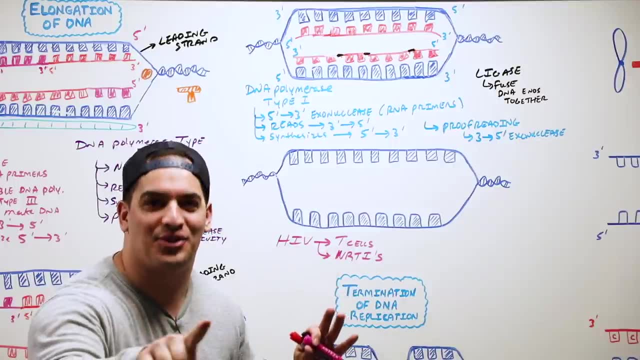 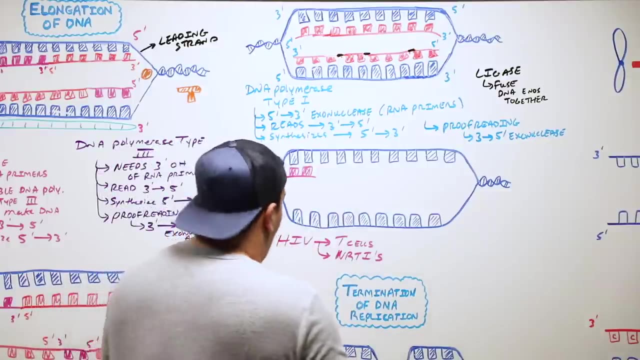 what the heck does that mean? I just want you to remember that they're drugs that are used for HIV and they inhibit the replication process and T cells that have been infected with HIV. Let me explain how this works. This is really cool. Let's say here, I just quickly put down an RNA primer, Okay, And I have my DNA polymerase three. 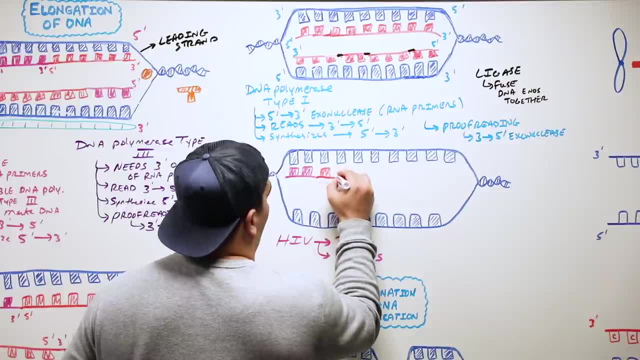 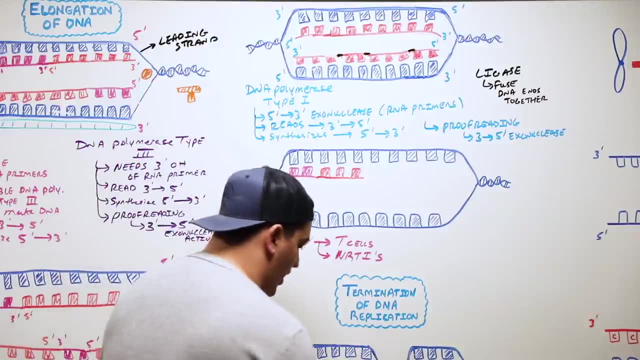 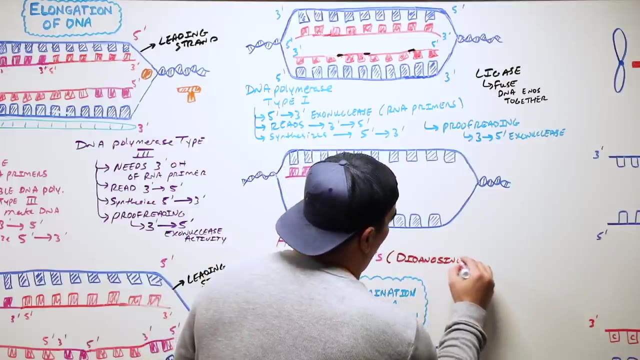 It comes in here and it starts making some DNA right, Uses that three prime end of the RNA primer and starts making DNA. I give them a drug- Let's kind of put here an NRTI. And again, there's many different names of these, like didenosine, zidovudine. There's a whole bunch of these. 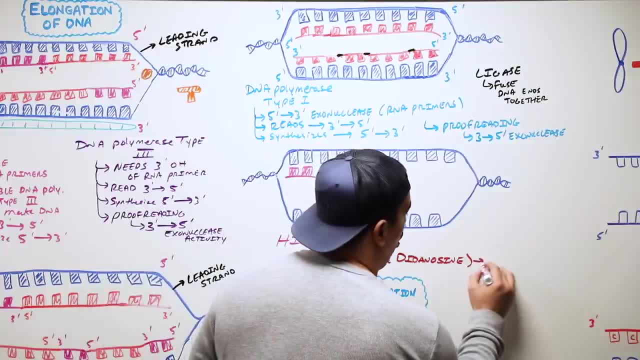 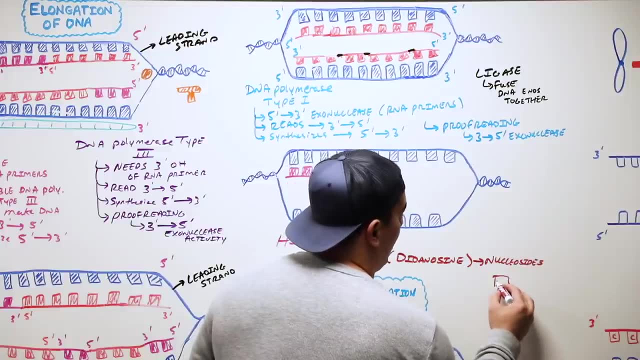 But what I want you to remember is imagine these as what's called nucleosides, Okay, And what they do is imagine here is basically my ribosugar, And then here I'm going to have my phosphate group, And then here I have, like adenine, Okay. 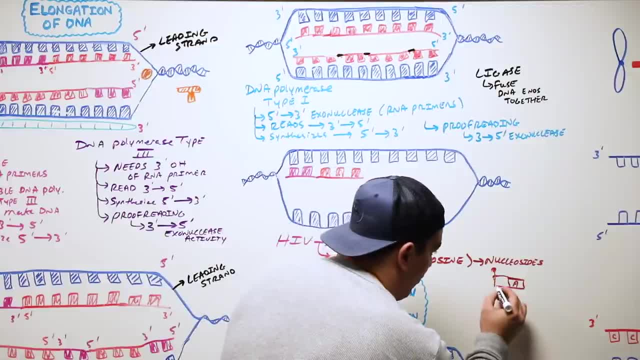 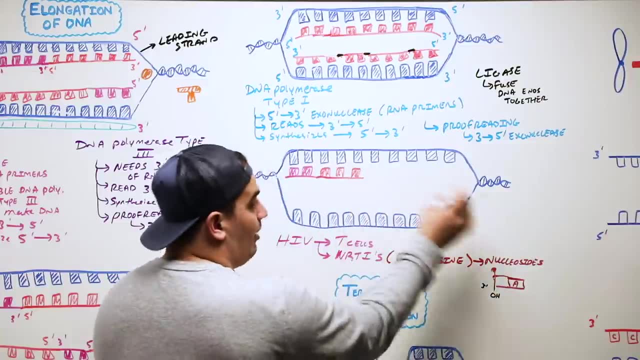 What they do, which is really interesting, is usually on your deoxyribosugar. you should have an OH right And you need that OH on that three prime end in order for the DNA polymerase to continue to keep adding. What they do is: 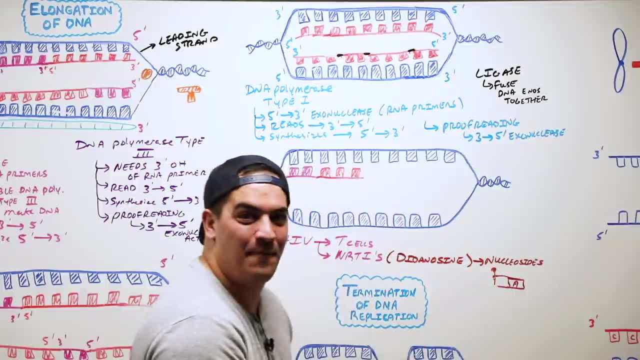 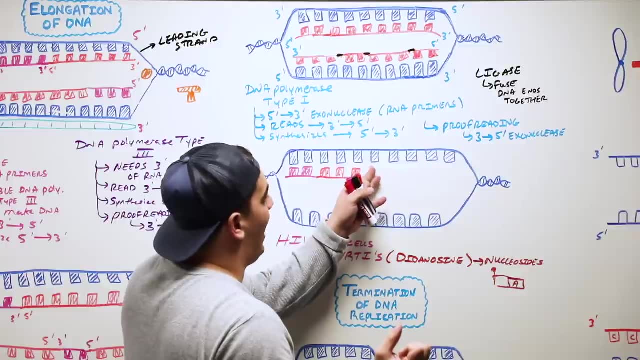 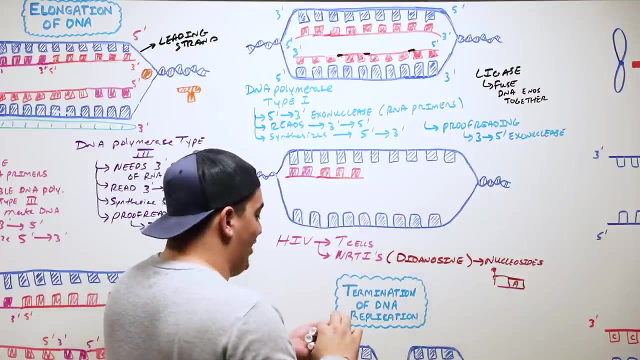 is they remove the three prime OH region. So now the DNA polymerase three will get another nucleotide. It'll read this and say: okay, this is adenine, I'm going to put a thymine or something like that And I'm going to add in this drug. This drug kind of floats around, kind of interestingly. 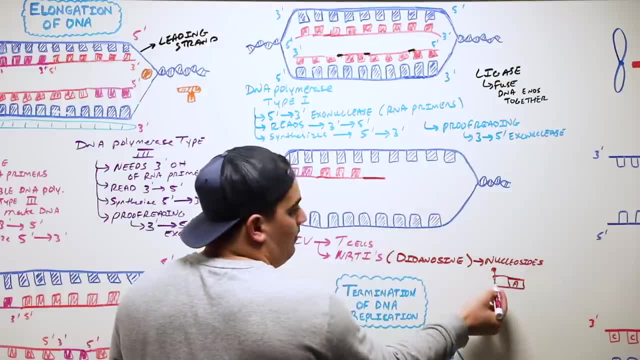 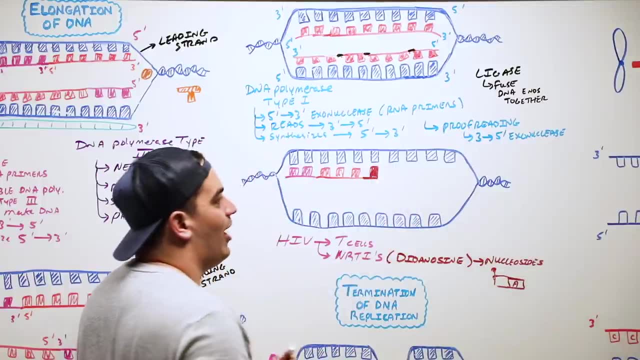 And the DNA polymerase. three will then say: okay, here, this is another nucleotide, just like the ones I've been adding. Let me add this one on. The only problem is is it doesn't have a three prime OH region. So what I'm going to do is I'm going to add this one on. 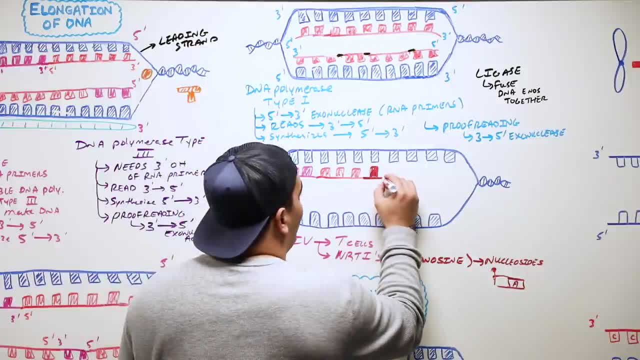 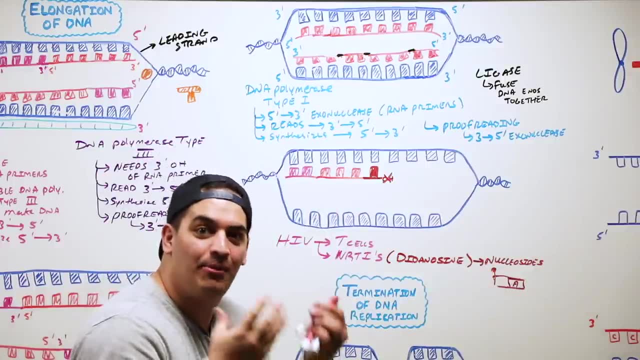 So you know what happens here. Since there's no three prime OH, DNA polymerase can't build off of that. Remember what I told you: DNA polymerase type three needs a three prime OH region to build. If you give a drug that doesn't have that, can you continue? 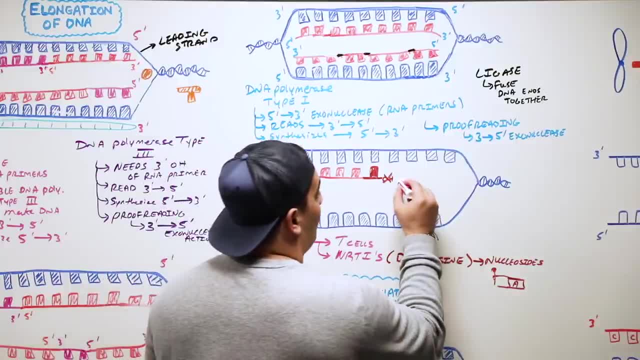 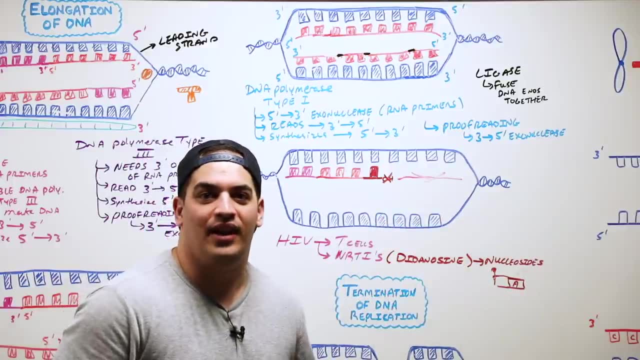 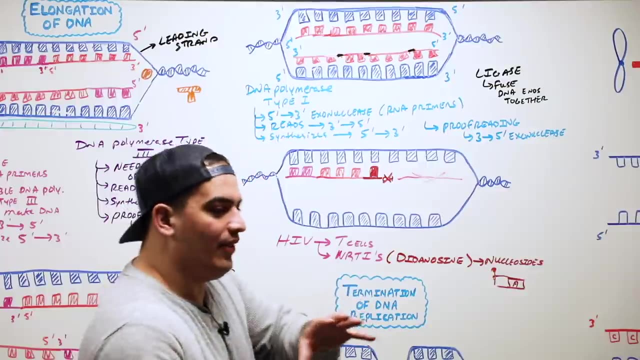 to build off of it. No, So all the DNA replication from this point is inhibited. Are you able to replicate all the DNA within these T cells that have been affected with HIV? No, So that's how it does it. They're what's called kind of like analogs- nucleoside analogs- where you're kind of 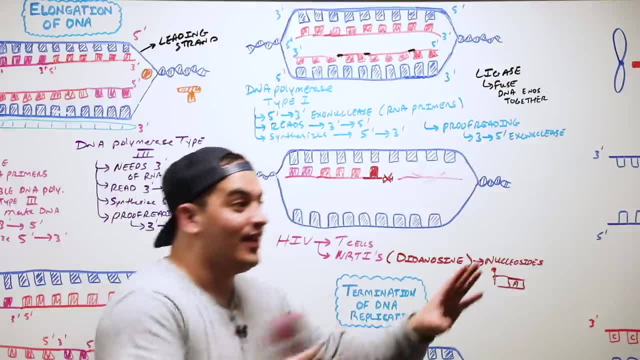 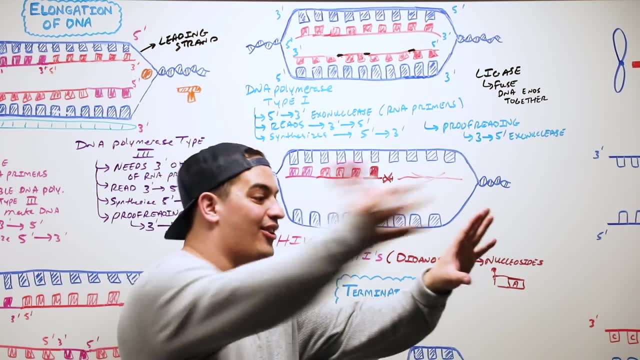 like DNA polymerase three. doesn't know the difference. It's just taking nucleotides and adding on. And all of a sudden, just by chance, you have this drug that it attaches on. It doesn't know the difference, It goes to add another nucleotide on. It's like, hey, that didn't add. 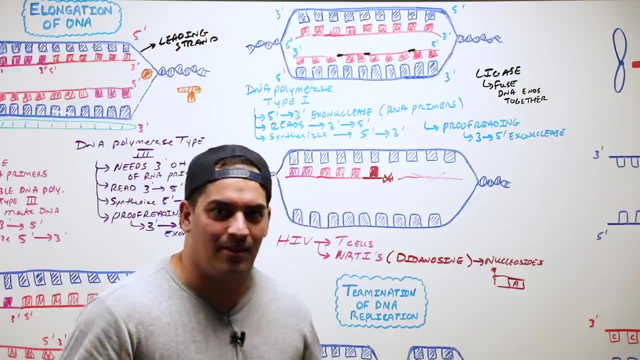 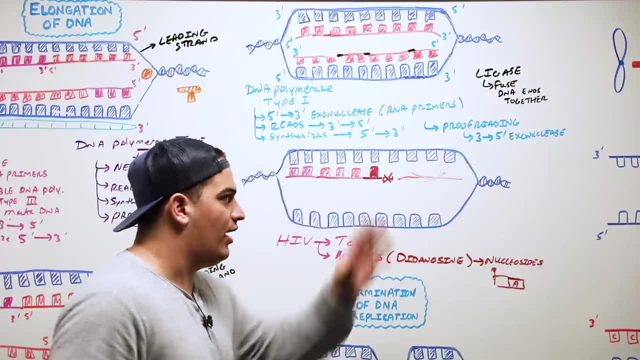 on What the heck I can't add this nucleotide on? And the DNA never gets completely replicated. So it's a good. it's a good clinical point to understand. That covers our elongation. Let's hit it home with termination and take a quick second to talk about telomeres. 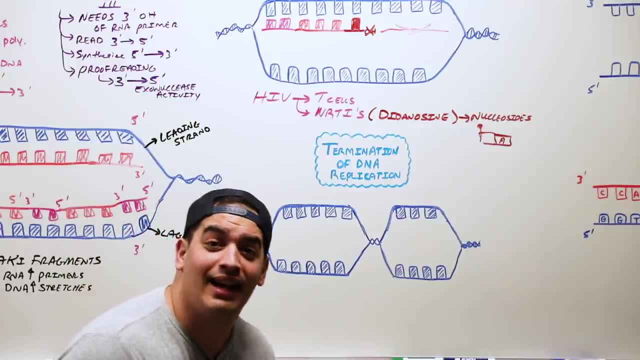 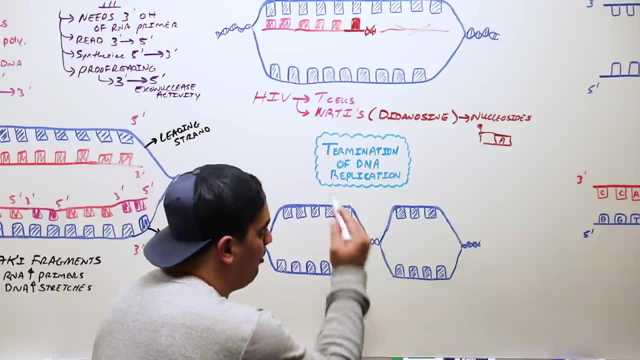 All right, This is actually the easiest one of all. You're probably like: oh please, Zach, I can't do any more. I know this, This is a lot. But let's say that we have another enzyme- OK, that helicase- And we're getting to the point where DNA replication has been completed. 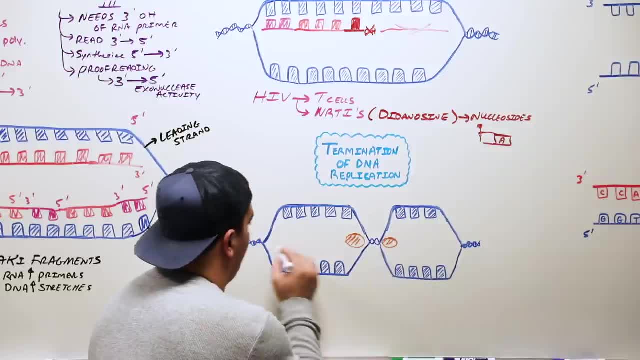 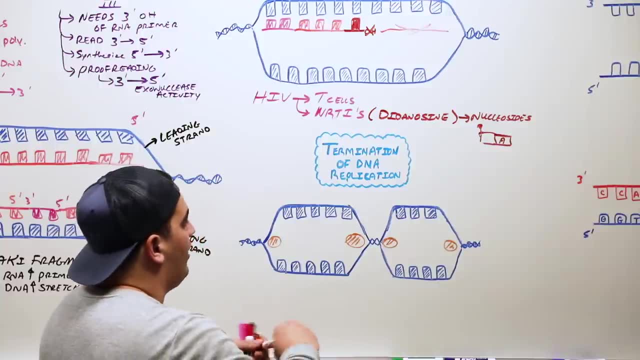 We got that enzyme- What was that enzyme that was working at these replication forks and just continuing to unwind the DNA, you know, in front of it What are they called The helicases. And then you had those enzymes, the DNA polymerases, type three and type one. 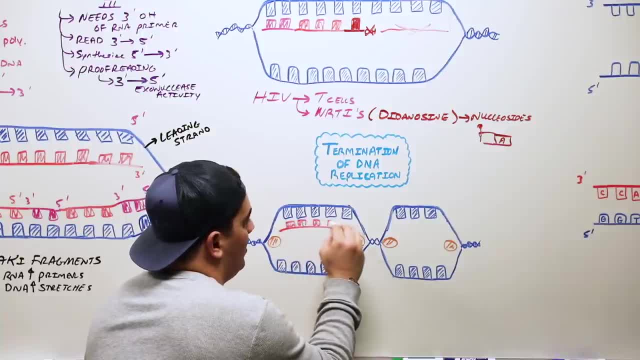 and all those guys that were coming and basically reading the DNA three to five and synthesizing it five to three, proofreading it in the three to five, all that good stuff, And you've synthesized the DNA And the helicases are meeting each other. 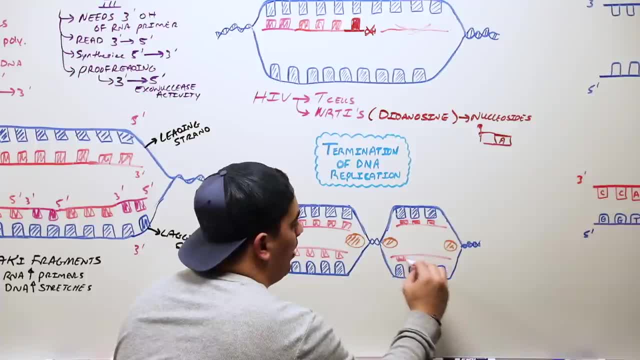 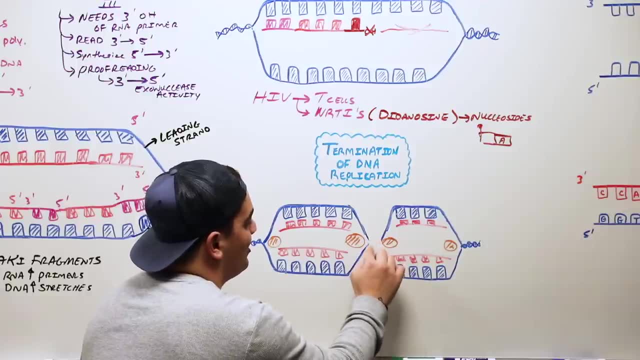 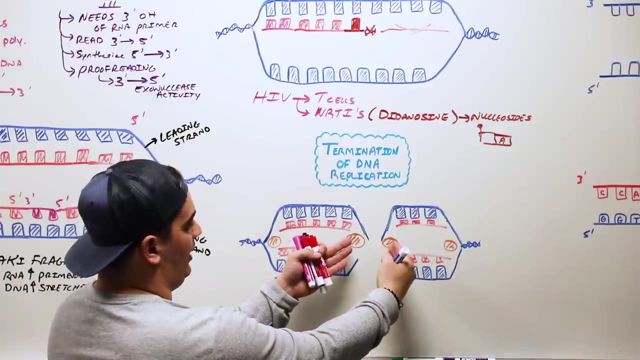 at kind of replication forks that are about to abut one another. When this happens, when the helicases meet and you kind of unwind this portion of the DNA, what's going to happen? The helicases are just going to kind of say: oh well, hey, buddy, I guess I don't need to. 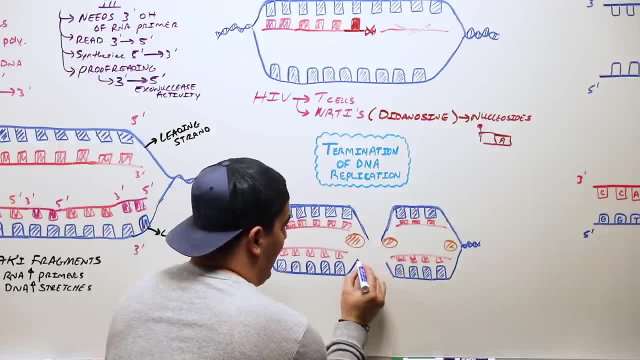 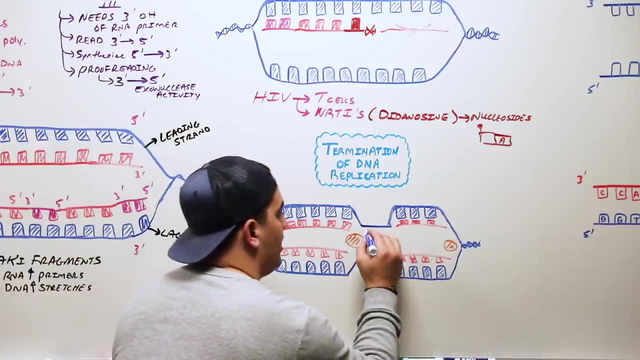 keep unwinding anymore, And what will happen is you're going to have a helicase. that's going to. you're just going to kind of have this point here where the DNA polymerases will just hop off of the DNA Because at this point there's nothing else for it to read, And so usually once it gets to, 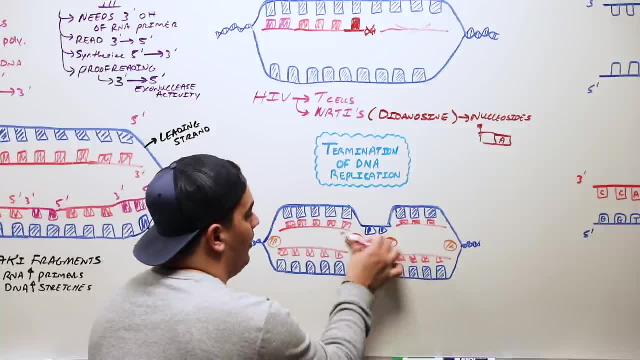 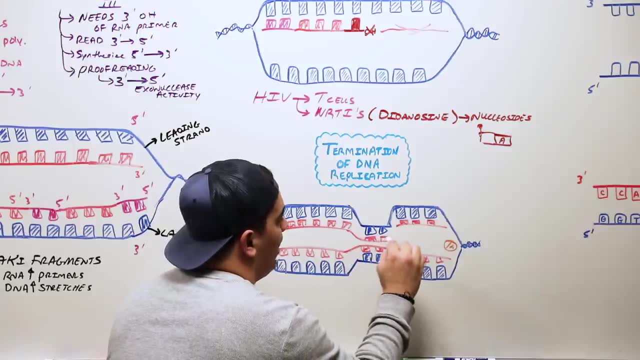 that point they'll just say, hey, I guess the helicases are done, There's no more unwinding for me. And then after that the DNA polymerases will say: hey, I've already kind of hit all the nucleotide regions here, I'm done, And I've replicated all of my DNA, So that's important. 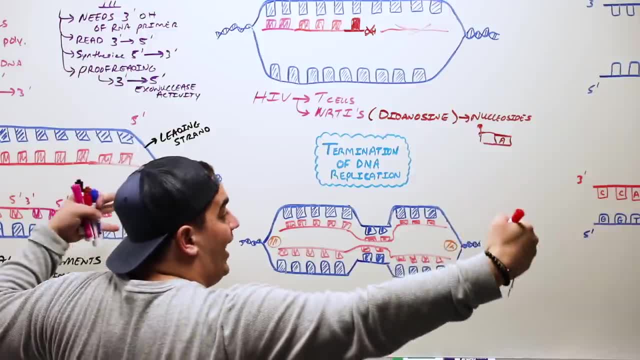 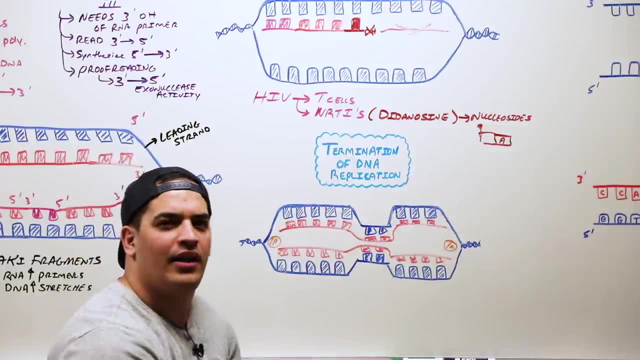 So it's basically again where there's multiple origins of replication and they're constantly moving towards one another. Whenever they moved and hit one another, the DNA replication at that point stops. Now there's something else that you have to remember, though. DNA replication will. 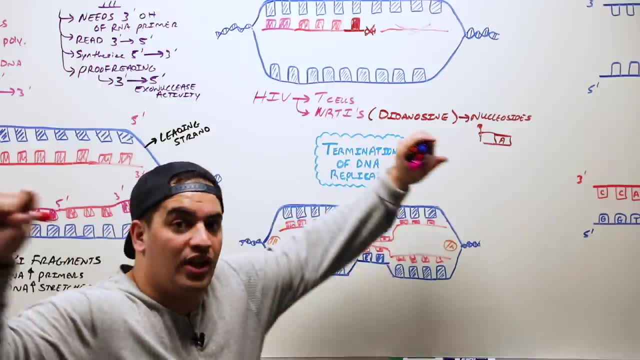 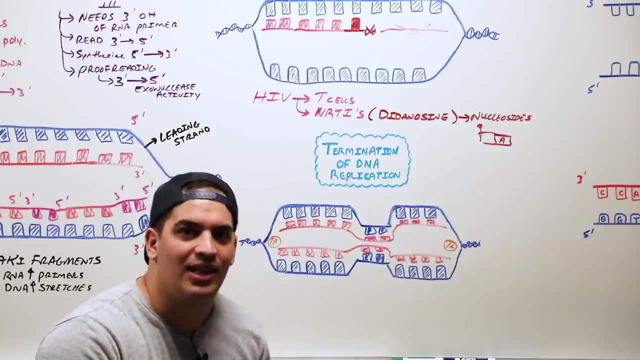 start at a point and then work bidirectionally. It's eventually going to go to the ends of the DNA, or the chromosomes, which we call the telomeres. There's a particular nucleotide sequence at that end where the DNA polymerases have a really hard time being able to replicate. 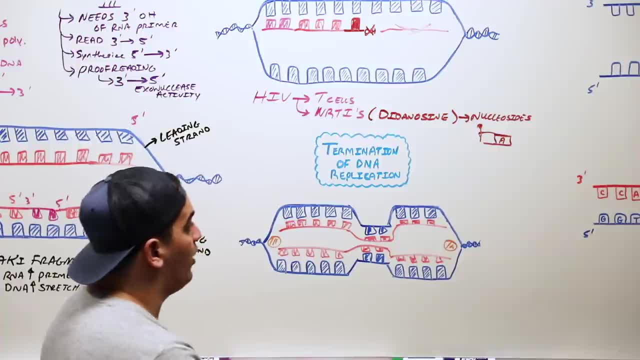 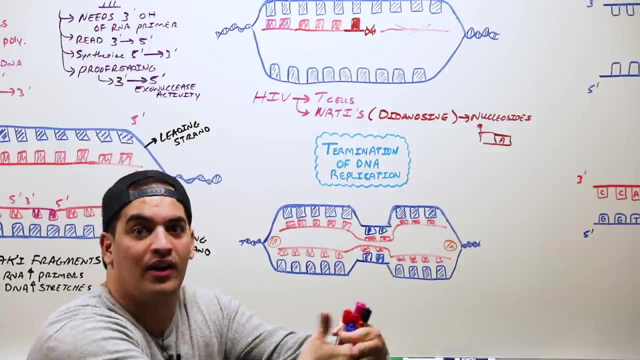 And that's very important. We'll talk about that next, Okay, But again, termination of DNA replication. it's really simple. It's when the DNA polymerases are moving towards one another at a replication fork and they've just stopped at that point, They hop off and they no longer. 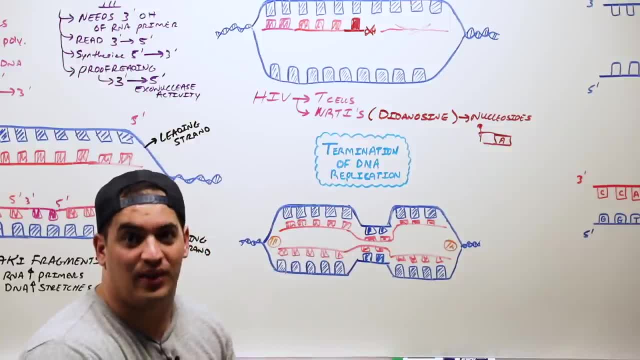 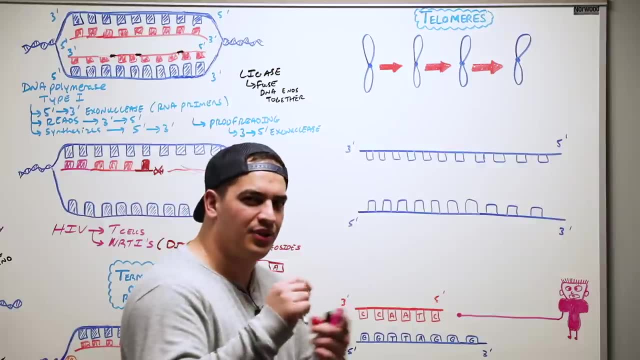 perform their function. There's one other part of it, which is with the telomeres, which we're going to finish off with, All right. So the next thing that we got to talk about is telomeres, right? So DNA replication. there's a little interesting issue that happens at the telomeres. 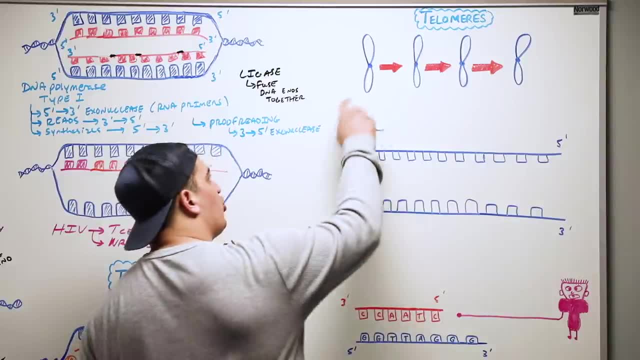 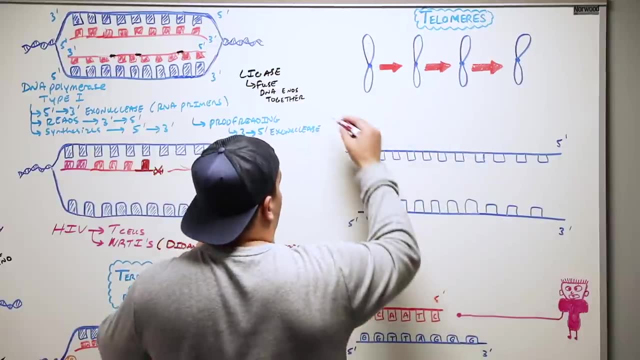 So one thing I need you guys to know is that telomeres they really over time. So let's say that here we look at some chromosomes which are again made up of DNA and proteins. Well, let's primarily think of it as DNA And let's say that this goes through. 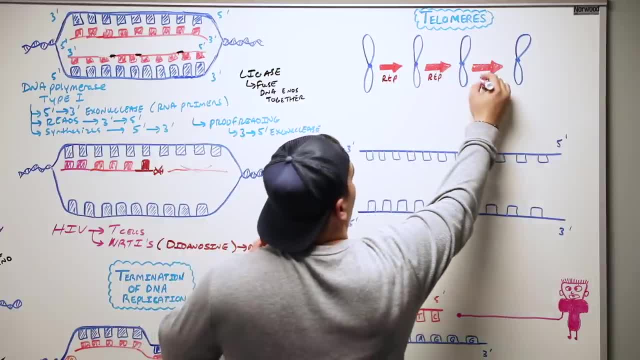 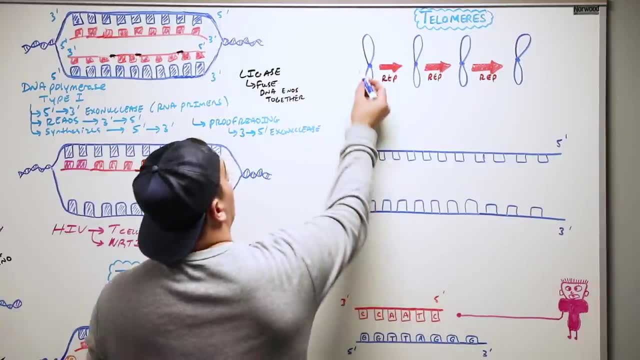 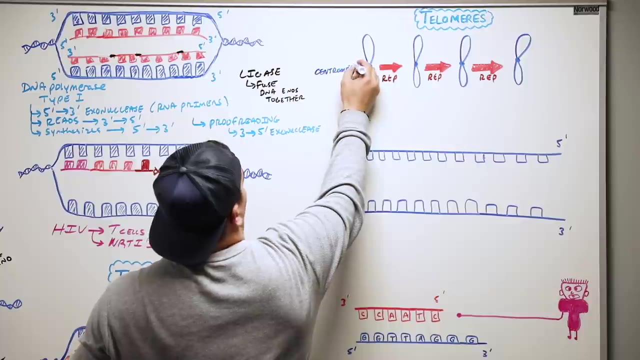 a replication cycle a couple times. I want you to notice what happens to the ends, right. So when you look at a chromosome, there's two primary kind of like structural points: The point in the center right Which is called your centromere, And then the ends. okay, These points here. 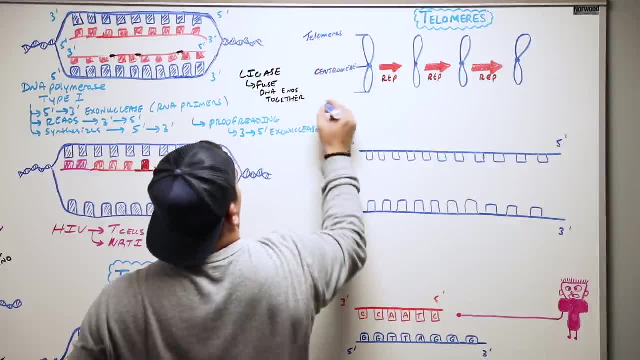 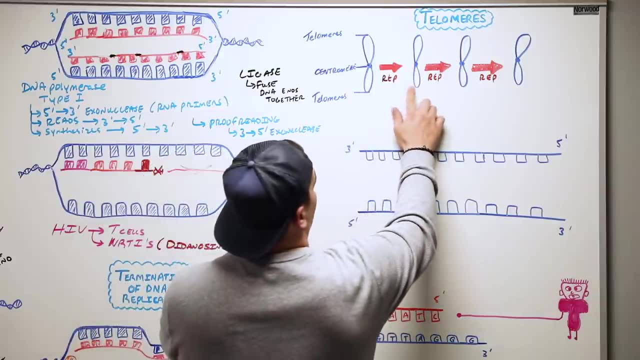 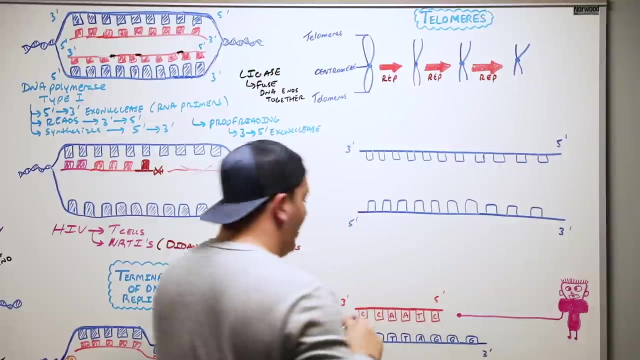 And these are called your telomeres. Now what happens is, over time, as your cells continue to keep replicating and the DNA replicates. watch what happens to the telomeres: They get shorter and shorter and shorter As that continues to happen. there's a worry with this, And let me. 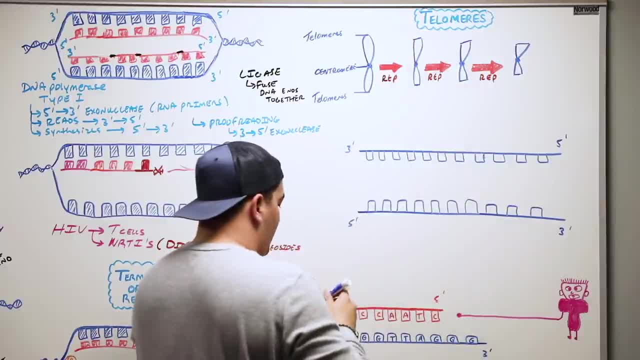 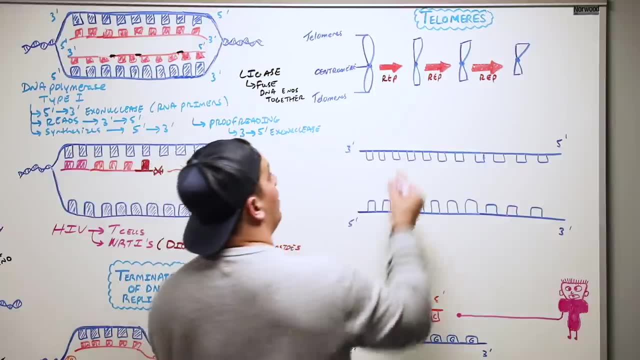 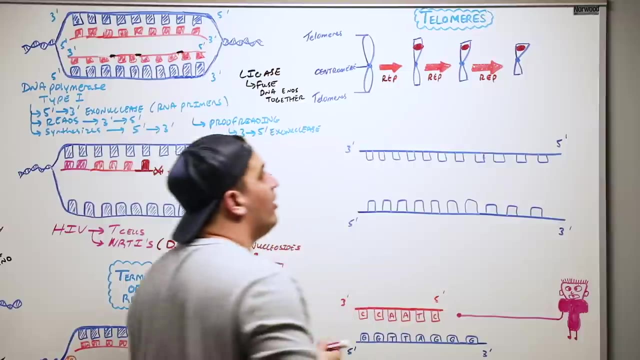 explain what that worry is. Obviously, your DNA has particular areas which code for RNA. RNA can translate into proteins. What are those called? They're called genes. So let's say that I have a gene right here. The telomeres will be there And their primary function is that they will. 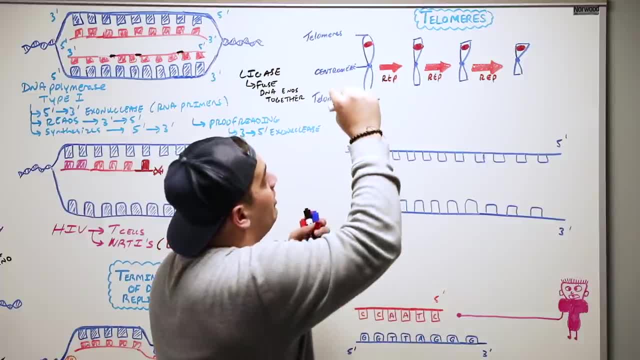 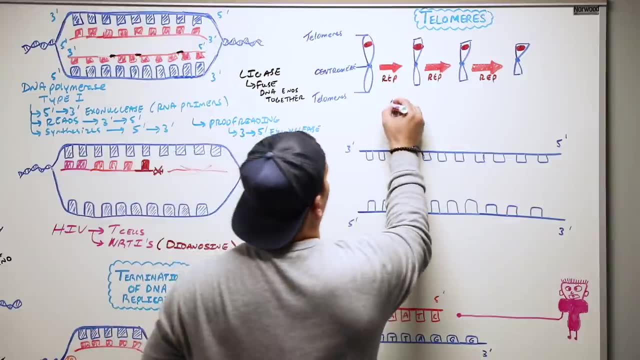 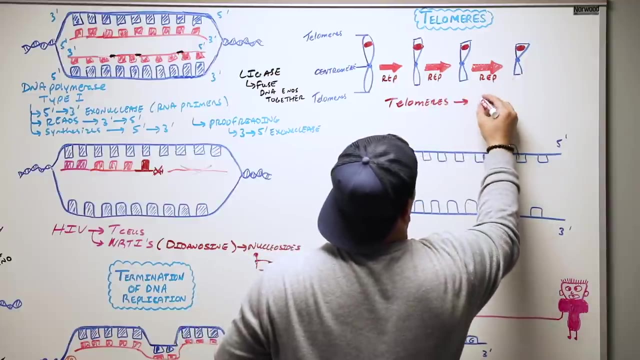 it's common for them this to happen, where the telomeres were shortened and shortened and shortened, But the whole purpose of them is that telomeres don't code for anything. That's very important. Let me write that down: Telomeres do not code for any RNA. 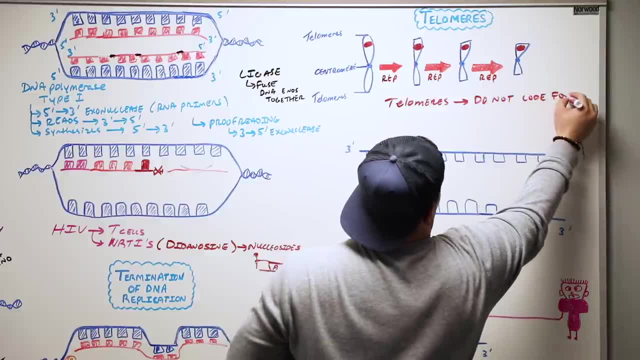 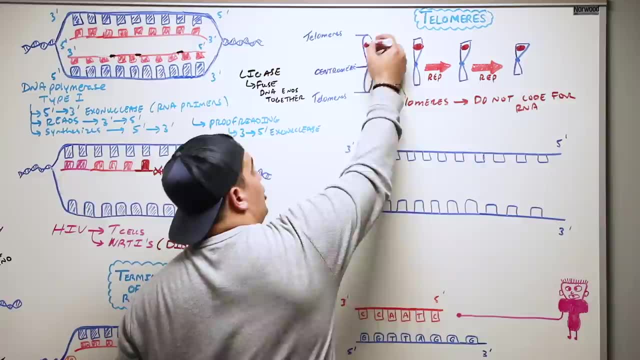 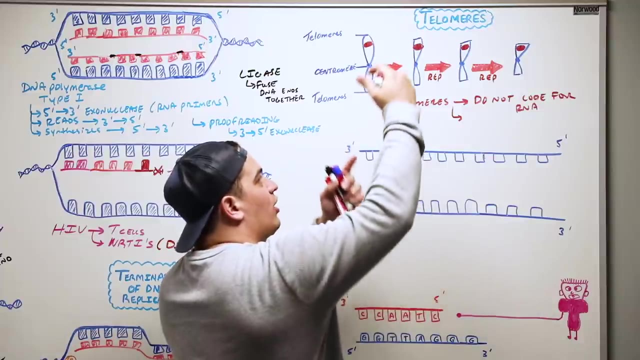 So do not code for RNA. In other words, you can't take the DNA from a telomere, make RNA, make protein. That's important. But let's say here there is a gene there that can make RNA, The telomeres will kind of sacrifice themselves because DNA replication doesn't occur at this. 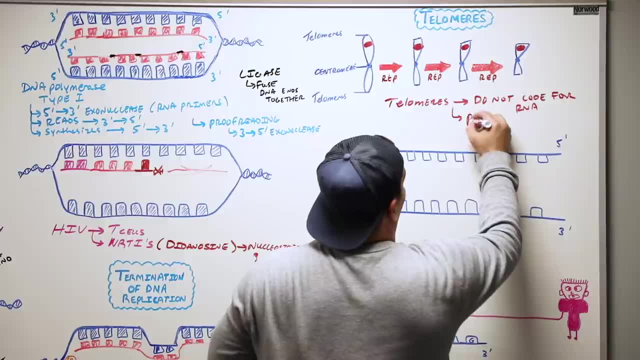 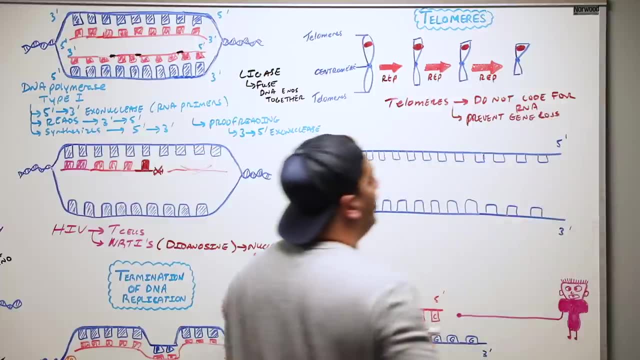 point for a particular reason. We'll explain why. And so because of that they prevent gene loss. So they kind of like take the hit for us. if you think about it, They're like: don't worry, I don't code. 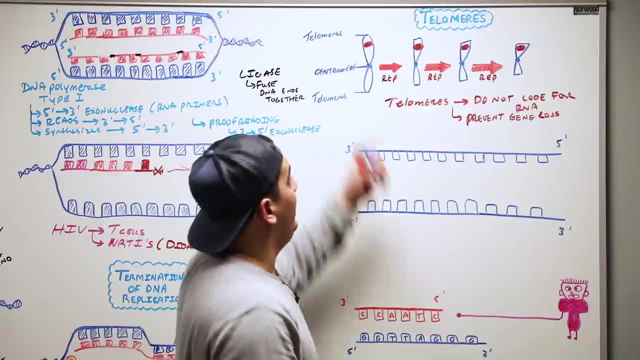 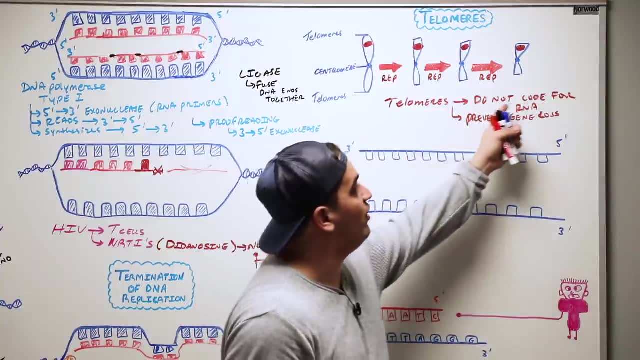 For any RNA, So you don't have to continue to replicate me. So with each replication cycle the telomeres will shorten, and shorten, and shorten. but that's okay, And for a particular reason, because they do not code for RNA and they help to prevent gene loss. But here's the problem. 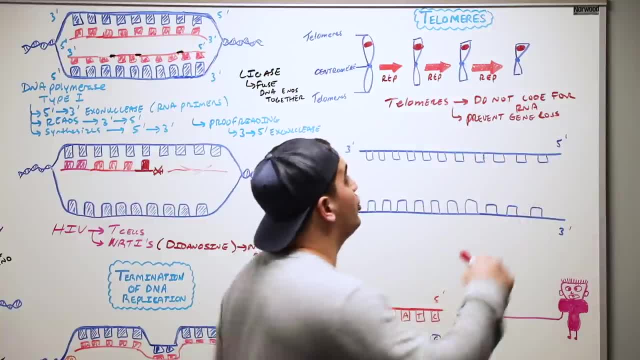 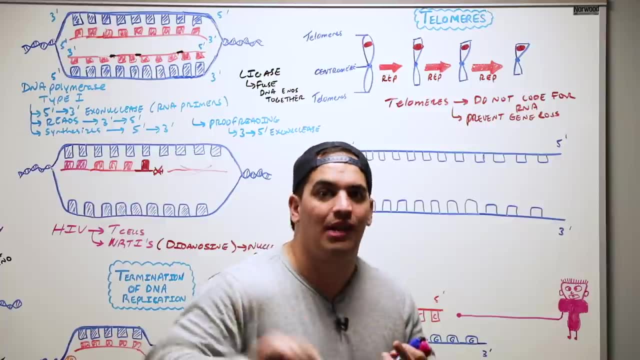 Eventually, you're going to get to a point where the telomeres will shorten so much that it can interfere with the genes. Once that happens, where the cell has reached the replication limit, where it can't replicate anymore, it's reached its maximum number- There's a particular term. 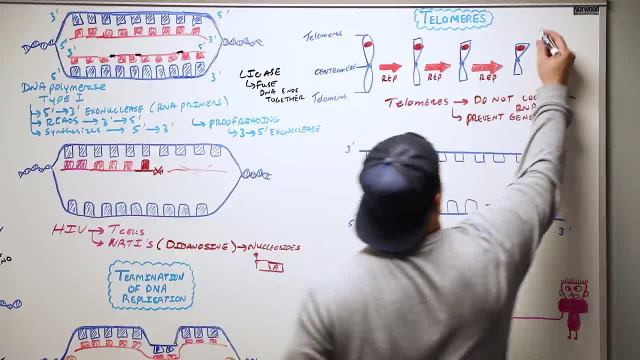 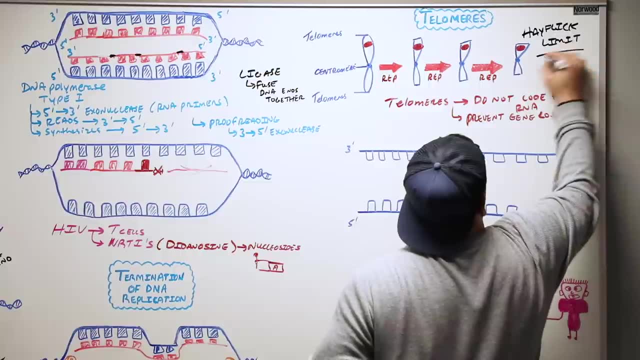 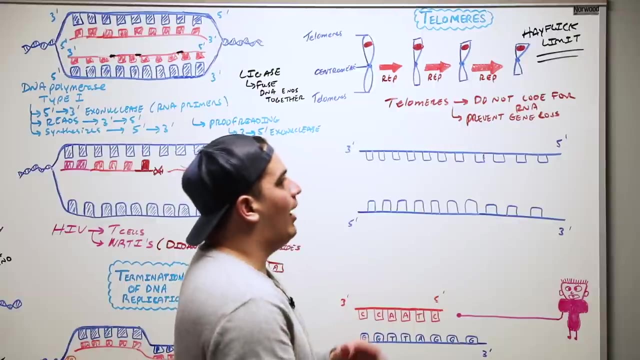 that you guys need to know, and it's called the Hayflick limit. It's called the Hayflick limit, And that is basically the maximum amount of times that this kind of DNA can replicate before it starts to involve genes. Now let's talk about why these telomeres are shortened really quickly. 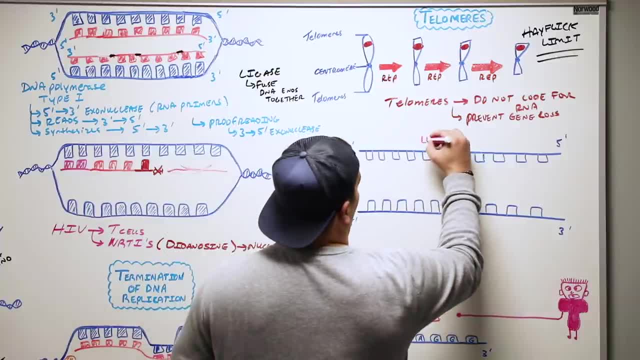 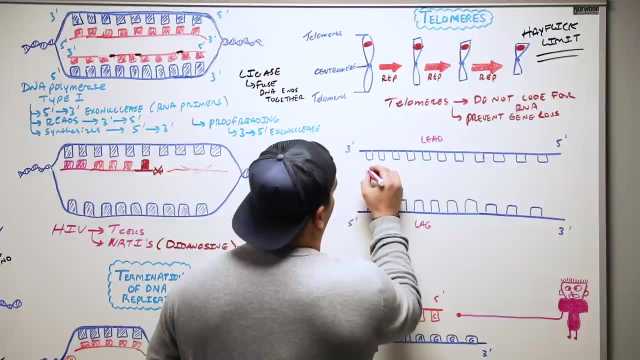 Let's say: here we take in. let's say that we use this as our example. This is our leading strand and this is our lag strand. right, Let's just say: here we have our three prime end. We're going to use our RNA primer here. 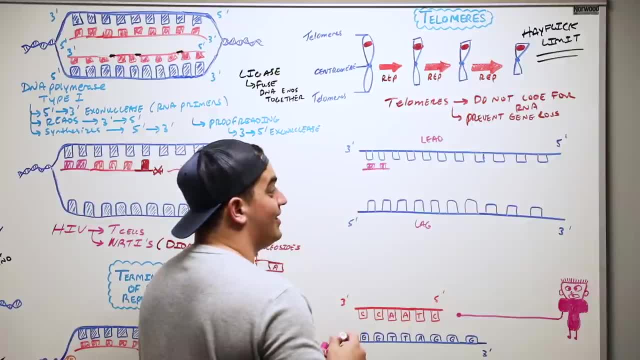 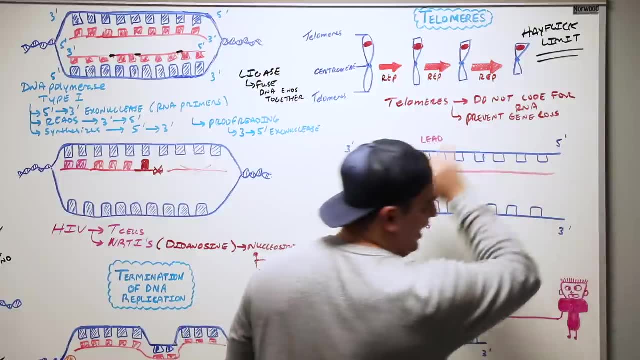 And then from here the RNA primer was made by the what enzyme Primase. DNA polymerase type three will then add on to that three prime end and start making DNA continuously all the way down the leading strand. Remember it was continuous, So this will happen all the way down. 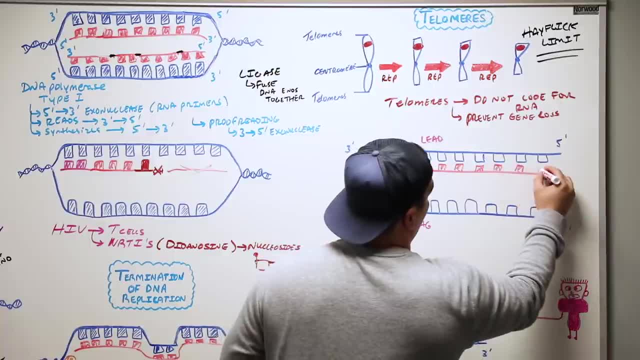 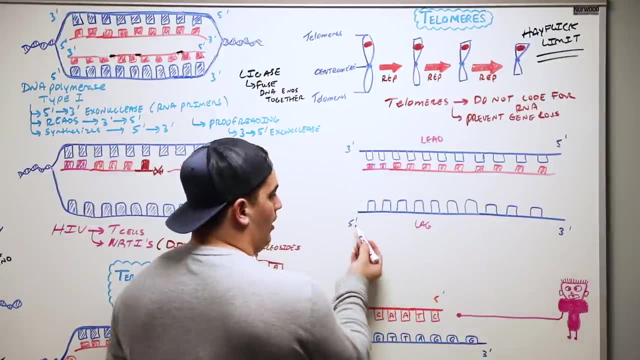 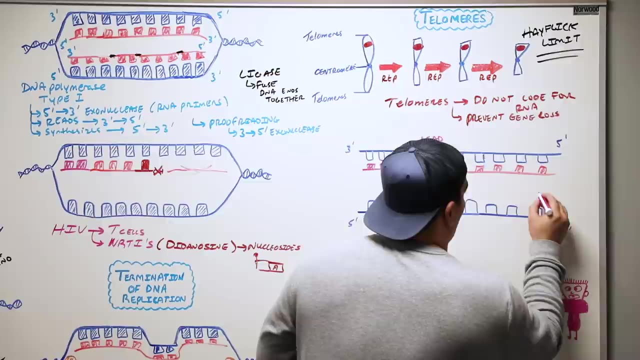 okay, on the leading strand. The lagging strand is where it becomes a problem. So this is our three prime end. right, and the five prime end. The primase will have to add onto that three prime end. So let's say it adds on right here at this three prime end. When it does that, 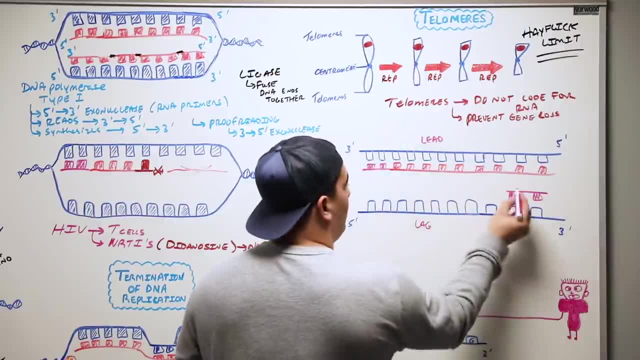 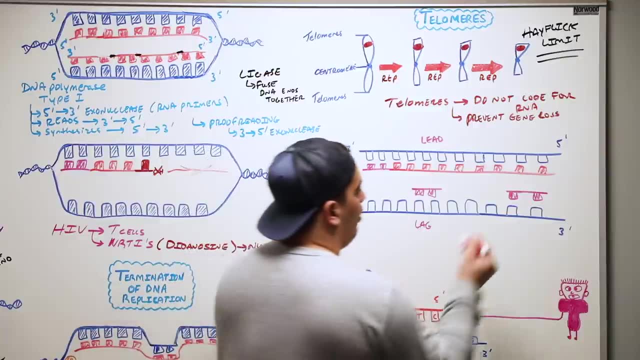 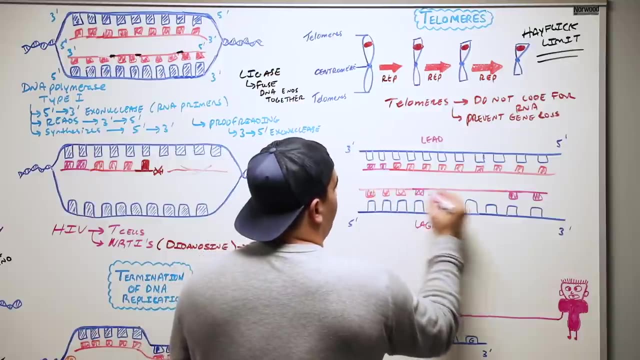 it gives a little primer And then again DNA will build off of that. Here's another primer. and then DNA will be built off of that right. So we kind of know that process. This is pretty much a review of what we just talked about, But here's what's different Here. watch what happens. 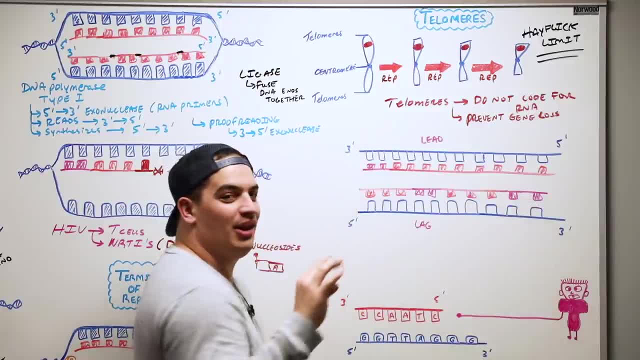 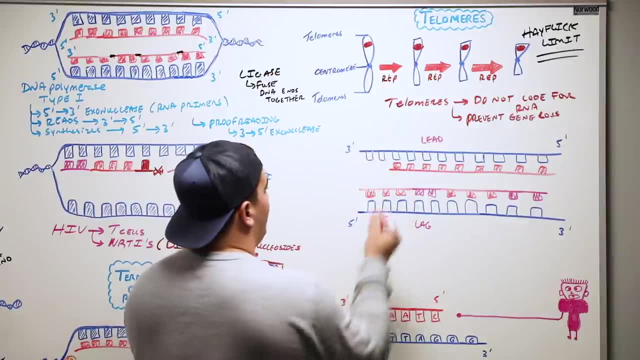 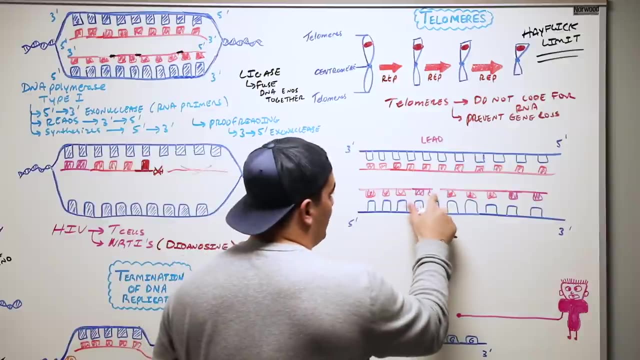 You guys, your minds are about to get blown. Remember DNA polymerase one. What does he come in and do? Comes and plucks off the RNA primer and then makes DNA right on the leading strand, On the lagging strand. it'll come off and pluck this portion here, okay, that RNA primer. And when it? 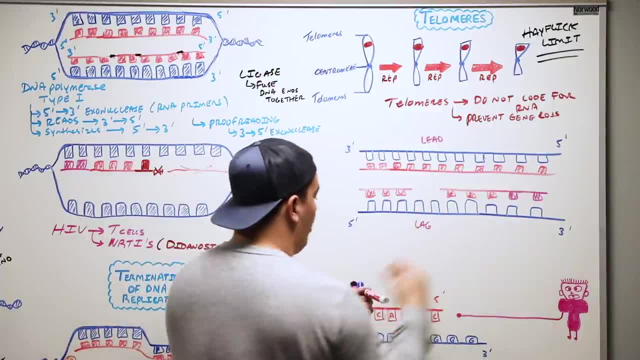 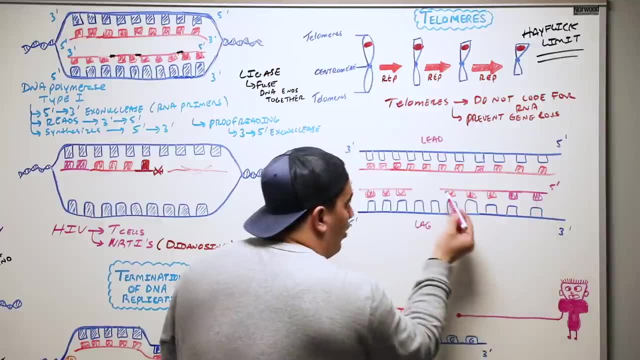 plucks off the RNA primer, it still has a what Remember, this is the three prime end. What would this be here? Five prime, three prime. So remember: five prime, this is a three prime end. right here, It still has a three. 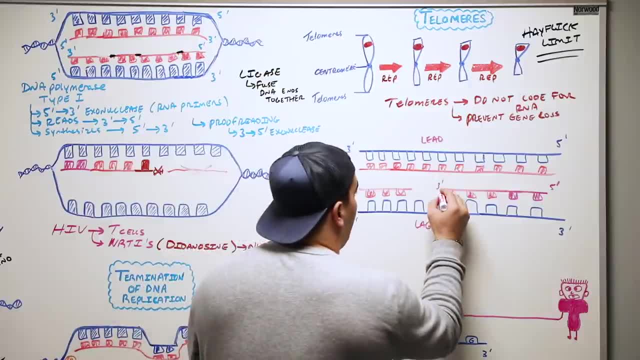 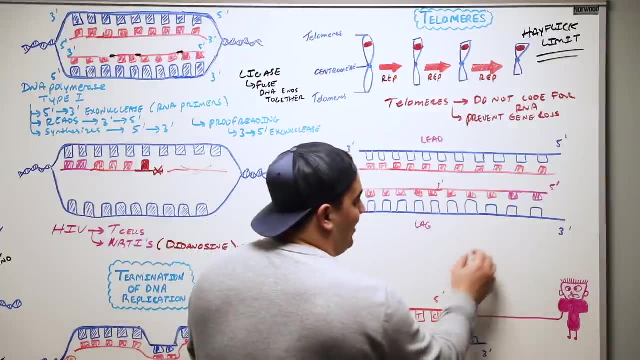 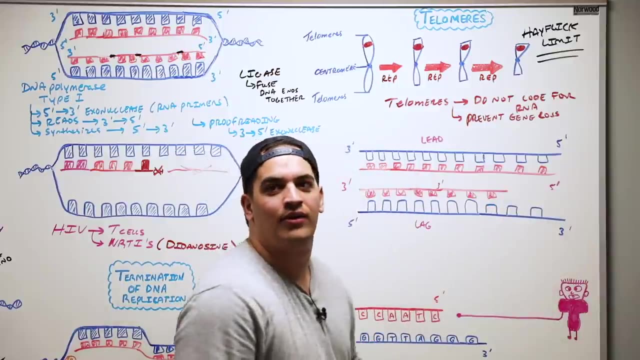 prime end that it can use to build off of and make DNA at this point here. But watch what happens down here, Comes down to this end here, plucks off these RNA primers. Uh-oh, Do I have a three prime end that I can add off of somewhere? I don't dudes Why, Because look. 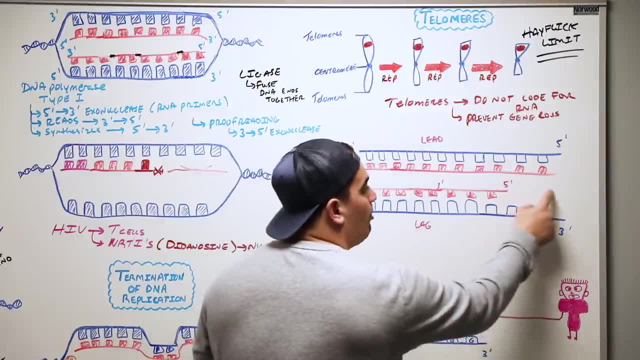 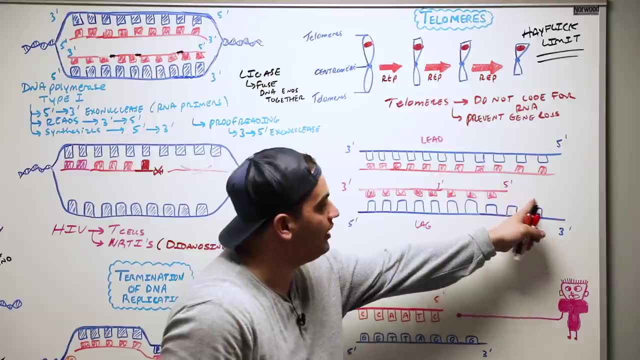 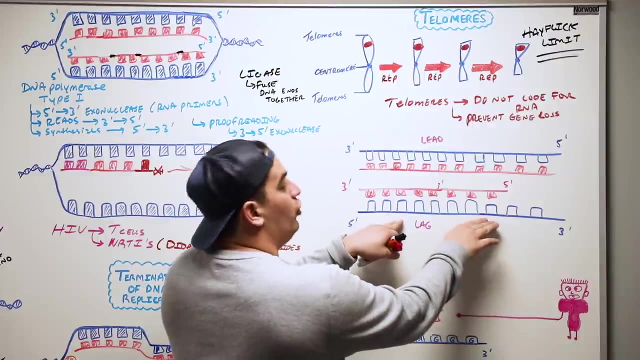 this is my five prime end. I have no three prime end here: that that DNA polymerase can add on nucleotides to. So DNA replication won't occur at these points here. And that is problematic because guess what? This was the old DNA strand. You replicate it and made a new DNA strand- This: one's going to get shorter. It's shorter than the original one. Guess what happened? when this one replicates, It'll get the. the new strain will be shorter than it, And then the next one, next one, and the DNA will continue to get shorter and shorter and shorter and eventually start. 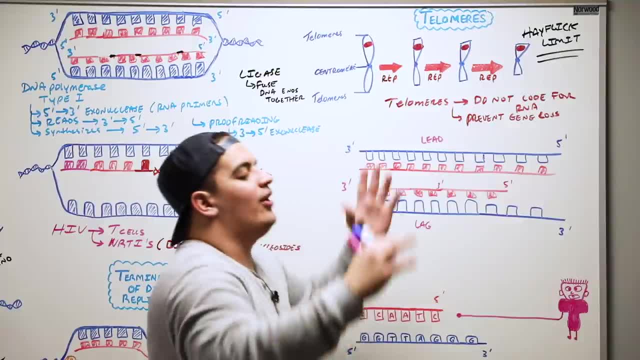 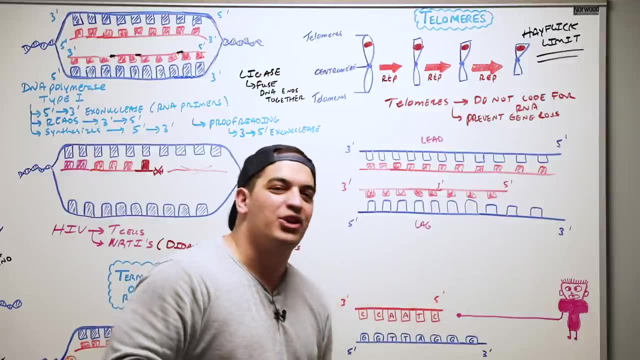 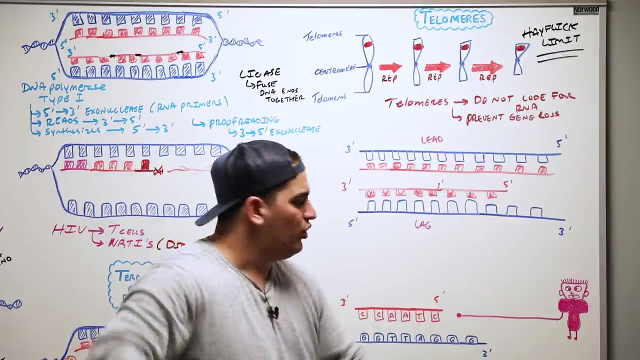 involving those genes. so, thank goodness, in particular cells where we have a need, a lot of replication to occur, we have a special enzyme that comes in and says, hey, I'm going to elongate those telomeres for you, so that way, whenever DNA replication does occur, you don't start really. 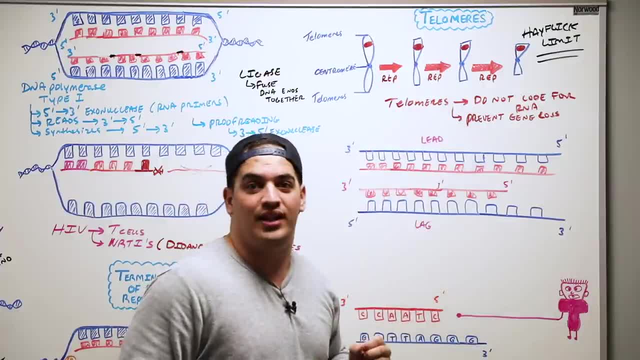 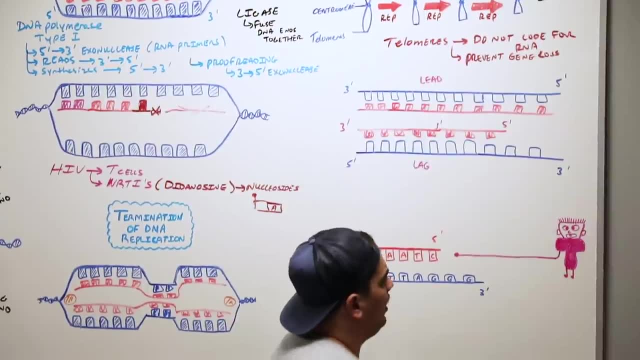 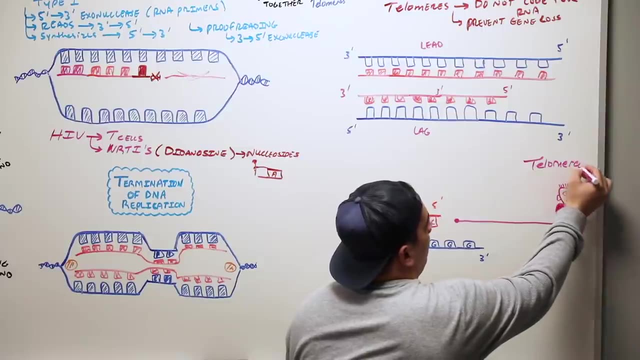 taking away too much of the telomeres and involving these really important genes. so what is the name of this special enzyme that we should give great thanks to? this wonky looking enzyme here has two arms, and this enzyme is called telomerase, and telomerase is a really interesting kind of 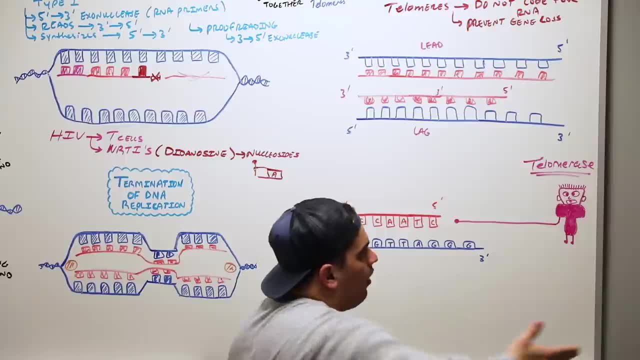 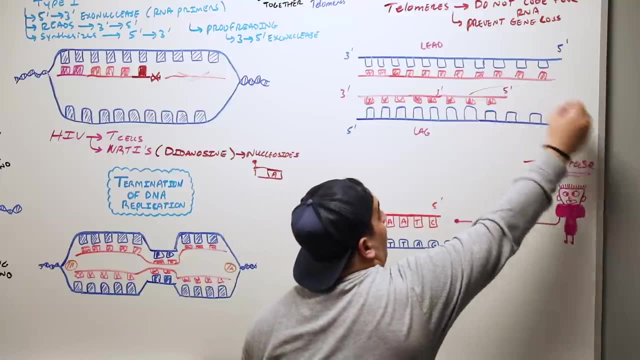 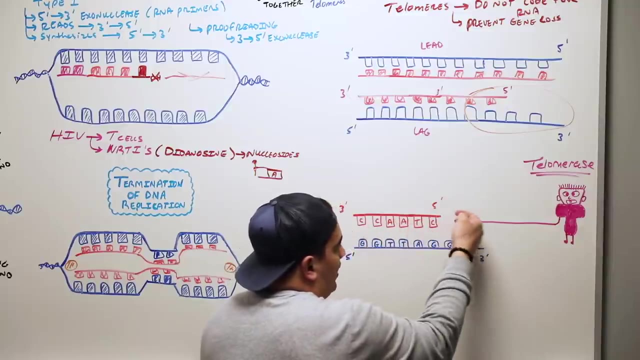 ribonucleoprotein. one arm comes here, okay. so, remember, we're just looking at this portion here, so we're only zooming in on this lagging strand about right here, okay, and zooming in on it. so here we're on this portion where we didn't finish and synthesize the nucleotides, because 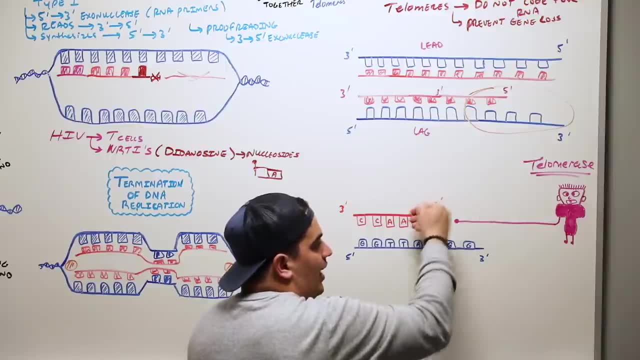 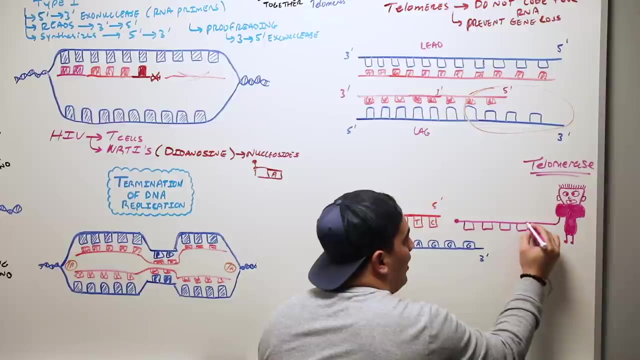 again, we didn't have that three prime OH region here to add nucleotides off of for the DNA polymerase. so what the telomerase does is it takes one arm and brings that arm out, and on this arm is something really, really cool. it expresses nucleotides and a particular type of nucleotides. 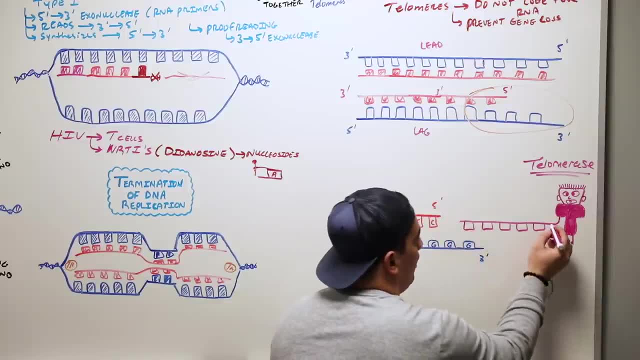 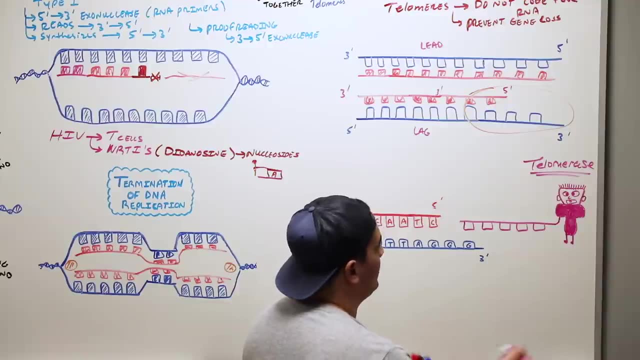 that you guys really need to know. okay, and so what are these nucleotides that it has? well, what it expresses is complementary nucleotides that are commonly seen on the telomeres. telomeres always have- and the easiest way there's a mnemonic to remember them. telomeres always have a particular repeat of nucleotides on them, on their 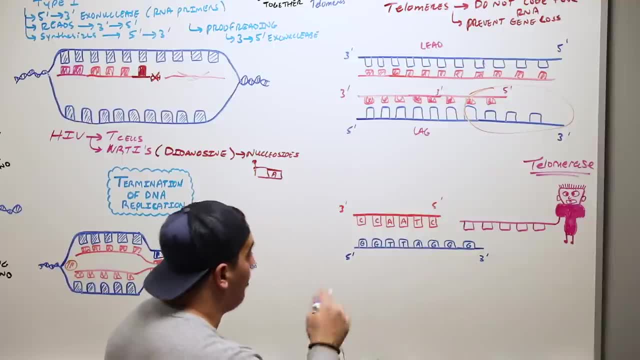 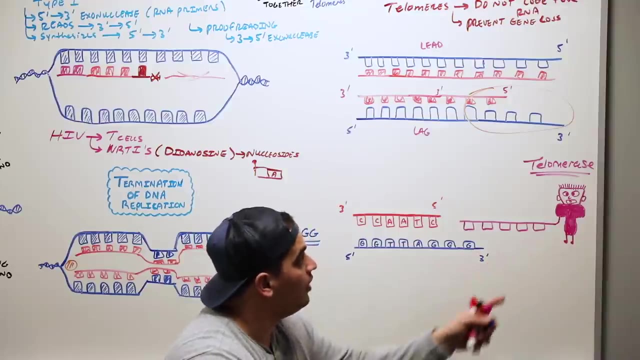 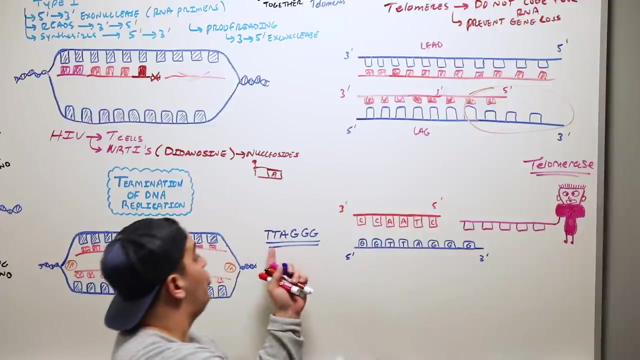 three prime end. and the easy way you can remember that repeat is the mnemonic: tell them: all genes gotta go. that is the repeat that you constantly see on that three prime end of that parental DNA. so what telomeres does is it comes in and says, hey, I have all the complementary RNA nucleotides to this. 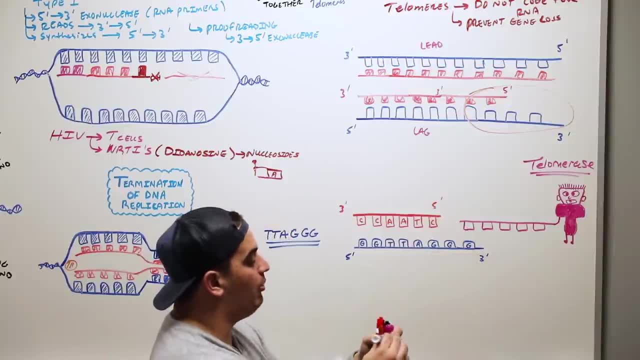 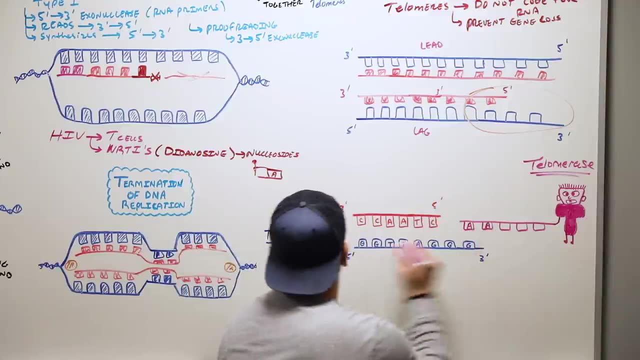 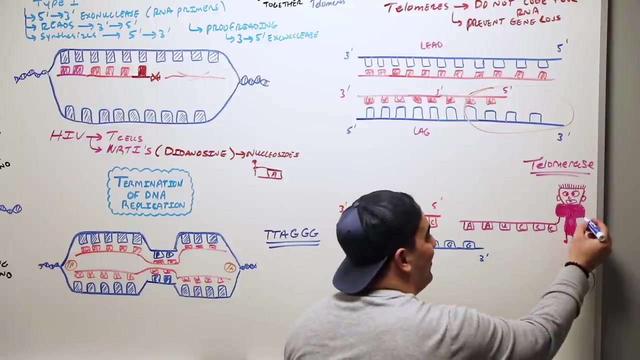 sequence that's commonly seen here. so let's kind of write down what would the complementary portion be. if it was T, it would be A, T, it would be A, A, it would be U, G- all the way over here, so you got a across- it would be C, C, C. So it expresses that with its one arm, The other arm is really cool. 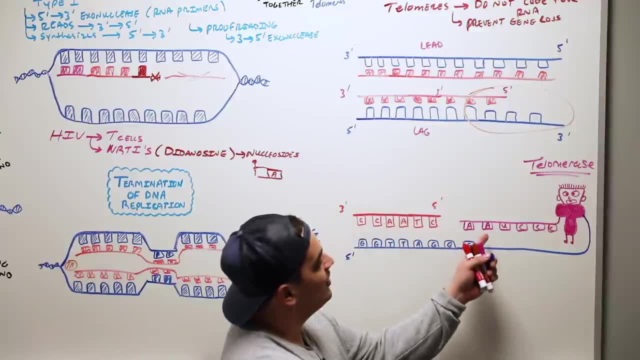 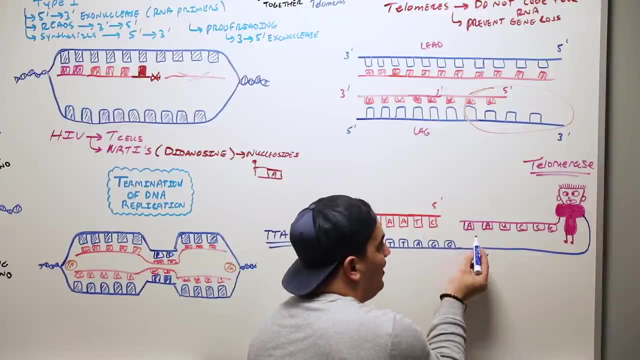 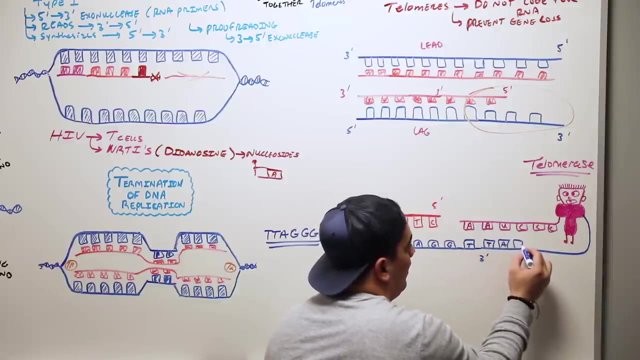 The other arm will then use this RNA strand as a template to make DNA that's complementary to it. So if it does that, it's going to take this RNA, read it and then what would be the complementary? T, T, A, G, G, G. 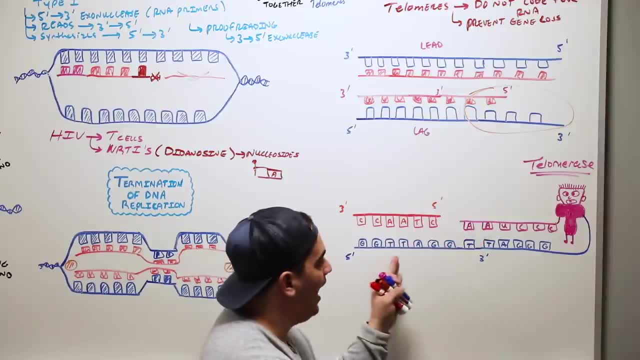 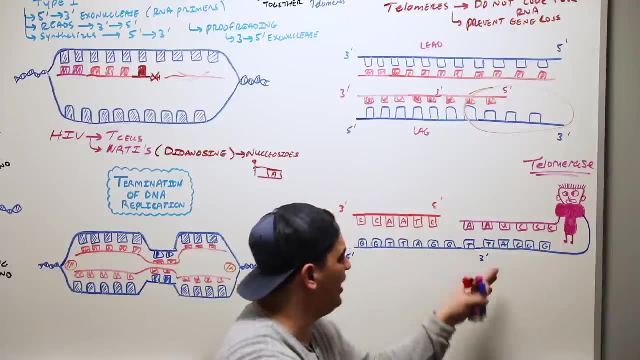 This is really interesting. You want to know why I elongated my 3'N. okay, which is important. I elongated it so that way next time this DNA replicates I won't really take too much of the DNA and involve those genes because of the telomerase. 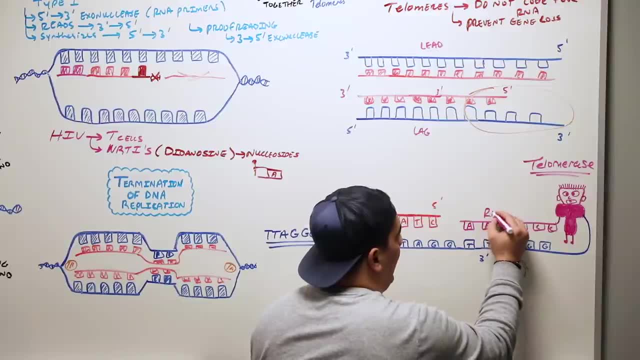 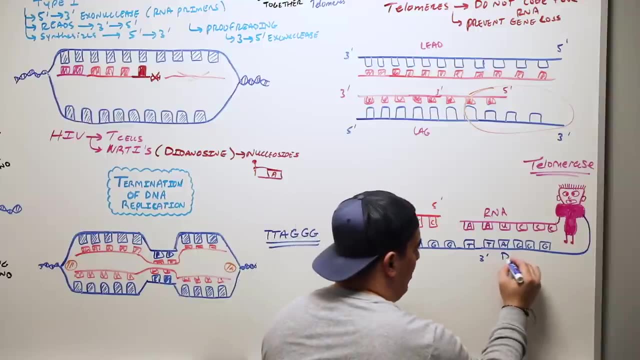 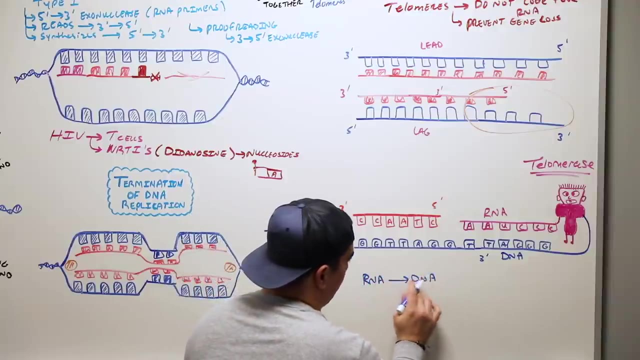 But what I did is I used RNA And from that I used T And I made DNA. I need you guys to understand what that's called. What is that called when you go from RNA to DNA Reverse transcription? This is called reverse transcription. 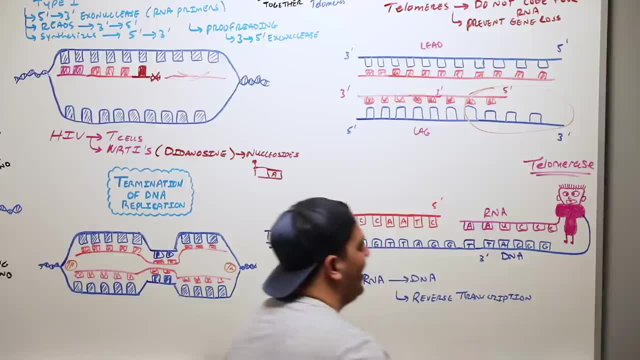 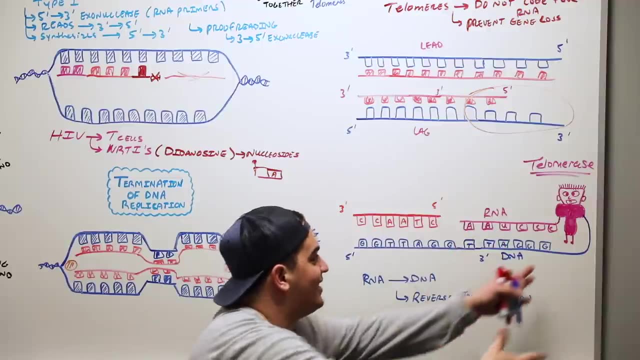 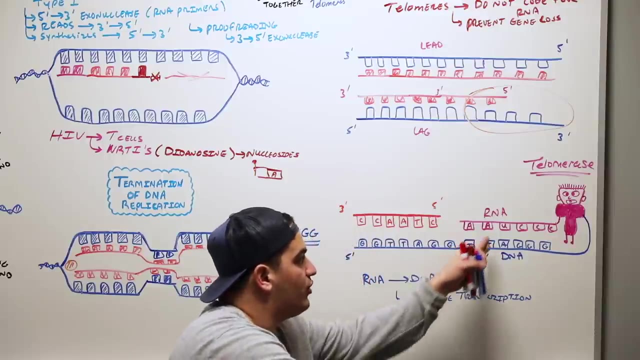 And so what this kind of telomerase does in a way, is it has again. it's a protein which expresses nucleotides, It expresses RNA, And then it has this: It has this other arm, this other arm that reads the RNA, and says: oh okay, this is A, I'm going to make T on the parental strand. 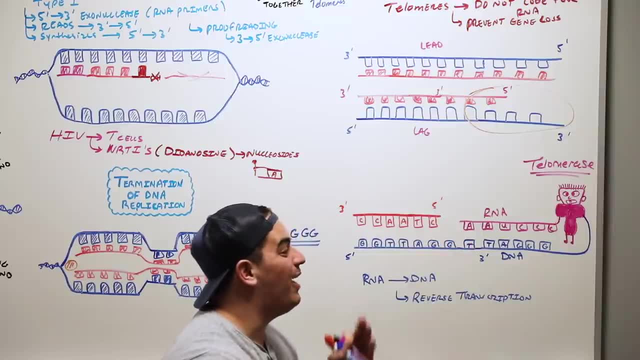 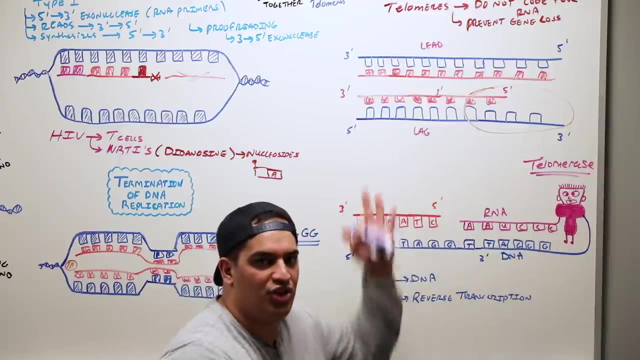 That's A. I'm going to make T on the parental strand So it can take RNA and make DNA elongating the telomeres. Why would we want to elongate the telomeres? We obviously know to prevent gene loss, and so we don't shorten those telomeres significantly. 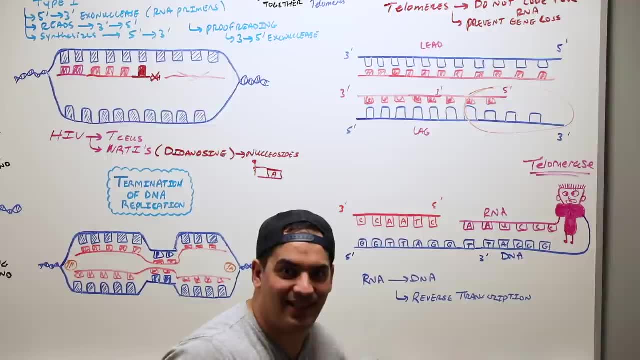 And what cells would you want there to be? a lot of telomerase enzymes or a lot of high activity highly replicating cells, Cells that are replicating so much That those telomeres would shorten if we didn't have it. So this is important. 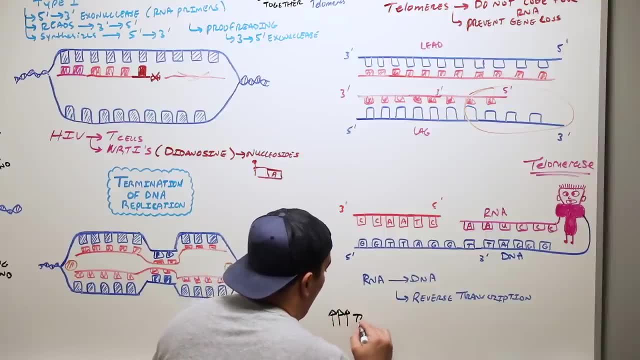 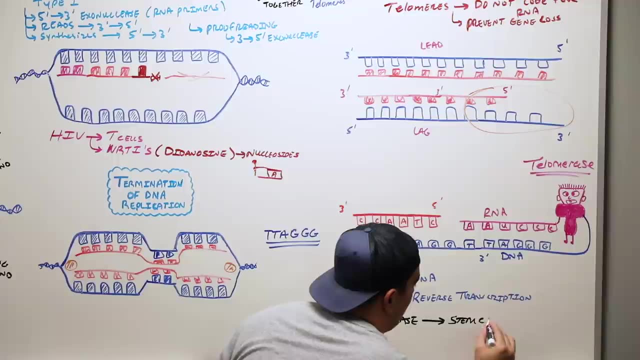 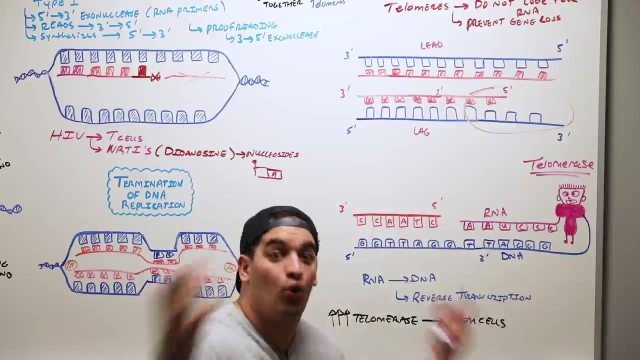 You need lots of telomerase enzyme. And what kind of cells? Primarily in like stem cells. So if you're a zygote and you're starting with one cell, you need those cells that have lots of telomerase activity to replicate and make the whole human body. 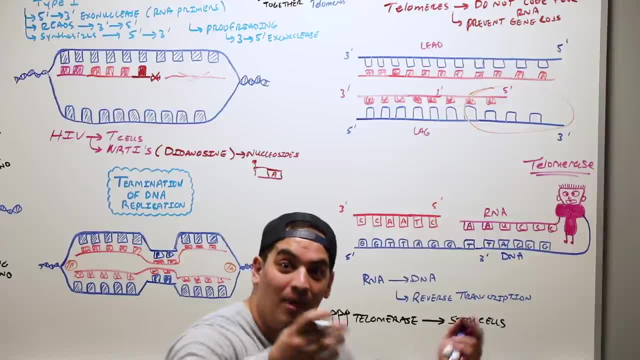 Or your hematopoietic stem cells which are making red blood cells, white blood cells, All those different things. You need those to be able to replicate and have enough telomerase enzyme so that it can replicate without hitting and losing those genes. 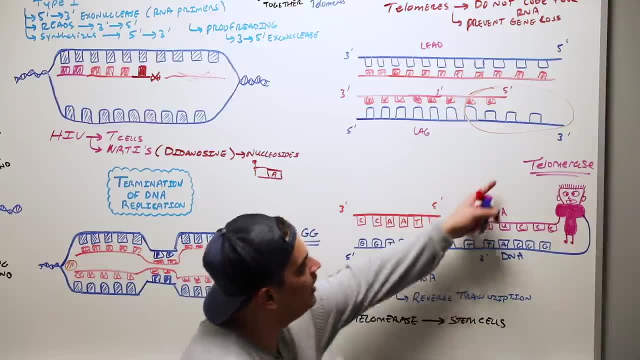 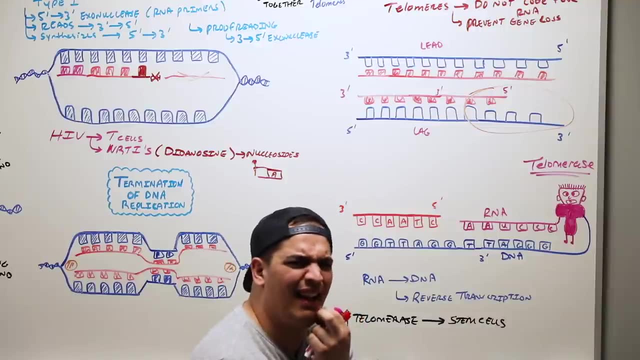 That's important. One last thing: Clinical point: Telomerase. What if we figured out a way- Cells- Certain damaging and really nasty cells- figure out a way to evade the cell replication where they can just continue to keep replicating without not being able to stop?